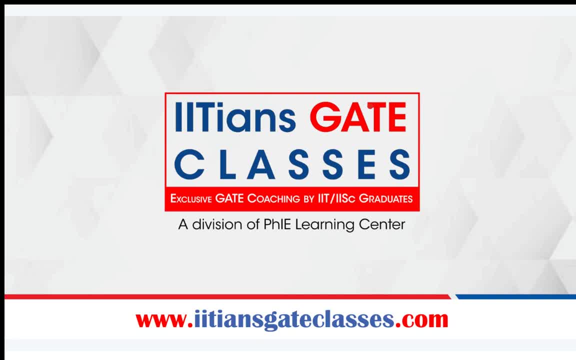 So, So, So, So, So, So, So, very quickly, in our last class we have discussed some fluid properties, So, So, So that we will continue, So, So that we will continue. So we have to discuss about the viscosity. 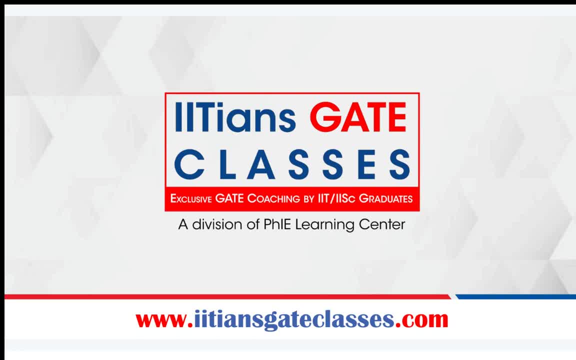 Right, Yes, Yeah, we will talk about it, So yeah. so some of you guys are having doubts, right, In particularly what you call point function. that is clear, right. Point function concept was clear, right, Like point function, right. 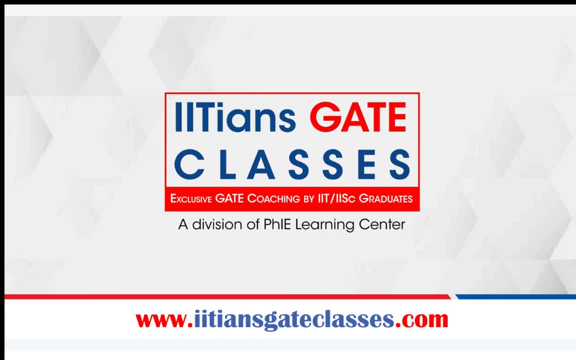 So yeah, All the properties are point function. whether it is what you call intrinsic or extrinsic, all the properties are point functions. It does not depend on the path, it only depends on the end points, getting a point In thermodynamics also, or in gas dynamics also. you will come to know about that thing. 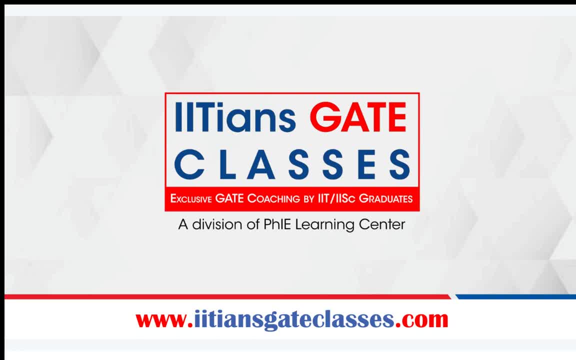 And can you please quickly tell me some of the properties: intrinsic or intensive property, Internal energy right. If I talk about, If I speak, internal energy, that will become intensive property right? That will depend on the end points, right. 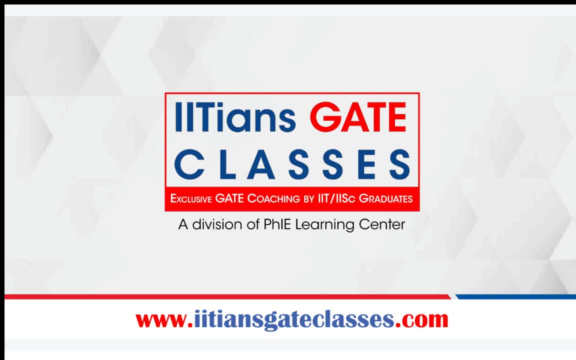 For more clear informations, let me give you a very quick idea about PV diagram. So how many of you are aware of this diagram? PV diagram in thermodynamics. And what about area under the curve of PV diagram? If I draw any curve A to B, then what it will give me. 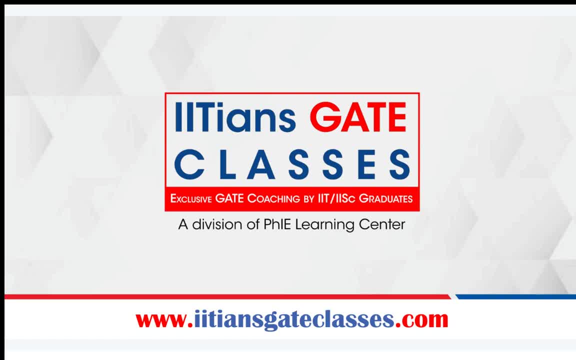 So let us see, Okay, What actually other end points do it beautifully. These are quite simple lines. Just say: w Beta R delta is equal to greater than W of theta delta slash two times w beta x, In other words. please, dear viewers, thank you for viewing this video. 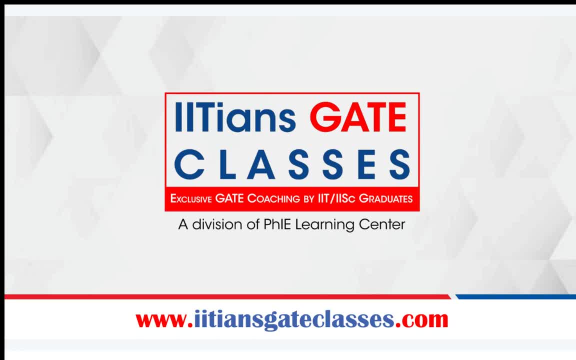 See you in the next one. Bye for now, Not visible, Just wait, just wait Now, if you can just see that. See, This is tear часто. expressions over there you can say they don't change thehews of. 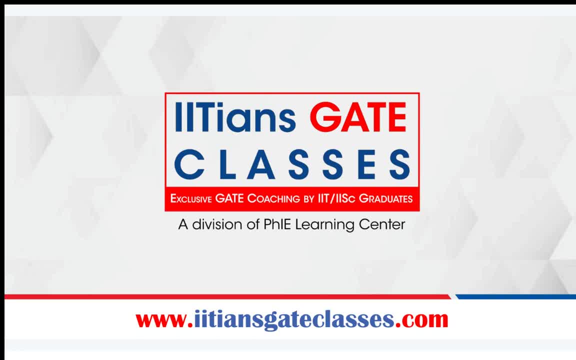 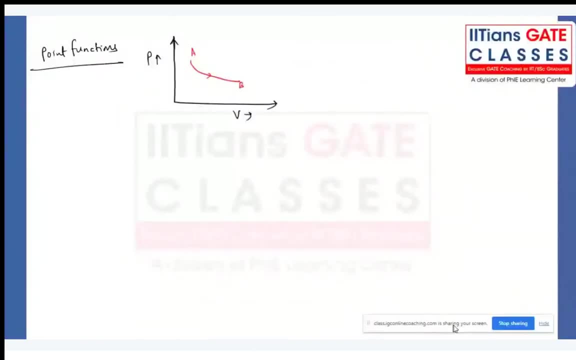 vacuum also of actually Falcon's measuring power. So let me See, So let me just write it down Here, I am… How muchョ can I pull? Okay, So I have just drawn the PV diagram. if we just look at very carefully this PV diagram, 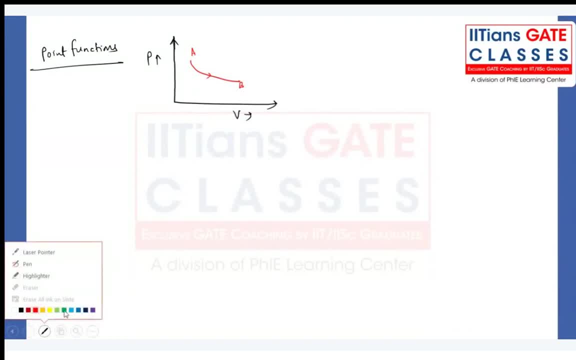 the area under this curve will give me work done, work done by the system. Now, if I draw another process, this is A to B, let us say this is a path 1, and let us say this is a path 2, or may be A to B, and then B to A, or this will be the cycle. let 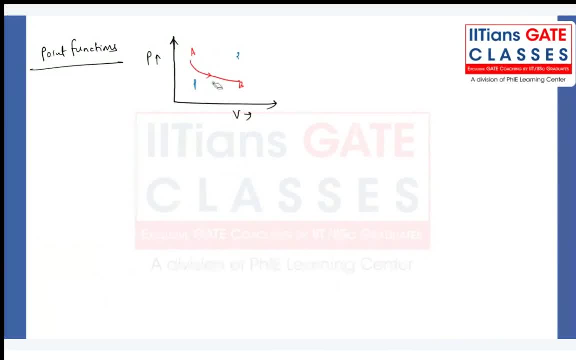 us suppose, for example, now this blue color, what you are observing, the red color, this is the path number 1, and the blue color, this is the path number 2.. So when we talk about the work done, the work done in path number 1 will not be equal. 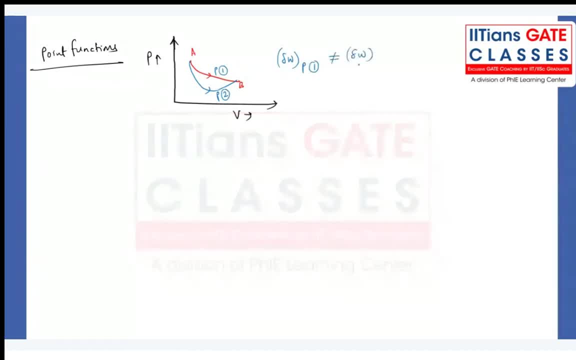 to work done in path number 2, getting my point. So work done is depending on the: what Path, that is not the point. function, that is not the property. But if we talk about the internal energy, internal energy for the path number 1, that 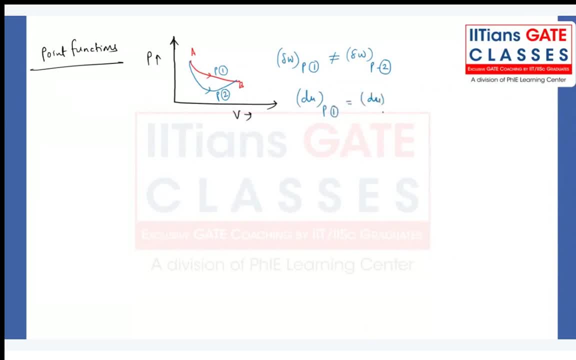 will be equal to whatever the changes in the internal energy for the path. number 2 will be same, Because internal energy will depend on the end points. What is that? U, B minus V, A and end points for both? the path is what same. getting my point? tell me, guys. 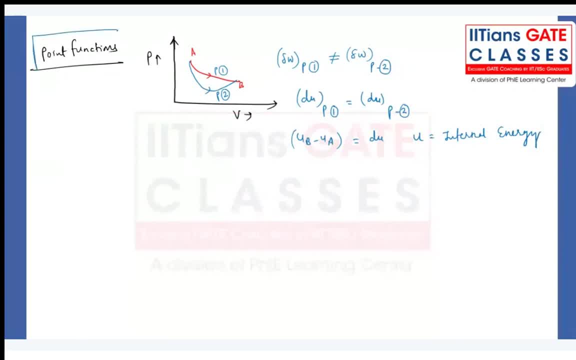 So just please make a note of it Once again, in thermodynamics it will be very much clear about this, all this topic, But for the time being, if you just make a note of it, that would be a good idea. And one more thing: we talked about the characteristic length. 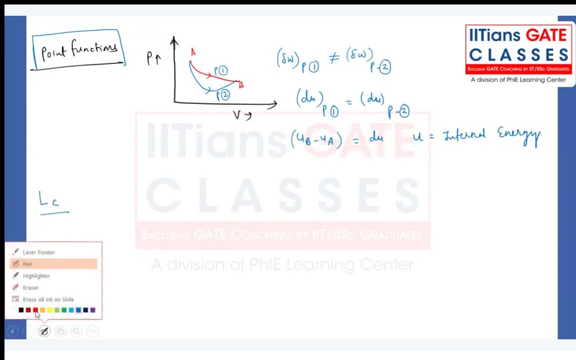 So some of the student, like one student, messaged me on WhatsApp regarding characteristic length. This characteristic length basically talked about the which affecting the type of flow, which affecting the type of flow for a particular fluid. Now, so what I said, the characteristic length, which basically the parameter which affecting 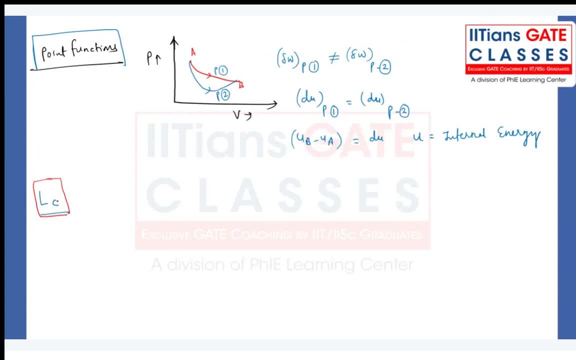 the types of flow. right Types of flow means laminar flow, turbulent flow, transition flow right Now, So in the particularly internal flows, internal flows like a pipe flow, right In the particularly pipe flow, what we have talked about. whenever fluid is flowing, then 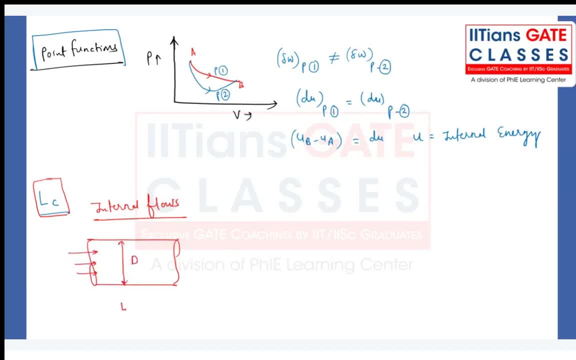 whatever the diameter will be there, the diameter will play a very vital role, right, The diameter will play a very vital role right In deciding whether flow is laminar or turbulent. right, Because what is the Reynolds number? Reynolds number is basically rho V, D by mu. 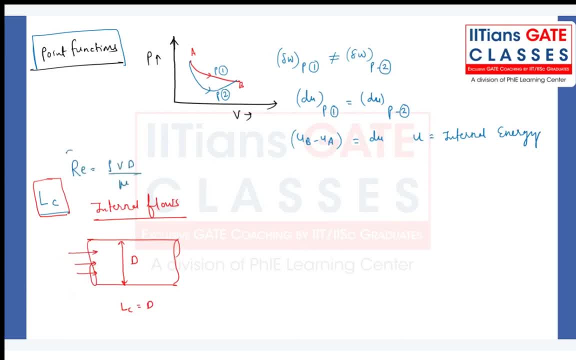 Right, Okay, So what is the Reynolds number? Reynolds number is basically rho V D by mu. Basically, if you talked about the Reynolds number, we used to write rho into V, average characteristic length divided by mu. That is about the internal flows. 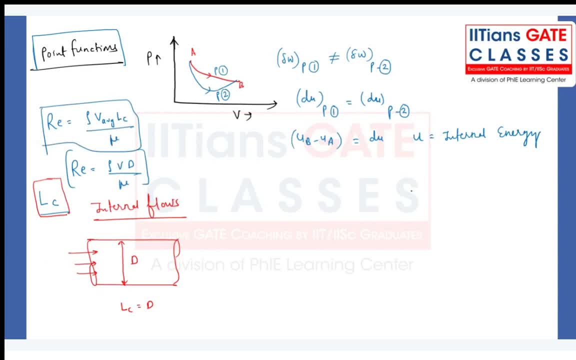 That is about the internal flows. What about the external flow? What about the external flow being over the flat plate? If the flow is happening over the flat plate, my dear friend, which is having a length L and width W, here, what you will be observed that characteristic length will be L Because length. 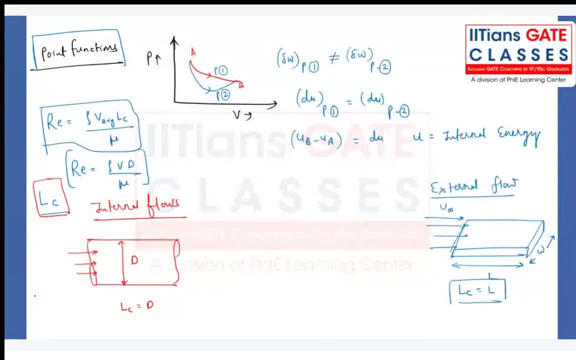 will be deciding parameter, not the width. If the flow will be happening along the width direction, then width will be important for us Getting my point. So that is the external flow. One more case is there in the external flow: No. 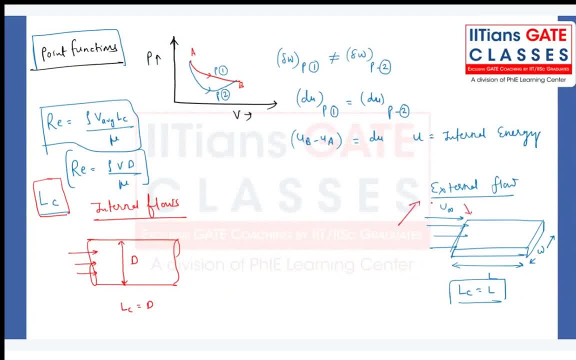 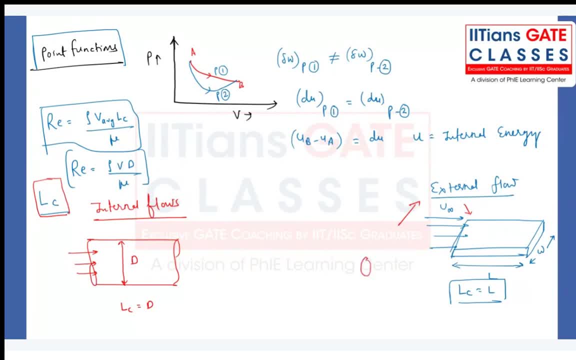 about all the cases. The flow over the cylinder, right, If the flow is happening over the cylinder. or I can say like this: if the flow is happening over the cylinder, then what you can write? What about the characteristic length? Not the length of the cylinder. 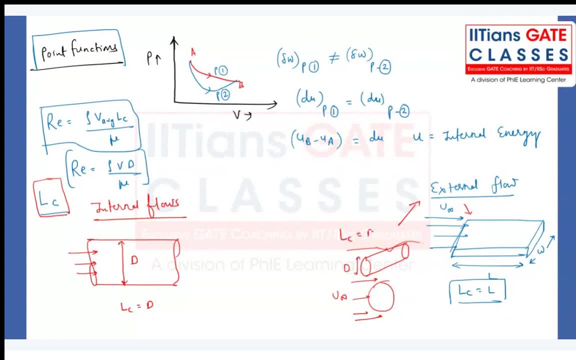 The diameter of the cylinder once again will be important for us Getting my point. Once again, this is a very, very important thing: flow over the cylinder In the internal flows. in our last class I talked about the non-circular section also. 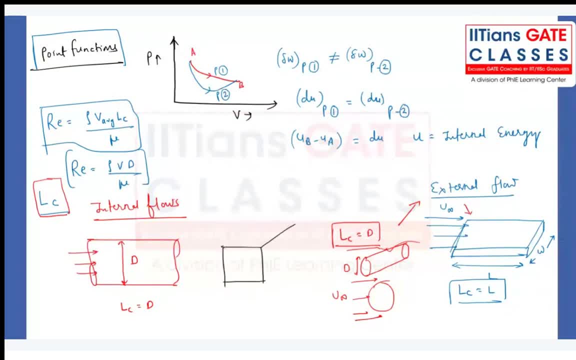 The non-circular section means something like this, In that I have taken one extreme condition. What is the extreme condition? See, there is no limit on thinking. We can think about any practical condition. We can get the idea. We can get the idea. 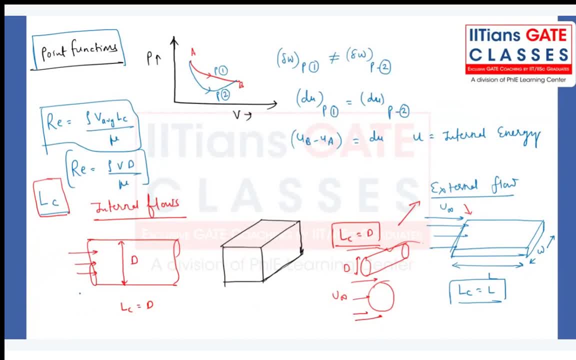 We can get the idea of that practical example. For example, if this surface and this surface is fixed one the top and bottom, one right, If the top and bottom is fixed one, this one and this one right, Then the flow and this particular left and right is moving along with the flow. 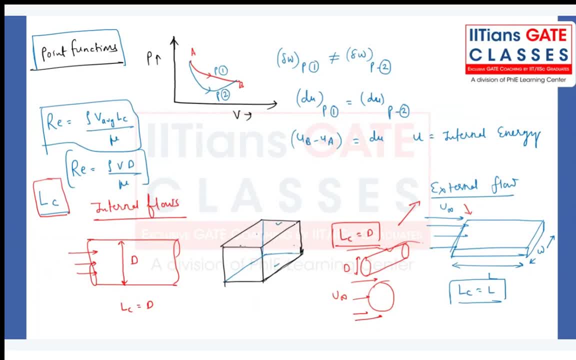 That particular part of the non-circular duct. it is also flowing, For example, in case of nanotubes, and all you will observe that If it is flowing, my dear friend, that case, in that particular case, my non-circular duct. 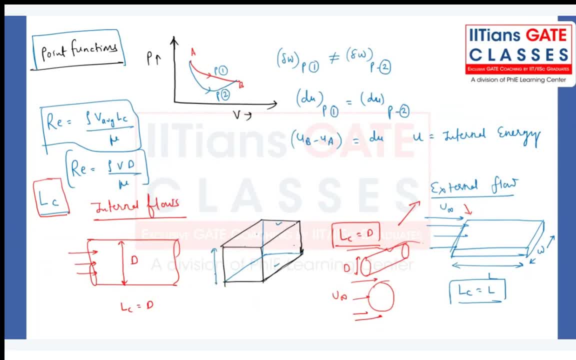 my particularly this one. what we call height will be important, right. But if that what we say, left and right is fixed, but top and bottom is moving, in that case width B will be important for us, Width B will be important for us. 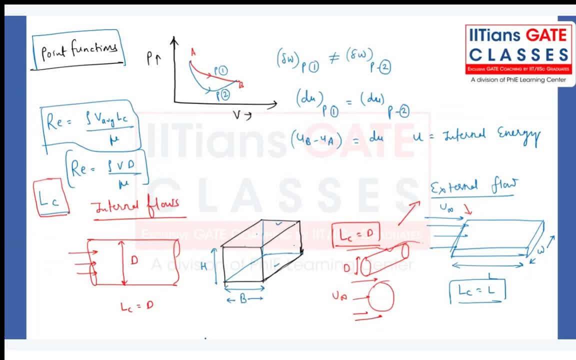 In particularly some situation. my dear friend, both the parameters will be important. In that case, now tell me which will be the characteristic length I thought to discuss in the laminar flow, but let us discuss here itself, So that everyone can understand. 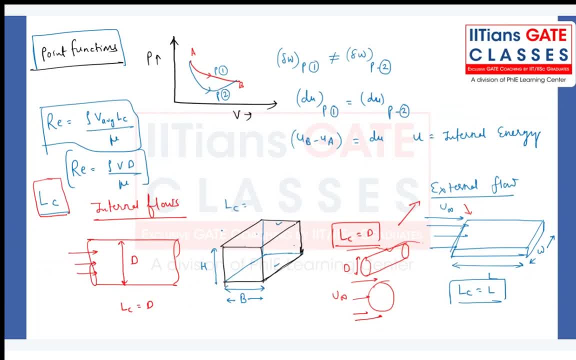 Okay, Everything will be clarified and we can make a compile notes. right, This will be the last one. Then we can discuss about the viscosity. See here, both the H and B will be important for us. So for that we have. it is only applicable for internal flow, that to non-circular ducts. 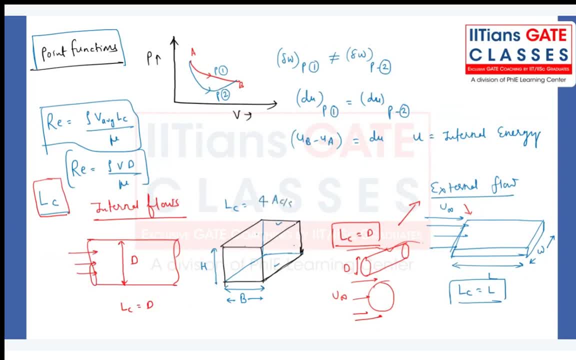 So you just write four into cross-sectional area by weighted parameter. Once again, it is not that important for aerospace guys, but still you can just make a note of it so that you will not be having doubt right Now. what is the weighted parameter? 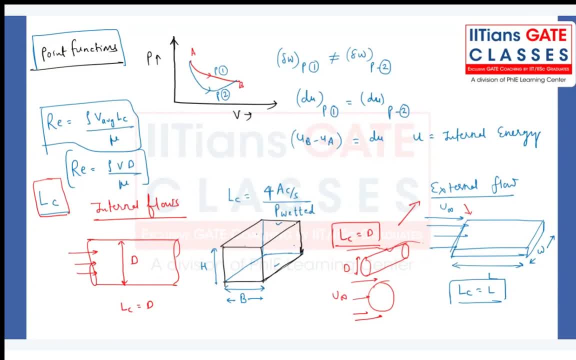 Now here it is very, very important. You can just calculate by using this particular formula for the cylinder case also: Internal flows through inside the cylinder. also How, What is the cross-sectional area, Therefore, D square right, And what is the weighted parameter? 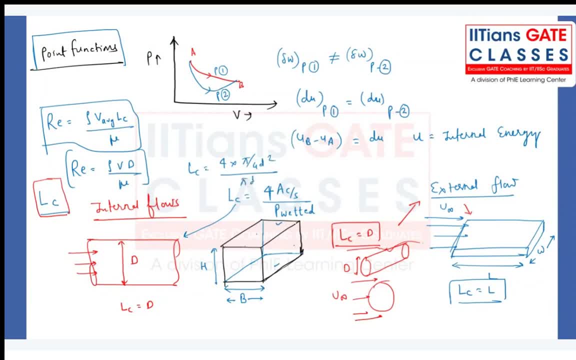 Pi D, right. So when you just calculate, you will be getting diameter only. Similarly my different. in case of non-circular duct, what is the cross-sectional area B into H And what is the weighted parameter? Two into B plus H. So this will be the formula where you can see B and H. both are playing. 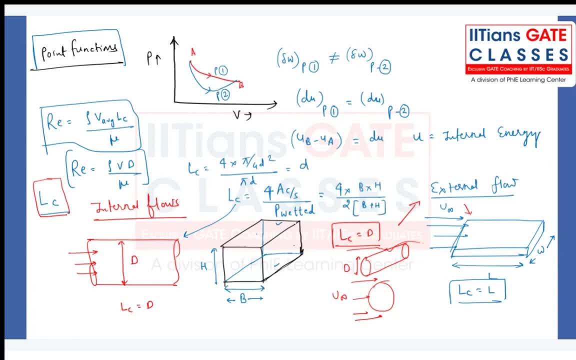 a very, very important role for this one, And why? Because in our last class also, I have said that whenever one parameter will be very, very large as compared to other one, then what will happen? Suppose, in such a scenario where width B is very important, B is very, very large as compared. 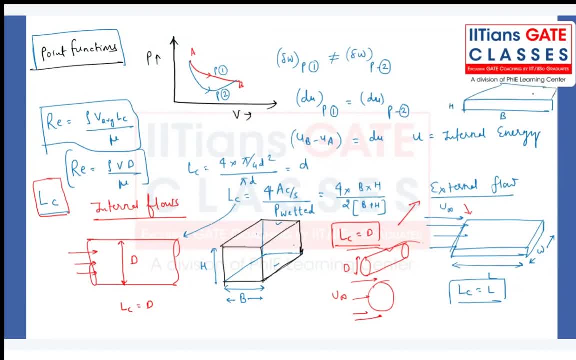 to height in a particular duct. Now tell me what will happen. B plus H will be B, only B, and B will cancel out. Then what? No, no, Think of once again this situation When B is very, very large. 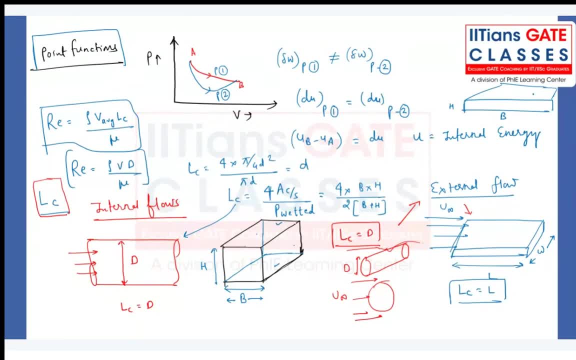 As compared to H. Then B plus H will be approximately equal to what B. only right. Then B and B numerator and denominator will cancel out H will be there. So smaller dimension will play an important role. Again, that is a very wider application we have. 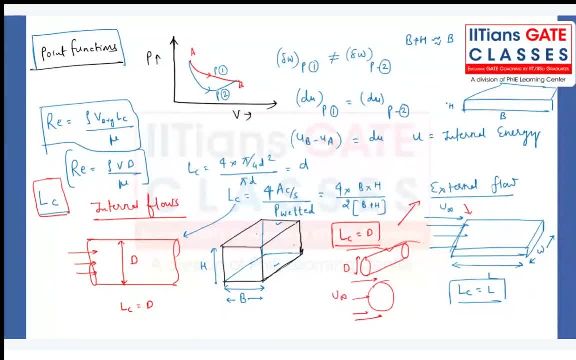 Not very important for the aerospace, but some of you who are very much interested for them. I am giving these ideas right, So make a note of it Again. this LC formula is not applicable for external flows. Remember that Only applicable for only applicable for internal flows. 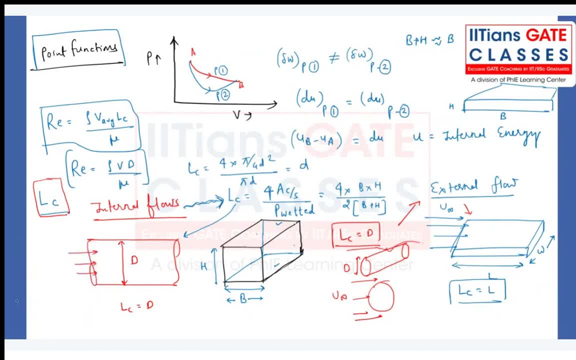 Make a note of it. Now we can move on to the topic called viscosity. Yes, for all, whether it is a circular one and the non-circular one. Non-circular it can be, you know, rectangular duct or square duct. 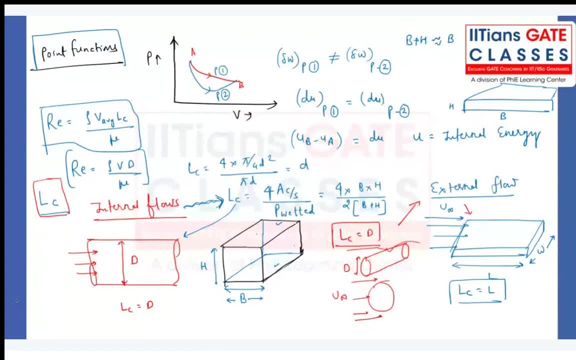 Because when you see air conditioning, your duct, you know big industries, you know you have to be careful. You have to be careful. There there is not a circular duct, They have the rectangular duct. Give him a point: What about the shape of what we call AC duct in particularly aeroplane? 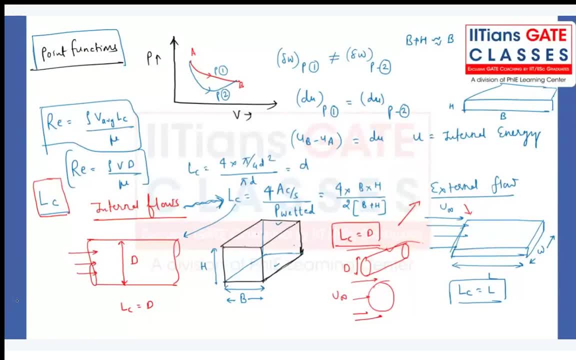 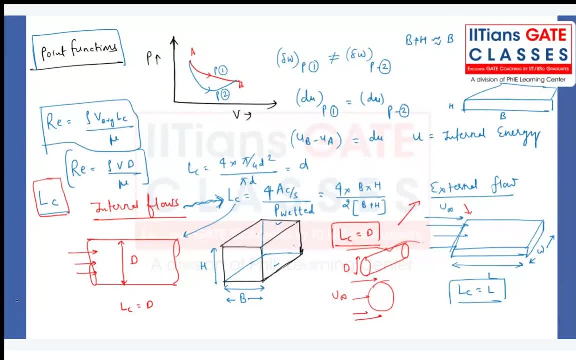 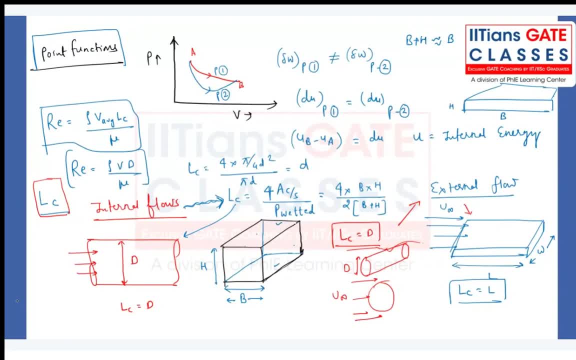 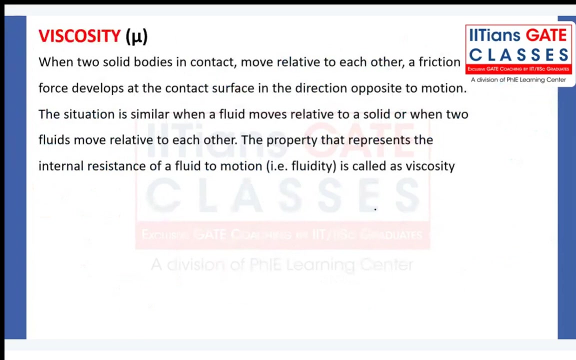 can always develop. Now, all of you, once it is done, let me know. Is it done? Can I move to the next one? Now note down the next topic. that is a very important: viscosity. So viscosity in a particularly, in a very simple term, if I give the definition, make a note. 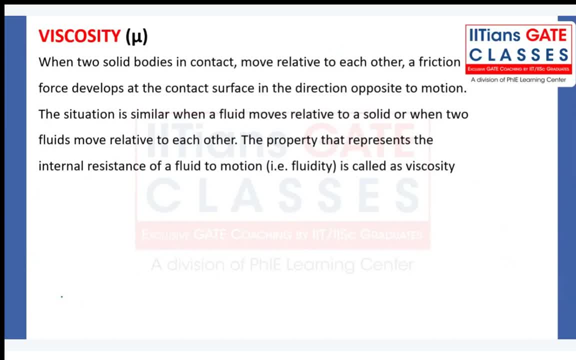 down. So what is the meaning of viscosity? Viscosity is the property of the fluid by means of which it offers resistance to what It offers, some kind of resistance to the what Motion of the adjacent fluid Right Correct, Just like in a particularly solid body. suppose we have any solid body example which is 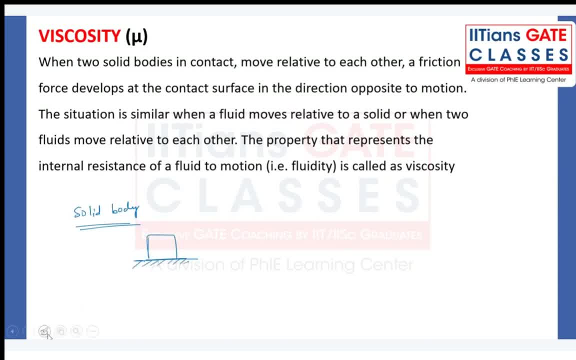 being placed on a rough surface. Now try understanding Correct. Viscosity means it opposes the relative motion between the two fluid layers. Getting my point Here. you try to understand. one more thing which I am talking about: Whenever any solid surface, any solid body is there, which 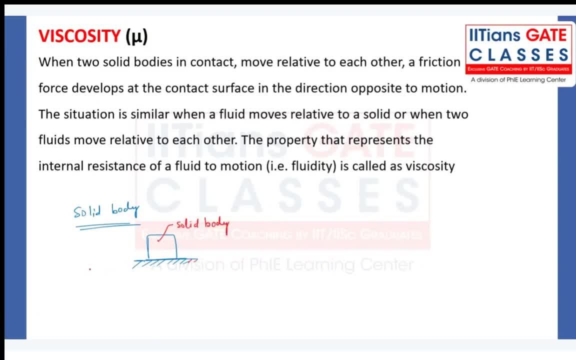 is in contact with the rough surface, what will happen? Whenever we are applying the force F, Then whatever what we have, the nature of contact here, this particularly body and surface- they will offer some kind of resistance. right When you draw the free body diagram you are: 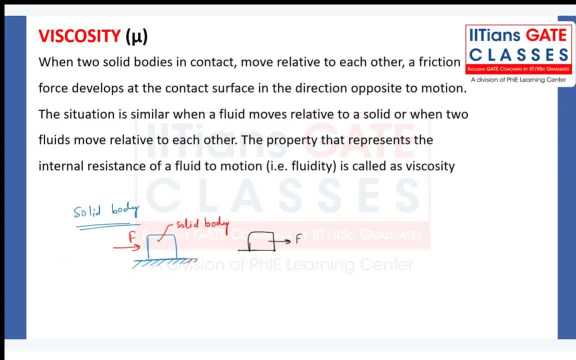 applying the force F, but there will be force of friction, will be acting in this direction, in the opposite to the direction of motion. This force of friction will be offered by the surface, this particular surface Getting my point. So here it is very important, in case of solid, just like what we have, frictional. 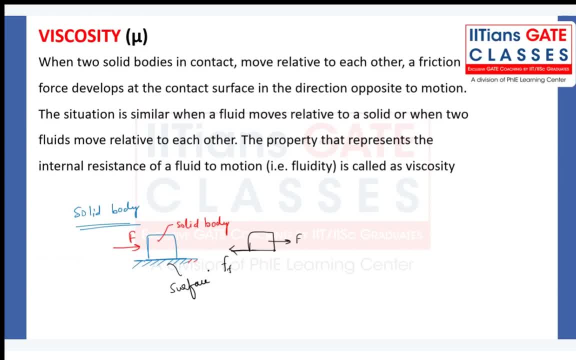 forces right In case of fluids. also, whenever a two fluid layer is there, this is a one fluid layer. Suppose fluid is flowing And when I just zoom it and if I consider only two fluid layer, which is in contact right, Which is basically moving, related to one other, 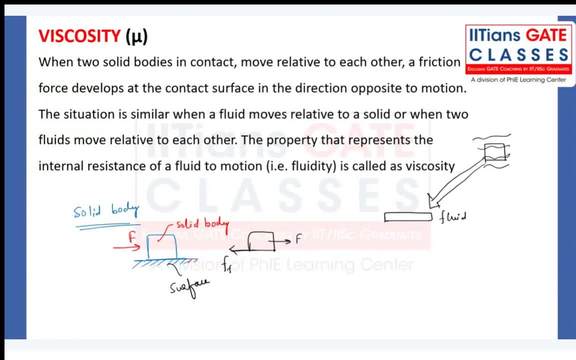 right. What will happen? Suppose this particular fluid is moving with some velocity U, dash and the second fluid layer, if I say here, which is moving with some velocity U, what will happen? What will happen by different. There will be always be resistive force. right Offered. 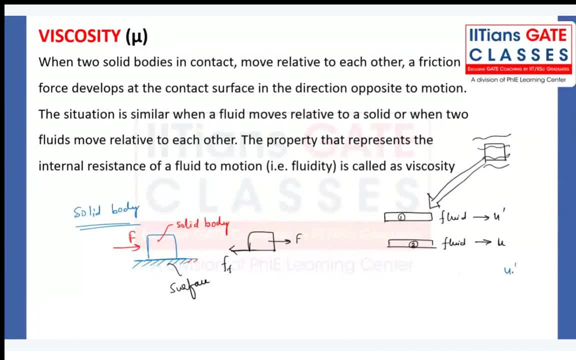 by the second fluid layer. Suppose U dash is more than U, then second fluid will offer some kind of resistive force to the surface, To the what Adjusting fluid layer. Whatever the fluid is there, they will offer some kind of opposite resistive force which is being opposed to the direction of motion of fluid. 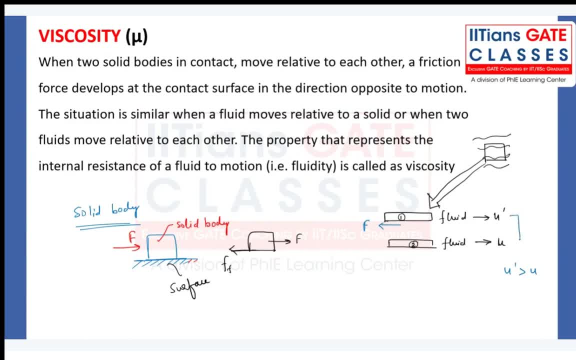 right, Because they have the difference in velocity. that's why the resistive force will be developed. But according to Newton's third law, if the fluid 2, fluid number 2, is offering some kind of resistive force onto the fluid number one, which is opposed to the direction of 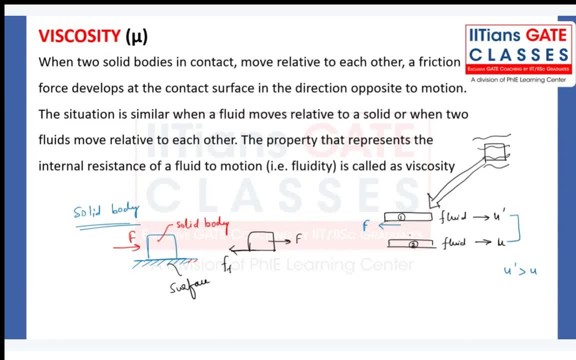 motion. The fluid 1 will also offer some kind of resistive force. Is there any point of reference here? No, there is no point of reference. Okay, force onto the fluid number two, like this, which is equal and opposite. getting my point, all of you? 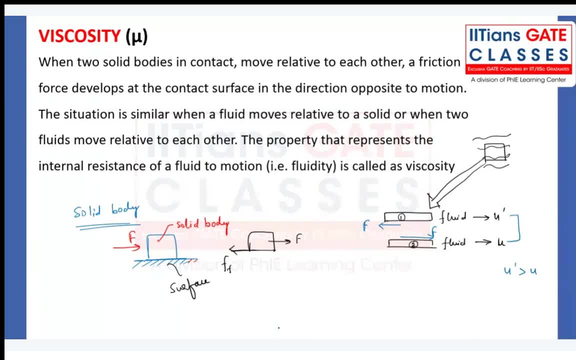 tell me, guys? so whenever the two solid body in contact, if they will try to move, related to each other, a force of friction? force of friction will be developed at the contact surface in the opposite direction of motion. this is a particularly very similar situation will be there whenever the fluid layer or fluid moves related to the solid or when the two fluids. 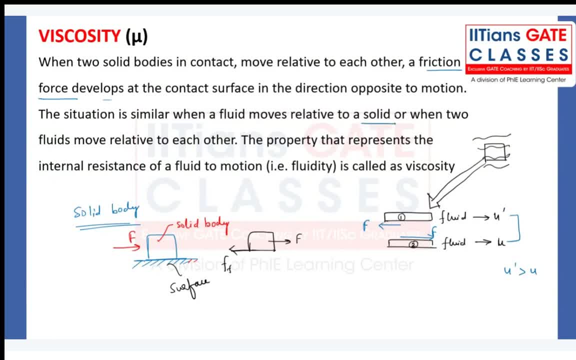 move. whenever the two fluids try to move, related to each other, the property that represent the internal resistance of that fluid to the motion will be called as viscosity. in a very simple term, what we can say fluid is a pro. viscosity is a fluid property, by means of which. 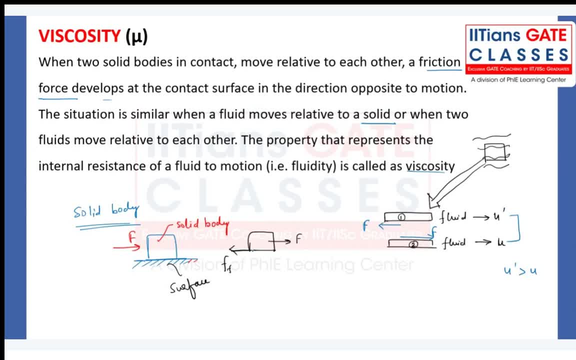 one fluid layer will offer resistance to the other fluid layer motion right, or, in short, can i say it offers some kind of resistive forces to the continuous deformation of the fluid layer. tell me, guys, can we say like that also? ultimately, whenever the fluid is flowing we say there is a continuous deformation, that continuous deformation should not be there, that 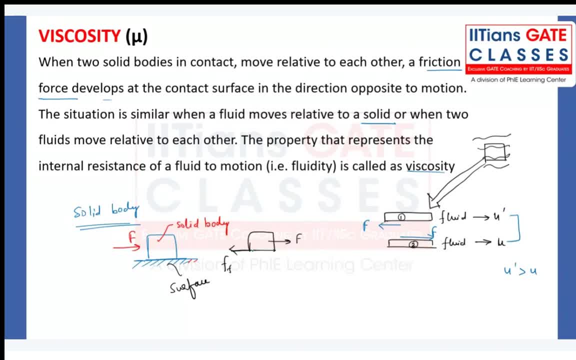 means the fluid should have very, very high viscosity, right? so in short, you can note down one more definition. so viscosity represents? viscosity represents the property due to which fluid will resist, fluid will oppose or assist the flow or continuous deformation or continuous deformation between the fluid layers. all of you are getting my point. viscosity always represents the property due to which 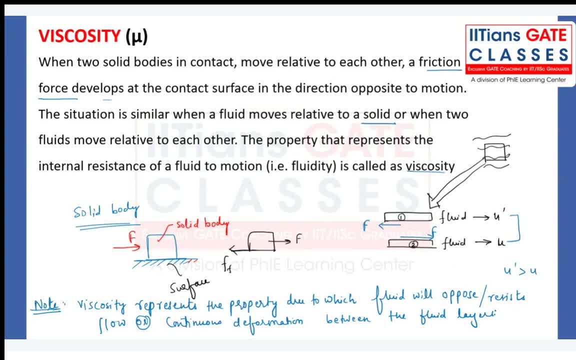 the fluid will oppose or resist the flow, or continuous deformations between the fluid layers. all of you getting my point? is that clear? right? we will try to see the physical significance also. yes, yes, that is just like a drag force, you know, that is just like a viscous force offered by the 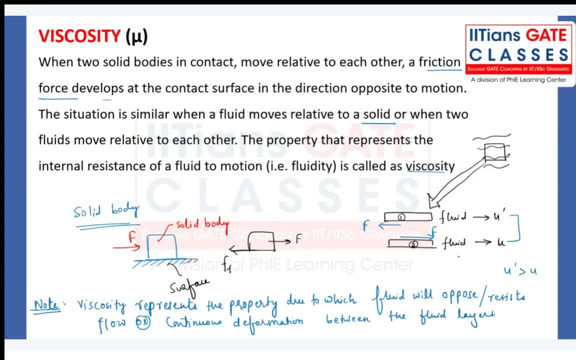 fluid layer one onto the fluid layer two, so that he, uh, what is the communication will be happening? what is the communication happening between the fluid layer one and two? first of all, fluid layer two will say: how can you, how can you move forward with such a high velocity? 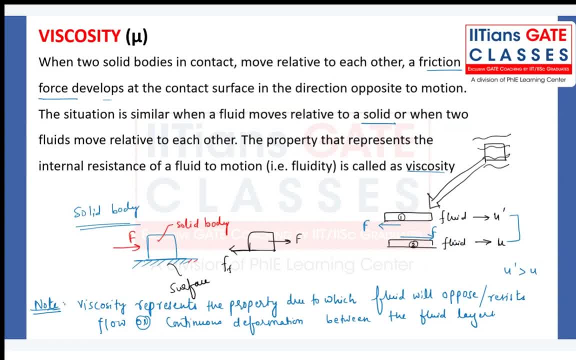 even you know that, and everyone know that. we have the bonding, we have some kind of- uh, momentary momentum, uh, we have to transfer some kind of momentum between us. right then, how can you move forward alone, right by leaving me? so what will happen? they will try to oppose it. you just come. 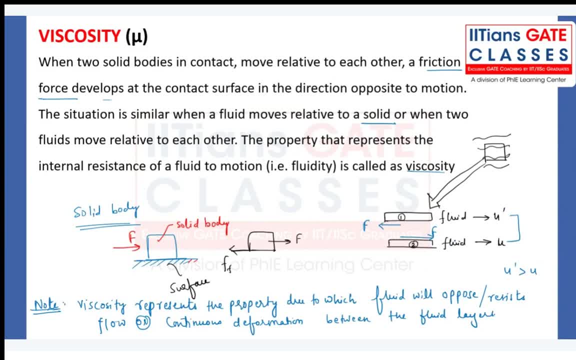 back. you just slow down your speed. what the fluid layer one will communicate to fluid layer two? uh, it's yours. if your speed is low, it's your fault, right? so i'm just giving you some kind of uh driving force so that you come to my level, whatever the velocity is there you try to achieve. 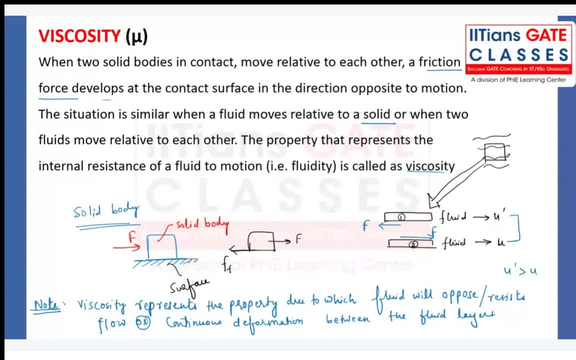 my velocity particular value so that it will offer some kind of driving force in the same direction onto the fluid number two. getting my point, once i will discuss the physical significance, that communication will be more clear. uh, what you're saying, isn't it the contradictory to the statement that fluids cannot resist? 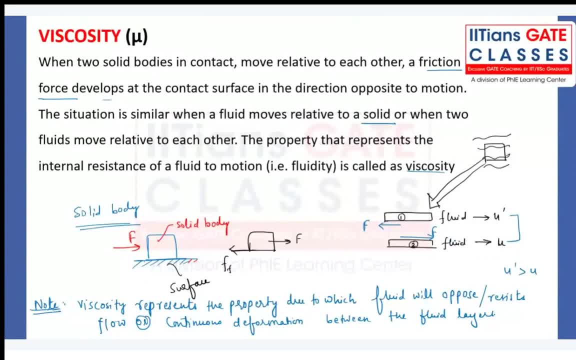 external safe force. no, that is a inherent fluid property. you know i'm not particularly talking about the external safe force, whether they can able to resist or not. i told you in the beginning of the subject, however small safe force you apply, the fluid having the tendency to deform. 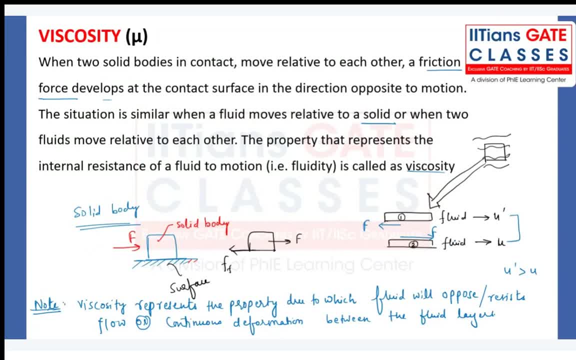 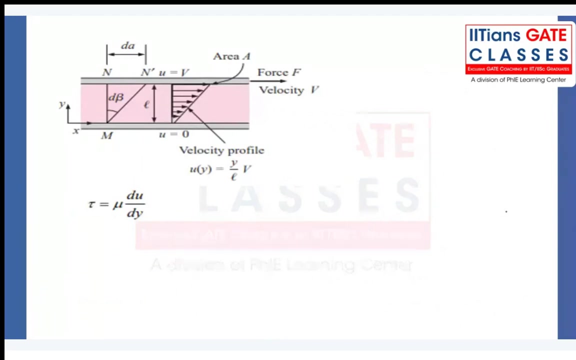 continuously getting my point right. we will discuss more in detail. all of you have noted down bad main. now is it done. now we will try to see uh some kind of uh scenario, example where we can uh analyze this particular situation right, for example. now for this example, what we are observing? there is a plate which is 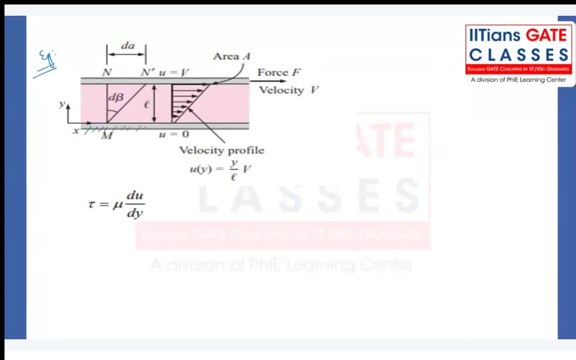 being fixed. this bottom plate is fixed, one and the top plate is moving with some velocity. my dfn, what you can observe, the top plate is moving at some velocity v. that is a constant velocity. right, that is a constant velocity. what will happen? whatever the stationary fluid will be there. that 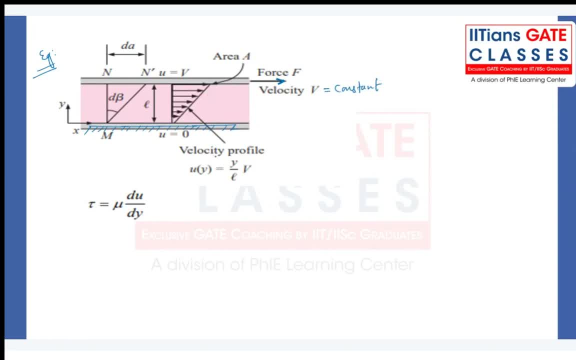 will be also start flowing with the. what top velocity. anyone in the class can tell me why it is moving at some constant velocity? because the top plate is moving at some constant velocity, so it is moving with the velocity of the. uh, why it is start moving with the top plate? 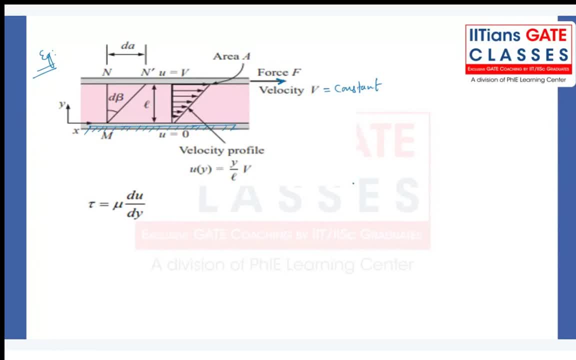 perfect now, what is the no slip condition? to understand that, let me discuss that phenomena: no slip conditions. perfect now, what is the no slip condition? and all make a note of it, because if you understand this thing, then you will understand boundary layer theory very easily. always remember what is the meaning of no slip condition and what is the proper definition of the. 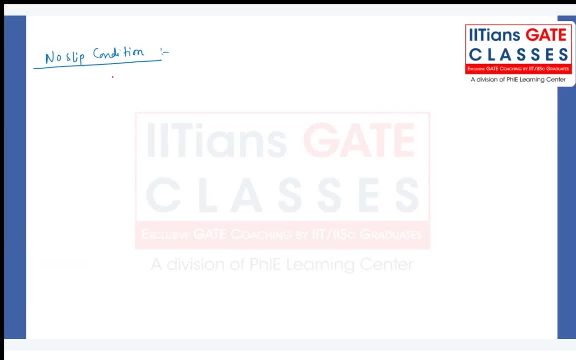 no slip conditions. no slip condition: whenever the fluid is flowing over any solid body, then the relative velocity between the fluid and the solid surface will be zero, right so down, whenever the fluid is flowing. a fluid is flowing over any solid surface, over any solid surface- our body. 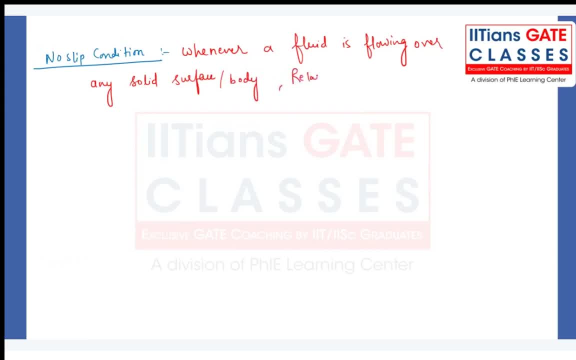 the relative velocity. the relative velocity between solid surface, between fluid and solid surface, will be zero. the relative velocity should be zero. that is the meaning of no slip conditions. that means let me give you one example of what we call flow over the flat plate. If I talk about the flow over the flat plate condition, the fluid is flowing with the velocity. 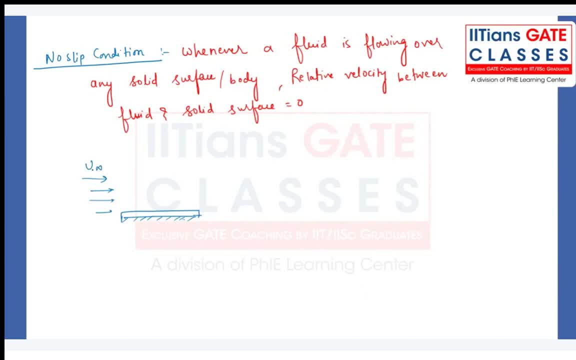 free stream condition. Free stream velocity means U infinity, what we call free stream velocity. Now you try to understand from here each and everything very carefully Now and after that you can ask doubt if you have, Whenever the fluid is flowing in a particularly in a laminar manner, flow over the flat plate. 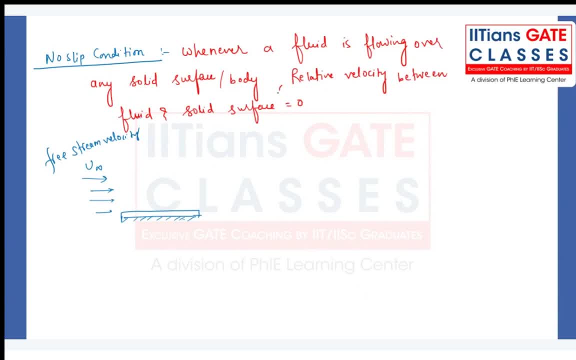 conditions here, what will happen? The plate is at the rest condition if I just extend little bit the length of the plate like this, So whenever the first fluid particle it will be coming in contact, If it is coming in contact with the flat plate, what about its velocity? 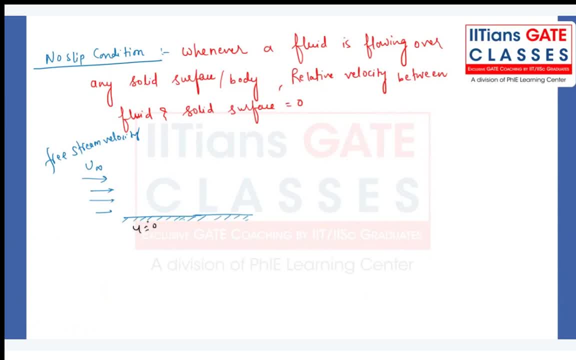 The moment it will see that the plate is having zero velocity, the fluid will also be having zero velocity. Then what about the first fluid particle velocity that is going to be zero? Why it is going to be zero, Why the fluid velocity is going to be zero? 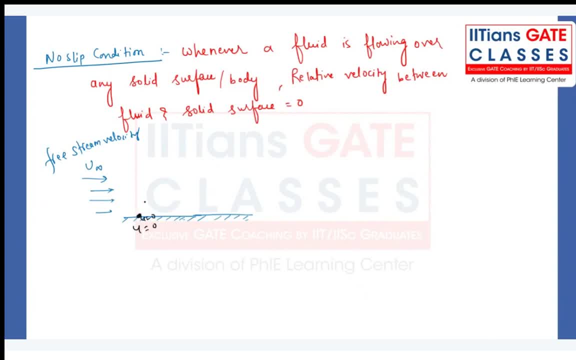 To satisfy no slip condition to satisfy. to satisfy no slip condition. Whatever, the first fluid particle is there which is coming in contact with the flat plate will have to have the zero velocity Because the flat plate is being fixed, Because the flat plate is being the fixed one. 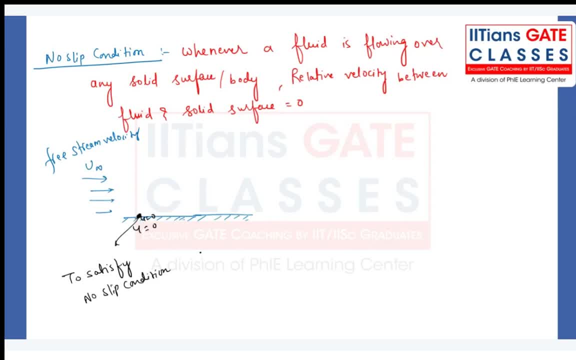 Now what about the other fluid layer which is in the above one, For example? earlier I have taken the free stream velocity layers, layer number one, two, three, four. Let's see what the communication will happen in between all four fluid layers. 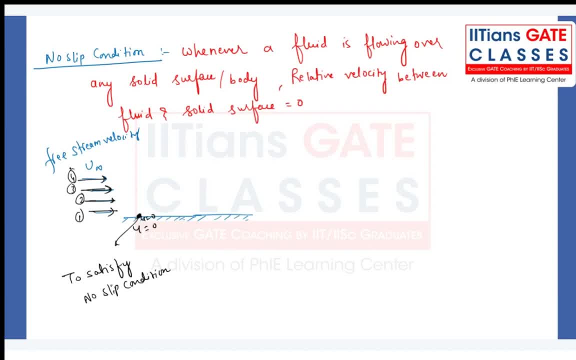 Let's see that and try to understand the situation very, very carefully. Now, here, when you talk about the fluid layer, When you talk about the free stream velocity which is approaching the plate, the first fluid layer is getting what? Zero velocity. 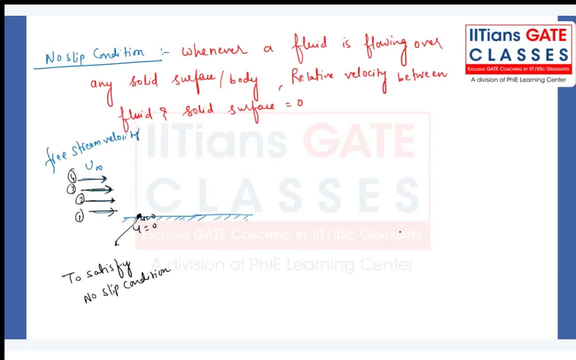 Now what the message will pass to the second fluid layer. Will it be moving with the same velocity as U infinity, or will it be moving slower than the U infinity? Tell me, guys. it is a very, very important When you see that, whatever the second fluid layer will be there, it will not be moving. 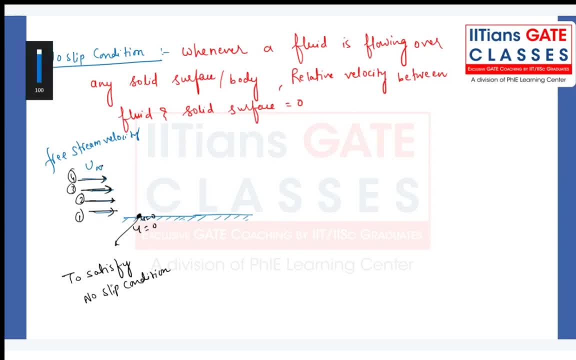 with the same velocity as galvanized fluid layer. It will not be moving. That of the earlier case, that is, free stream conditions. It will be moving somewhat with the lesser speed, something like this, Let's say the velocity called U. What about the third fluid layer? 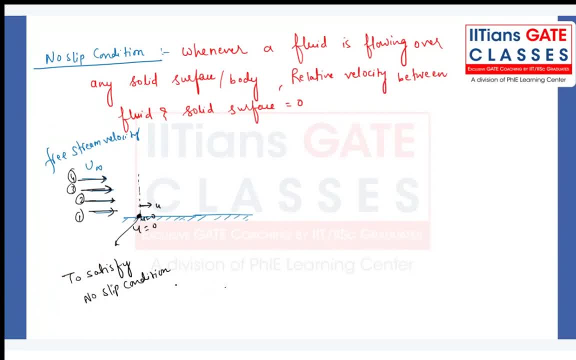 When you talk about the third fluid layer, what is going to be happening? It will be having a little bit more velocity than second fluid layer, or lesser velocity as compared to the second fluid layer. after hitting the plate, It will be having more particularly velocity. 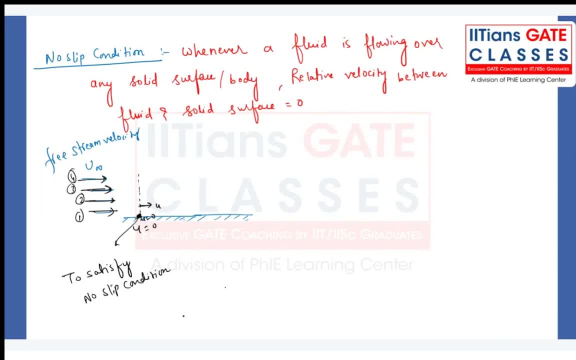 Now my question is: why? why it will be having more velocity as compared to second fluid layer. Now see, whatever the third fluid particle is there, the third fluid particle having two chances? What are the two chances will be happening with these third fluid layer? 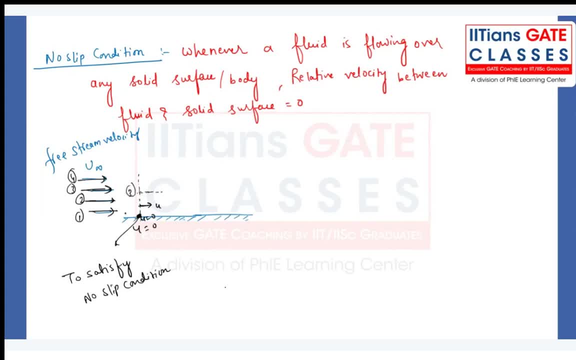 The third fluid layer which is being talked about here below third fluid layer. second fluid layer is there. Above third layer. fourth fluid layer will be there And obviously this is the third fluid layer. So what will happen? The third fluid layer is going to be moving at the same speed as galvanized fluid layer. 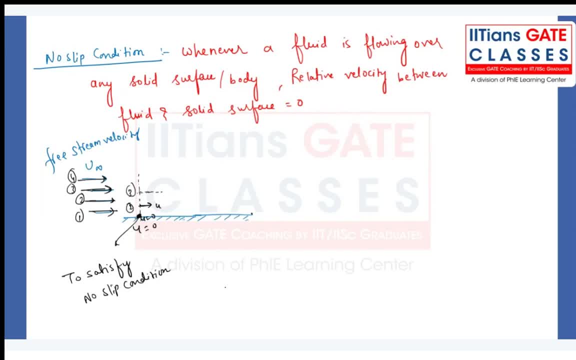 as you keep on marching along the y direction. this is the x direction. if i talk about cartesian system, if you are moving in the y particularly, direction, effect of wall will be felt very, very low as you keep on moving away and away and away in the y directions. because who will pass the 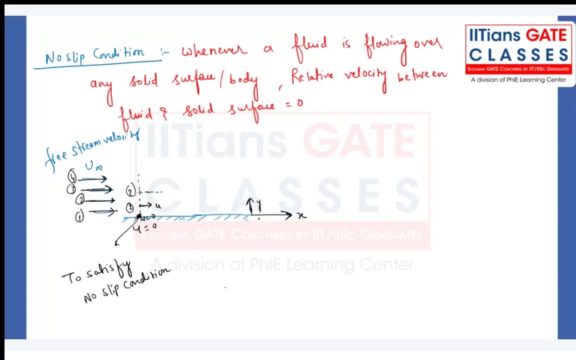 message that the fluid, the plate is being fixed, one who will pass that message among the fluid layers, viscosity, viscosity here will play a role of messenger. one right so, and you know that whenever messenger we talk, that is a human ability. human ability means what here? fluid property. 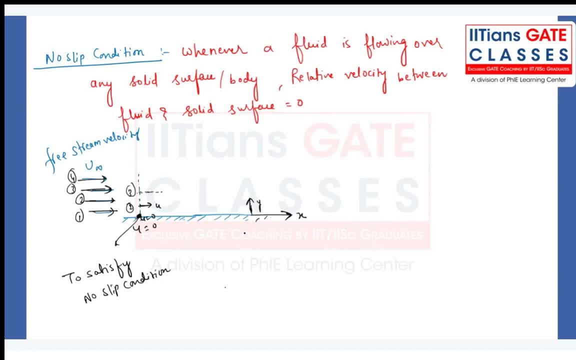 that's why the name itself is given, that whenever the fluid is being fixed, in any circumstances, you cannot change the viscosity. that is what we call. that is a fluid property, right? so third layer in a competition above fluid layer: more velocity below fluid layer, lesser velocity. in a particularly competition of that. 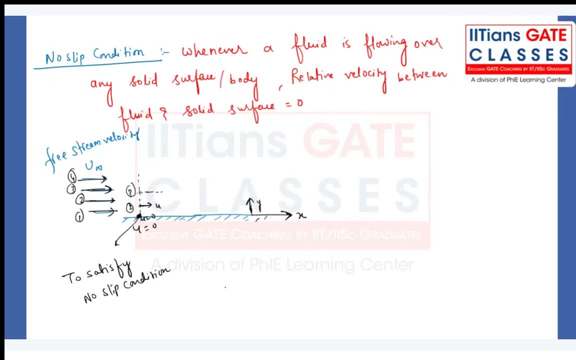 it will move little bit with the more velocity as compared to second fluid layer and the fourth fluid layer will be moving with somewhat higher velocity than this. slowly, slowly, if you just see that there will be some kind of velocity gradient will be existing right if we join this. 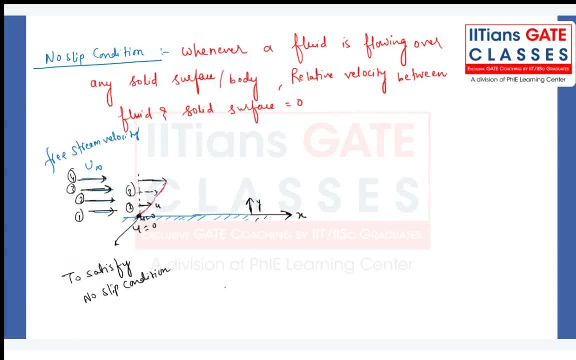 one. it will be developing some kind of- and after certain distance, my dear friend, the velocity, the plate velocity which is being fixed, one or effect of wall will not be felt. it will be constant right, for the fluid layer will be like that right. this is called velocity profile. 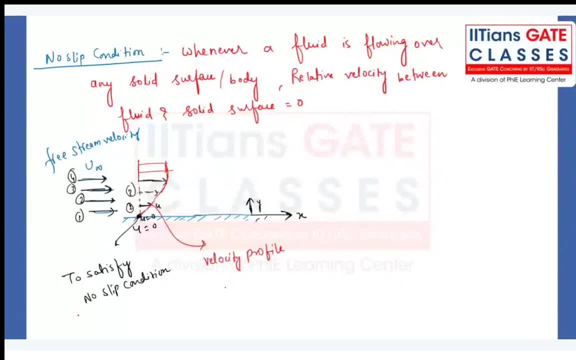 right now, when you come over here after certain distance, right, initially very, very less fluid particle is in contact with the flat plate. but when you talk about at this particular place, at this particular place, even though viscosity is being same, but what about the nature of the fluid velocity? 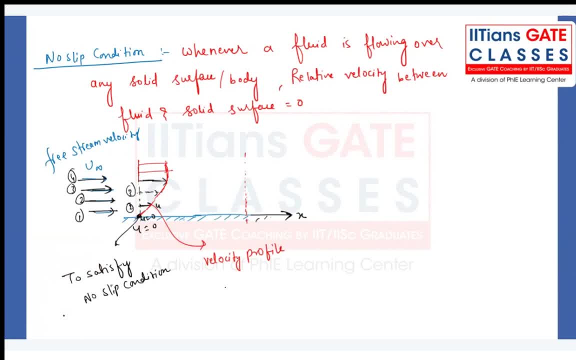 of individual layer of the fluid. what about the second fluid layer? will have more velocity than u or will have little bit lesser velocity than u? tell me guys? in the first case, all the fluid layer are moving with the same velocity profile, like a uniform velocity profile u infinity. 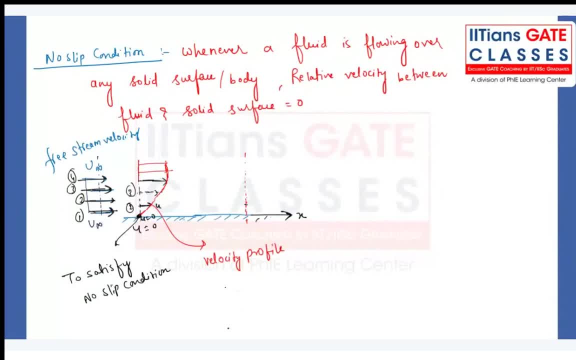 after hitting the plate, the particles are feeling some kind of slowness because of plate is being fixed one. but after traveling certain distance from here to here, what is going to be happening? my different. the second fluid layer will have further lower velocity than the watt at this. 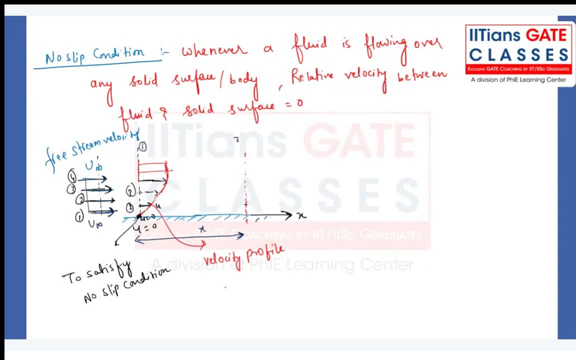 location, location number one: the fluid velocity velocity of the second layer in the second scenario, or in the second situation, or in the second place, will be lesser than the second layer, than than the first case, why it will be having lessen. now more and more amount of fluid will 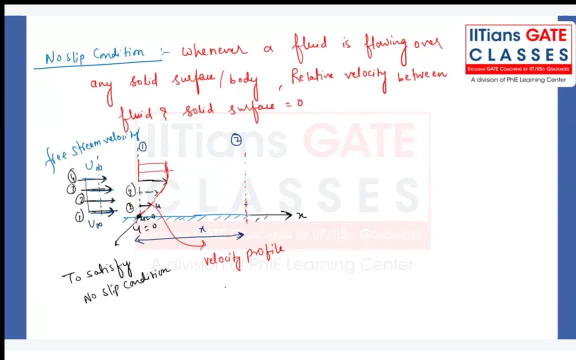 be in contact with the flat plate. earlier, only few particles are in contact, so that many message will not be propagated in the y direction. but now more and more fluid layer will be in contact with the flat plate. then what will happen? all will pass the message to the above fluid layer that 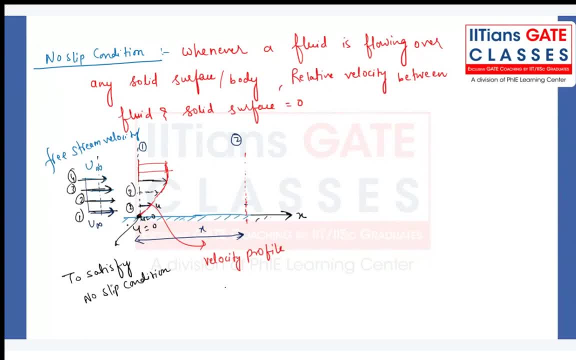 there is a sudden distraction happened. there is a sudden, uh, i know, uh, this, what we call the resistance to the motion happened by the flat plate, so all the fluid particle. they will think that, okay, something big thing happen at the location y equal to zero. so what will happen? 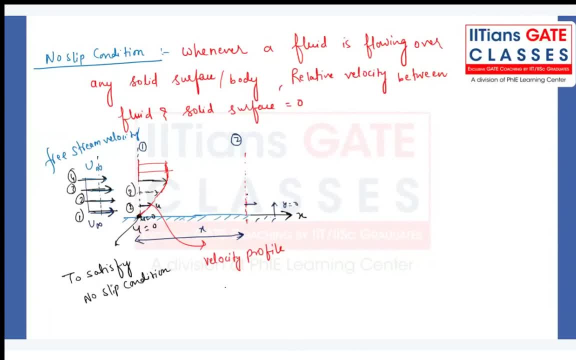 they will start moving very slowly and they will try to achieve the free stream velocity at little bit, somewhat higher distance than the earlier one. same free stream velocity might happen 0.99 times of u infinity. it will be achieved at a certain higher distance than the earlier one. 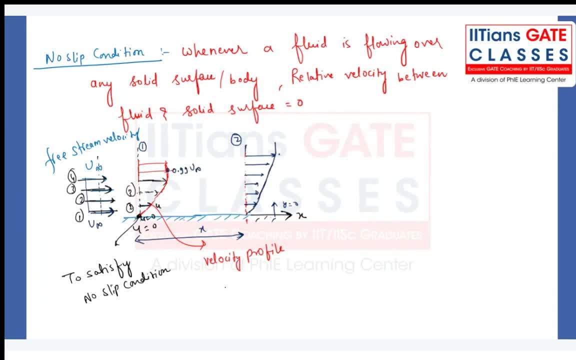 in the y direction as compared to earlier case. why? because effect of wall has been uh, you know, basically, uh, whatever the message is there, that plate is being fixed that is being propagated at, certainly among the high flow of a very large fluid layers. so that's why fluid 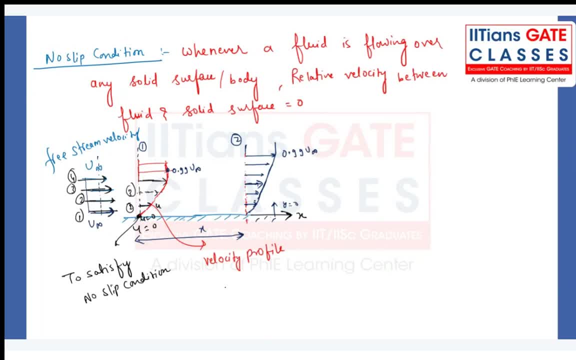 particles are taking certainly larger distance as compared to this one. so when you join from here, my different from the leading edge, when you join, you will form. you will form these flow, this particularly locus of all the fluid particles, where it is achieving the extreme conditions. when you join the locus of all these things, you will form certain. 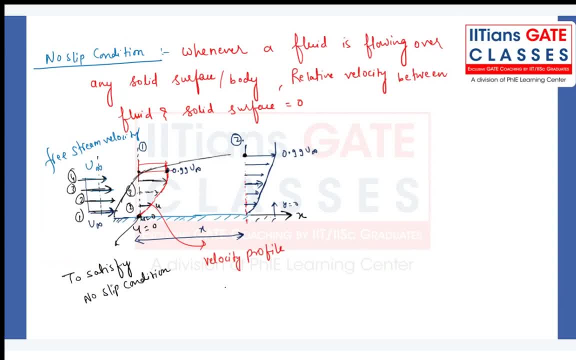 layer, this layer of the particulary uh, this particular layer, what we call, when you join the peaks of uh free string condition, which is being achieved by the fluid layer after hitting the plate, that particular condition of that particular plate, that particular layer, will start happening later on. and then v2, starting out from that particular lab type zone, is, you know, you willear theOMv3 component after hitting the plate, that particular condition, that particular casual application for this constant flood condition like that, so into formation while you will verify if the vendoing has been accomplished. finally, the law of motion is gonna temple P ale of whatever profile ancestry of this particular part from this fuel, of all the fluid, V, heaven, air. second, at the level of elementAthe Megatonis membrane is clear, which is junked inuw frequent work'. 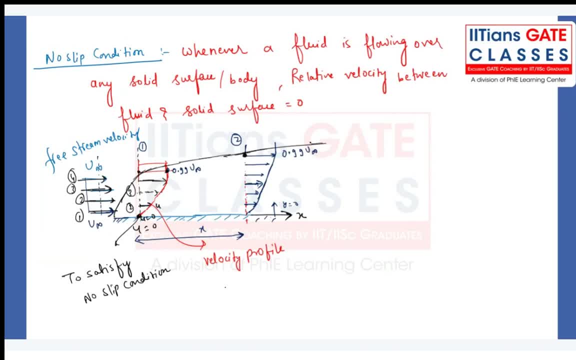 particular layer will be called as what this layer will be called as boundary layer, right? so remember that. my different here. yeah, that's why you will see always boundary layer. it is growing, right, so when you just talk about here, it is having when you draw very carefully. 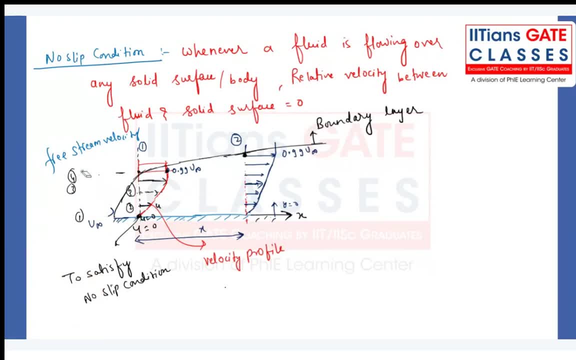 about this. let me draw once again here a little bit far from this leading edge. so here, when you just say here this is a delta one boundary layer thickness one, here it is taking a certainly more distance as compared to delta one. now the reason, reason is being clear, right? so what about the reason of viscosity, if i ask you? 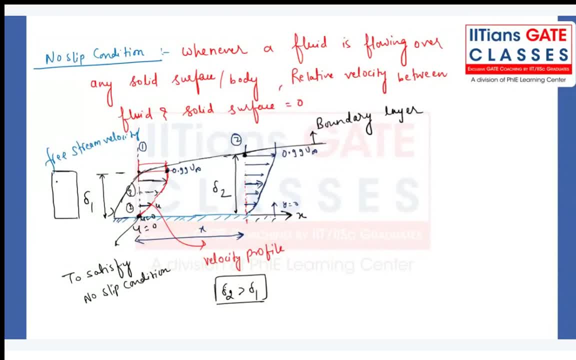 what you will say: uh, what about? what about the reason of boundary layer formations? not the reason of viscosity, the reason of boundary layer formations? you will say certainly. so, yeah, no slip condition. that is there. even no slip condition is there, but no slip condition is happening. because of what? viscosity only correct if viscosity of the fluid is zero. my 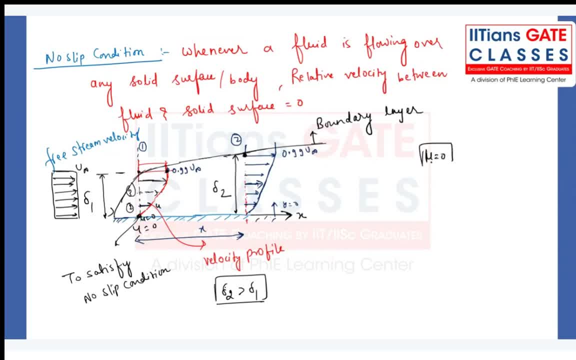 different. if the viscosity of the fluid is zero, what will happen, even though plate is being fixed? even though plate is being fixed, and whenever the fluid particles which is being approached, what will happen? they will certainly not follow no slip conditions, they will have same velocity profile as the earlier one and there is a no boundary layer. 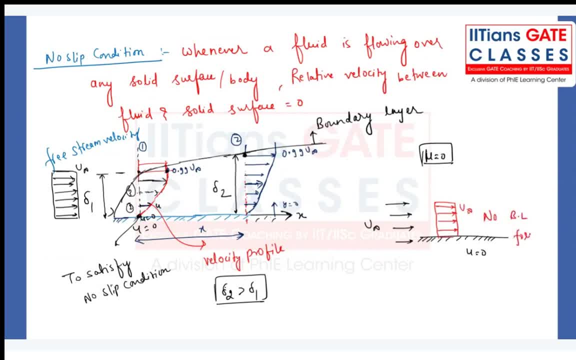 formation. there will not be any boundary layer formations. as you can see here, there is a slip has happened. now my question is: see, i am not here to discuss about the no slip condition and what we call boundary layer formations. that is being discussed by maybe other faculty also. 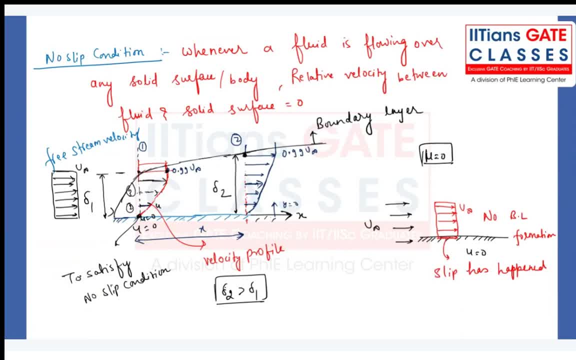 and you might have discussed in btech also, you know, by the professor of your college. but if you are coming over here at igc- something you should be getting extra right. my condition is that my question, or what, what actually i want to ask, is that: do the liquid or gases? 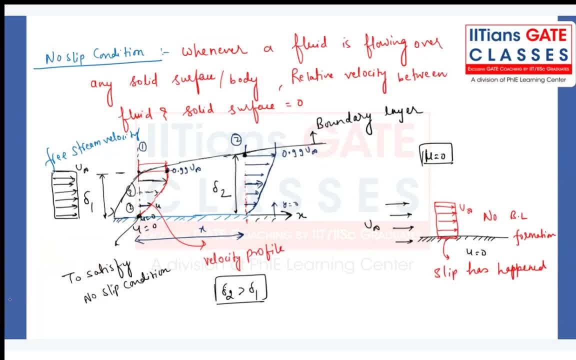 always satisfy this: no slip conditions. or maybe, if i just reverse my question, do this what we call no slip condition: in all the practical application will be justified. or we say, we observe, or in any cases you observe that it is not being satisfied but still the flow is happening, or we may have the practical application or outcome of that application. 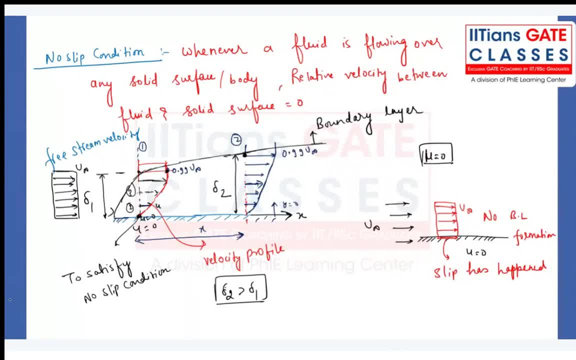 right. so all these things are happening just because of what they will try to resist the motion of adjacent fluid layer. and who will try to resist that? particularly motion of the adjacent fluid layer is the viscosity of the particular fluid. Now you try to understand what I am actually talking about. 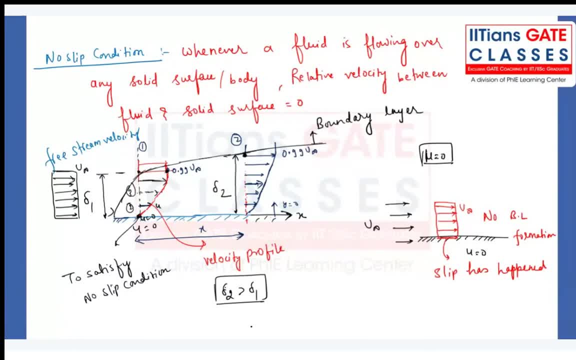 Suppose, if you keep on moving away from the earth's surface in a space, basically if you are sitting in a space where fluid particles are not that high in number, or maybe if I talk about the vacuum condition in a particularly vacuum situation, my dear friend, there will. 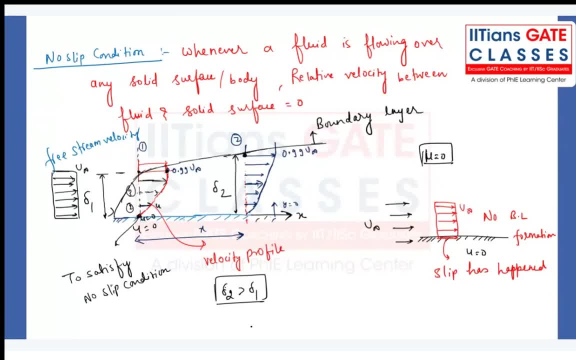 not be large amount of fluid particles. If I talk about the gases, the gases particles will not be in a large number in a particularly vacuum or rarefied gases theory. In that rarefied gases theory or in a particularly vacuum situation we don't have that many. 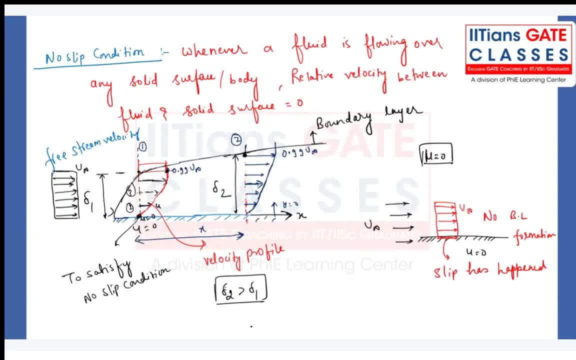 number of gases particles If we don't have that many number of gases particles. now, my dear friend, you only tell me that any momentum exchange will happen between the gas particles. no right, If there is no, that much of particle is there. there is no moment. is there lot of momentum? 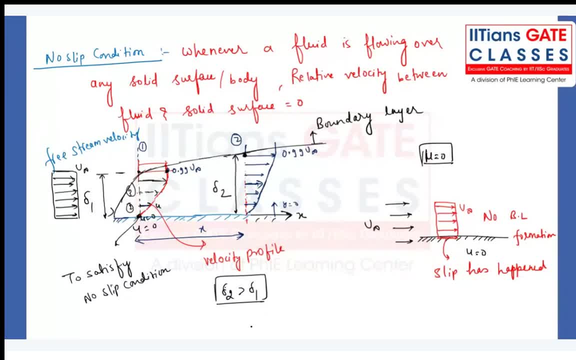 exchange is not happening, then what will happen? Then what will happen If I place a particularly fixed plate in that domain where, in a vacuum, or maybe in a certain space application, where the fluid is flowing over that plate or gas is flowing over that plate? they may not be able to satisfy no slip conditions. 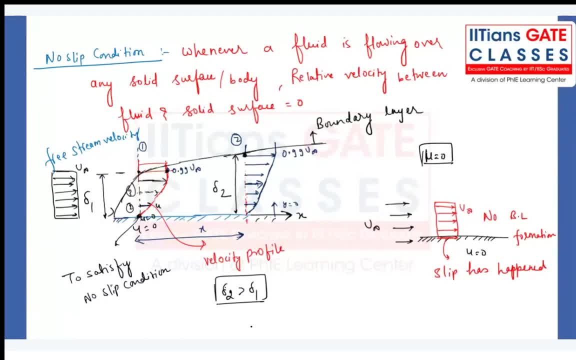 There will be slip. There will be some kind of slip in that particular case where- remember that- where effect of viscosity is not felt very high. So that is regarding the gases. Now, can the liquid always satisfy the no slip condition? Again, that is not true. 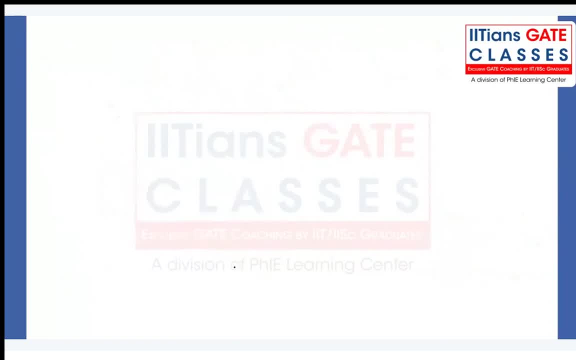 Again, that is not true. Remember why, if I just if you just look at very carefully Now, if you just look at very carefully, the fluid particles which are flowing with some velocity U infinity, and that is being flowing over the flat plate, that is being flowing. 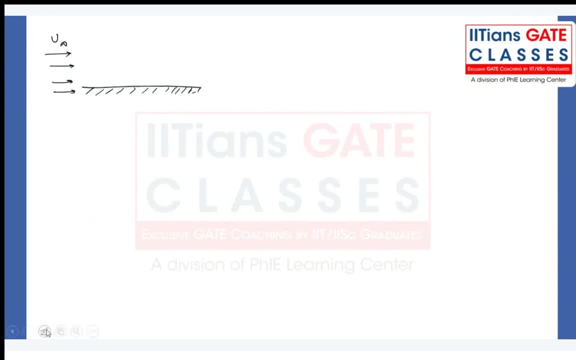 over the flat plate. why the fluid particle is having zero velocity right Whenever it is coming in contact with the flat plate. why the fluid particles are having zero velocity. If you just zoom it right and when you just look at with the microscope what you will. 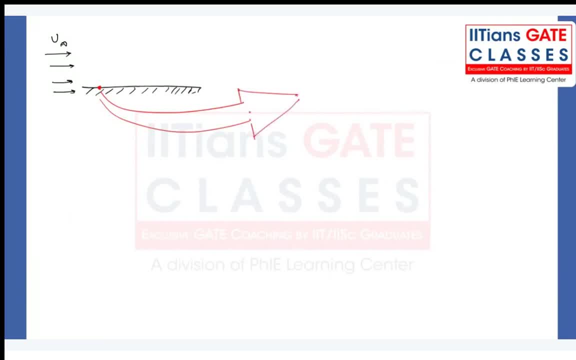 be observing. yeah, correct, correct, in a hydrophobic condition, my dear friend, that is the slipping will happen. right, Slipping will happen. Getting my point Now, Aman, you are from mechanical background, or what? 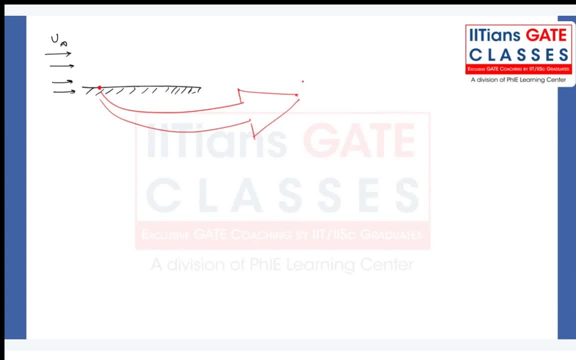 Zero, fine. Now when you just look at the microstructure of the, this surface, that surface will not be, the plate will not be smooth, right, There will be some kind of roughness. right In that roughness, my dear friend. 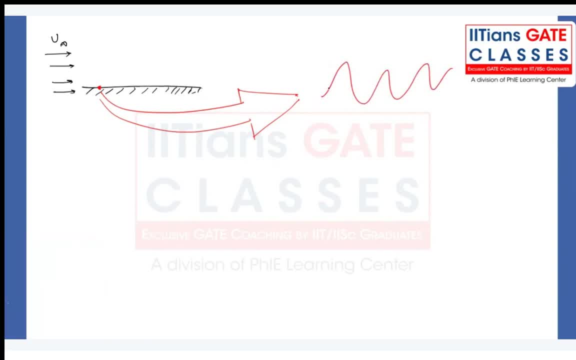 Yes, whatever the fluid particles will be there, they will try to stick with that and they will getting. they will be what getting locked? they will be getting locked in that rough surface. they will be getting locked in that particularly rough surface. my defense, and that's why they satisfy the no slip condition right, if i talk about the liquid, 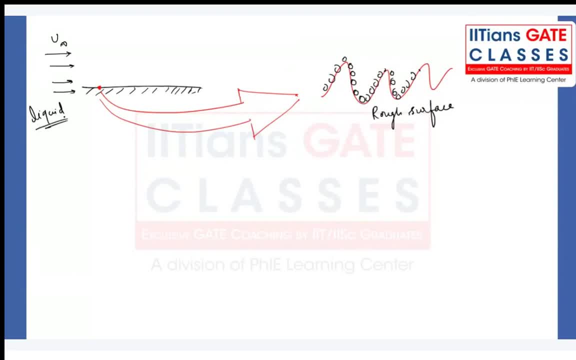 but when you are applying a a very, very high amount of shear force, very, very high amount of shear force, such a way that this locked liquid particles are coming out or jumping out from this particularly, uh, locked places, then what will happen? they will slip, they will have the velocity. 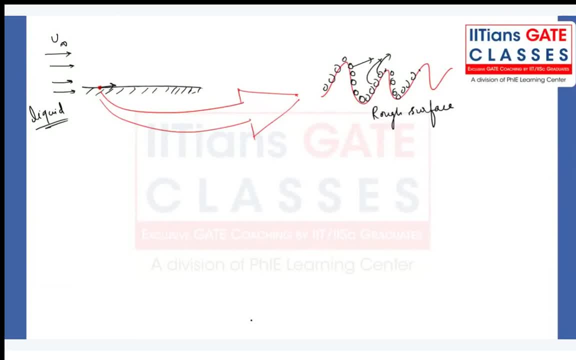 in that case, my defense: slip condition. no, slip condition will not be satisfied. that is the first scenario. second scenario: when you talk about the carbon nanotube, right, right, when you talk about the carbon nanotubes in that nanotubes, they are very, very smooth tubes. 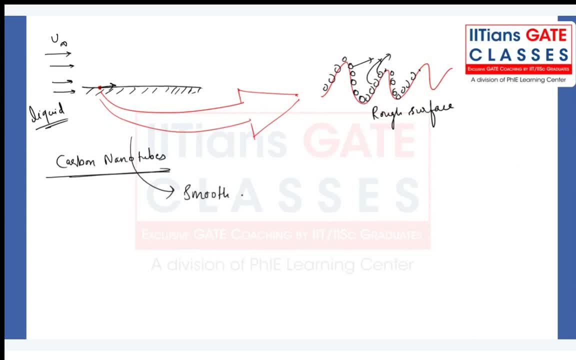 in biomedicals or maybe in aerospace application also. we use it right being uh mixed with the composite material to make the uh aircraft bodies right. in that case, my defense: when you flow the fluid in that smooth nanotubes, you know what will happen. very, very smooth nanotubes. when you talk about the carbon nanotubes, they are very, very smooth. 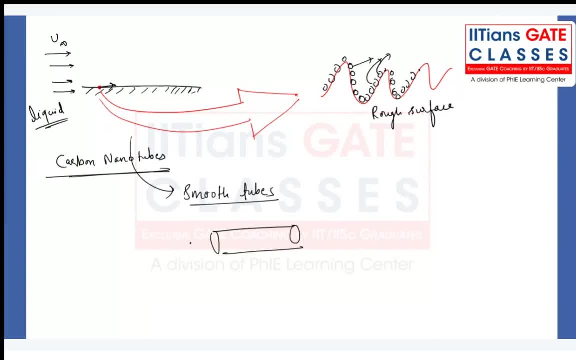 structures. they will not be getting locked. there will not be any rough surfaces there right against clip quedar. again, slip will happen right. so in those scenario, my defense: what will happen? no, slip condition may not be satisfied by the liquid particle, also by the liquid particle, but on the charge. topor. all the fluid particles are in fact notسب speeches or reaction of some��. You cannot allow carbon nanotubes to to apply. propose getting inside carbon nanotubes, so this should be completed easily, but i think we can focus on that as an approach for several. 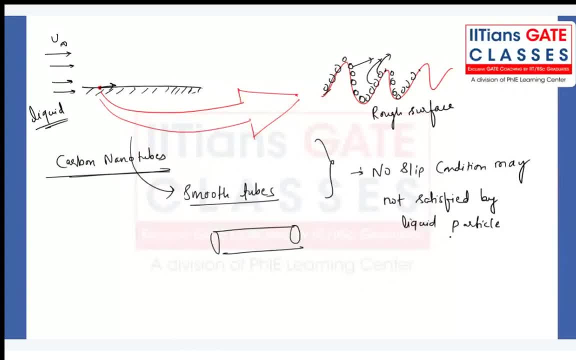 minutes history that i want to give you a very, very high guys research. what actually is a concept for those twoCooled by the? The good news is that, whatever the thing we are going to cover in our fluid mechanics course, we will talk about no-slip condition only. 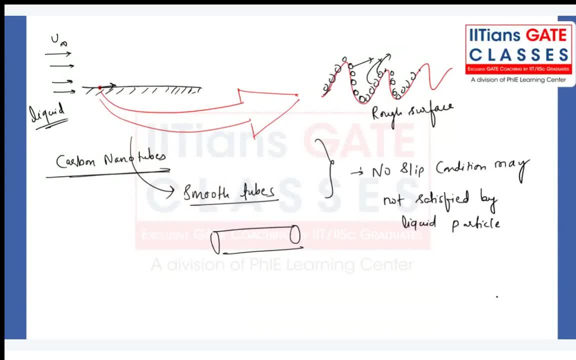 We will talk about the situation of the fluid flow where no-slip condition always satisfied, right, Because we are talking about this situation by different rarefied gases theory. right, Rarefied gases theory where the less number of particle is there in a particularly situation, right? 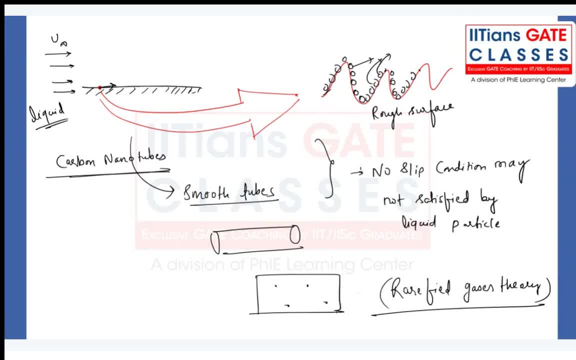 The rarefied gases theory means we talked about the situation where the pressure is very, very low, right? Maybe you can say it will, I don't know. basically it will give the same sense of feeling right. Slipping will happen in a hydrophobic cases also. 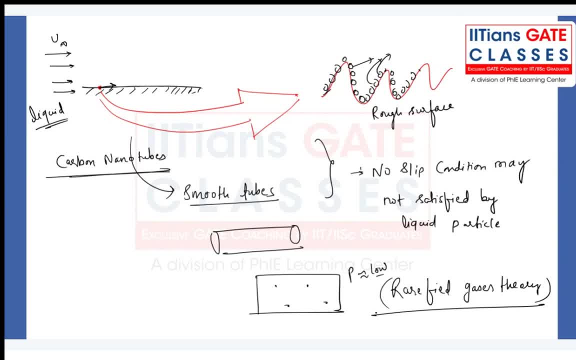 Getting my point: Slipping tendency will be there in that scenario right. So in a rarefied gases theory the pressure will be low and the system length, characteristic length, will be low. That means we are not selecting a very, very high characteristic dimensions or system dimensions. 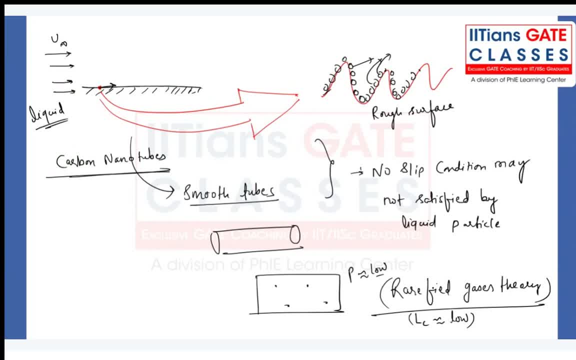 We are taking a very, very small length scale where we are analyzing our what Motion of the fluid right. So what will happen? Whatever the lambda will be there that is large as compared to LC in this case right. So concept of continuum. 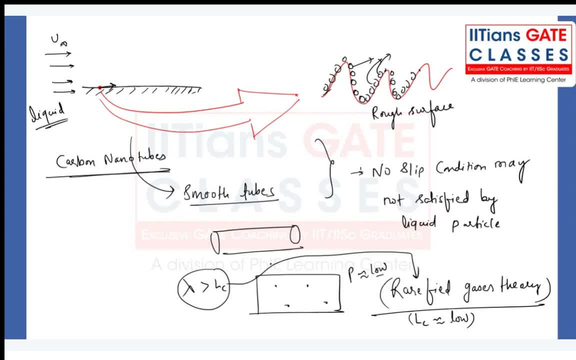 The concept of continuum. The concept of continuum will also be not satisfied, as well as whatever the no slip condition is there, that will also be not satisfied. Getting my point When I will discuss about the viscosity region in case of gases, right? 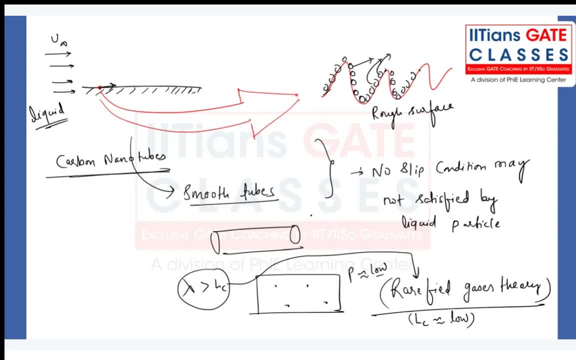 Why the gases do have the viscosity. then this picture will be more clear. which I am talking about: the rarefied gases theory, right, Make a note of it. Once it is done, let me know. Can I move to the next one? 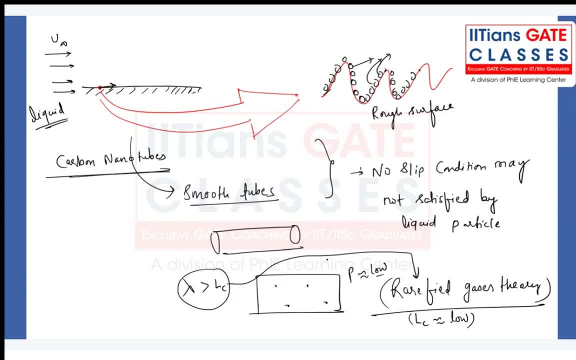 No, no, no, no. it is a completely fluid property. Remember: viscosity is a fluid property. We cannot change in any circumstances by changing the flat plate conditions, and all Viscosity cannot be changed. Why, Why Now? 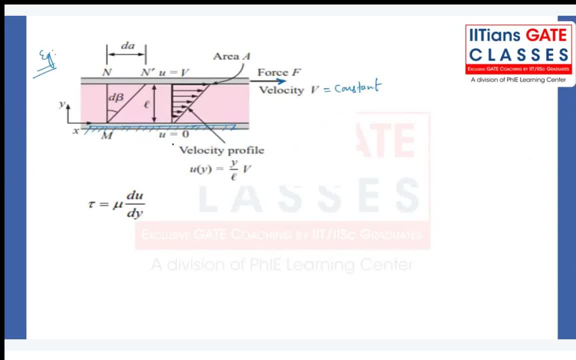 And here also my difference. if velocity of the plate is zero, the velocity of the fluid particle is zero. But why the fluid particle is having same velocity Once again here, Once again here. Because to satisfy, no slip condition To satisfy. 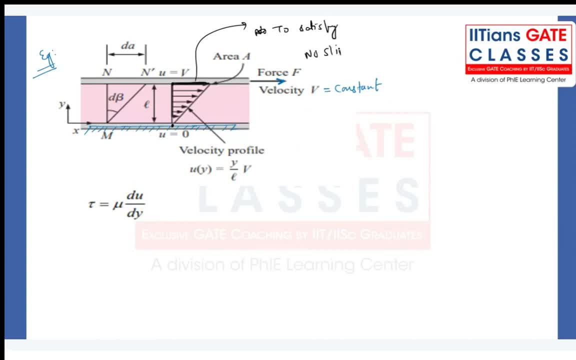 Once again, no slip condition. To satisfy. once again no slip condition. the velocity of the fluid particles will be higher, With having exactly same as velocity of the plates, so that the relative motion once again 0, right, Make a notice of it. 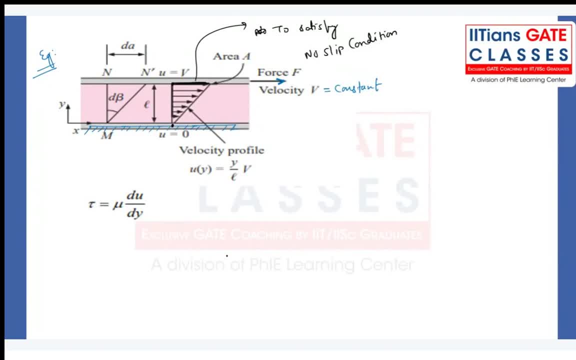 Right, Very, very smooth surface. Yeah, Viscosity You cannot change in any negative condition or maybe normal deep conditions, right. The nature of the fluid, that which can communicate to the Lok Dan, that can be deviated, right. but the fluid property, that is a viscosity that cannot be changed. 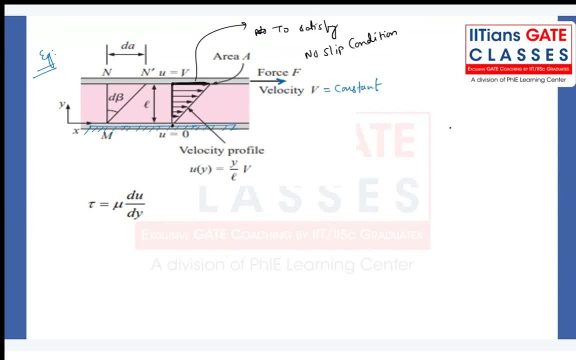 means if we, if we say viscosity of the water, uh, let's say any value, is there 10 power, 5 minus 5 pascal, second right, for example. then, for example, if i talk, then in any circumstances, whether water is flowing in a normal tube or in a very, very smooth carbon nanotube, that 10 to the power. 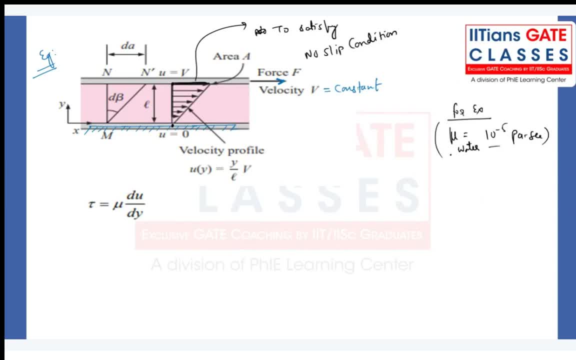 minus 5 pascal. second will not change. that value will not change, correct? you may be thinking about the viscous forces. yes, that can be having certain changes. right that that is correlated by the newton's law of viscosity. that is our next segment now make a diagram of this, make a note of it. 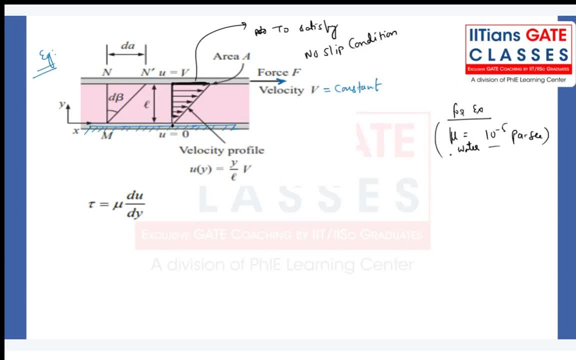 correct. correct. velocity gradient will differ. you now velocity profile. it can be parabola, it can be linear, it can be cubical parabola, it can be anything right. but the main important thing is that the velocity gradient, this one, this is called velocity gradient, right. 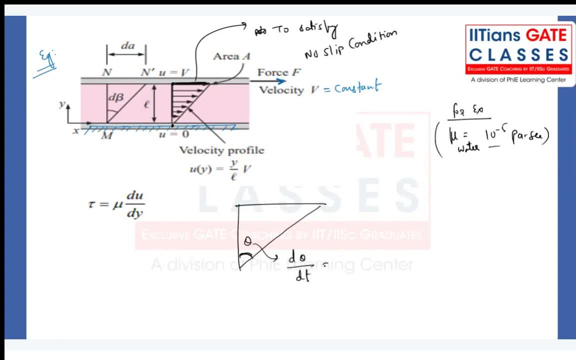 in a fluid term, if i say this d theta by dt, we also say: suppose this is v. this is for example the length, the gap between the two plates l right. so d theta by dt will be equal to du by dy. and how it is that we will prove in our 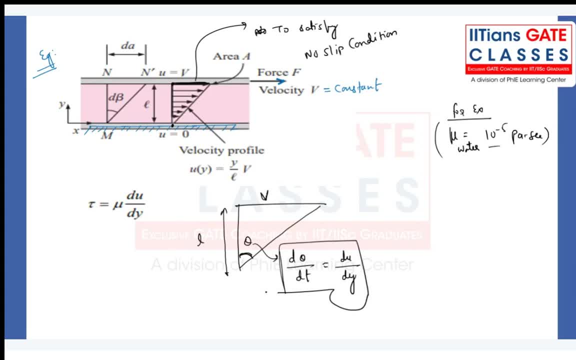 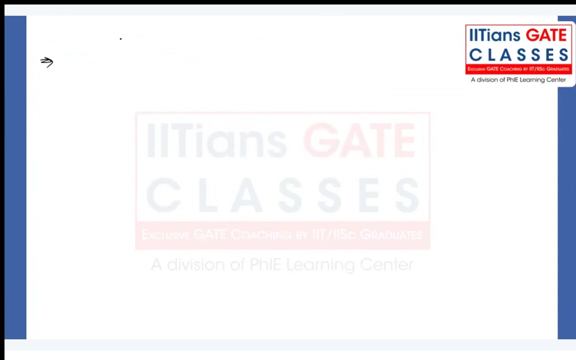 next page, all of you just note down. then we will discuss now my different, trying the stunning here. if you say, if you just talk about the situation, this is the my flow directions, this is my flow direction, this is my flow directions right in this flow directions, in this particularly flow direction. 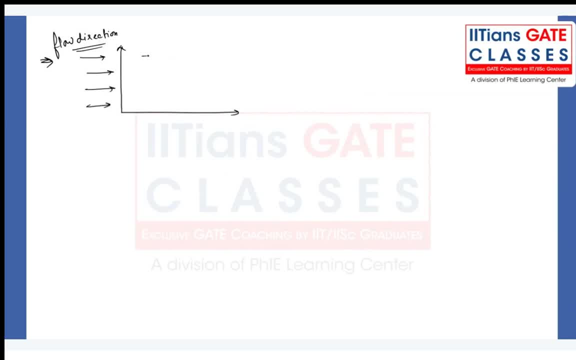 we have many fluid layer. right, we have many fluid layer, but i am for consideration. i am just taking four fluid layer, for example. right, and the first fluid layer which i am just talking about is moving with some velocity u, plus du. second fluid layer is moving with some velocity u and there is a some kind of 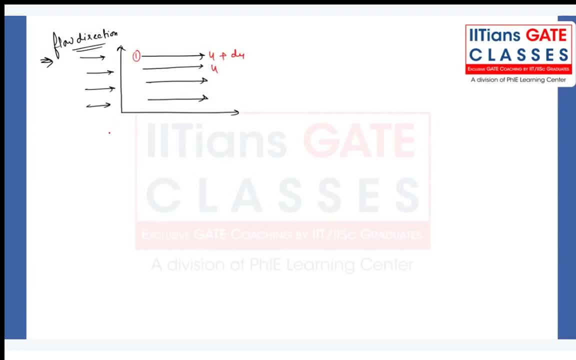 relative velocity, what we are observing right at a certain distance. second particle is being considered right at certain distance from the fixed wall. i am considering the fluid layer which is moving with some velocity u right and at a certain distance. particle layer at a distance y, which is having the velocity u Getting my point- And at a distance. 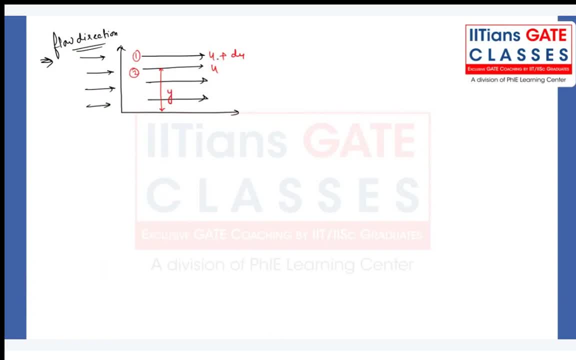 y plus du, at a distance, y plus du, I am having first fluid particle y plus dy, right, My dear friend, in a dt time interval. in dt time interval, in a particularly dt time interval, what will happen? The first fluid particle, which I am just composed of this one, the fluid particle, 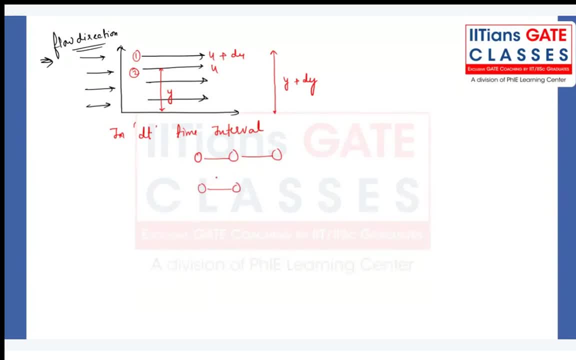 will travel? how many distance? What will be the distance that will be covered? u dt, that is the distance that is being covered by the second fluid layer. right, This is the second fluid layer. This is the first fluid layer. What is the distance? Velocity into time. right, The second fluid. 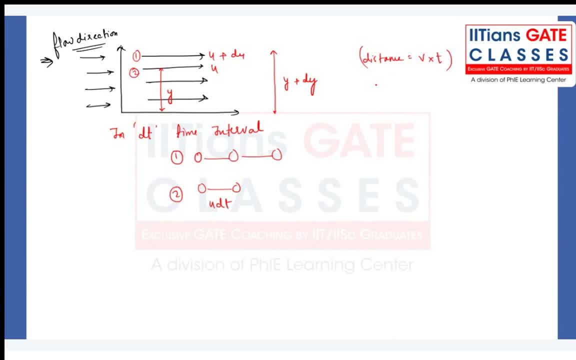 particle which is being traveling at a velocity u in a dt time it will travel. how many total? how much distance u dt? right? First fluid particle not only travel u dt, it will also travel another distance, du dt. Getting my point. So what is the total distance? 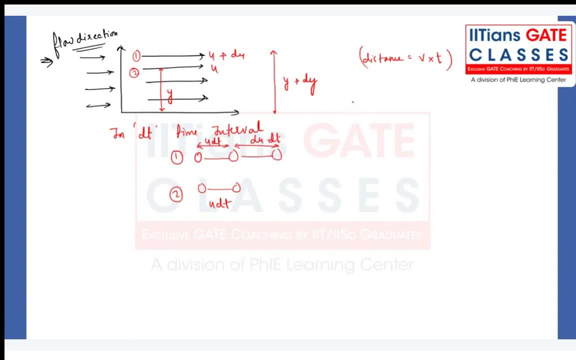 which is being traveled by the first fluid layer, u plus du, into dt. Getting my point? Is that clear? all of you? Tell me, guys, So when you join this one, my dear friend, what you are observing. What you are observing, my dear friend. 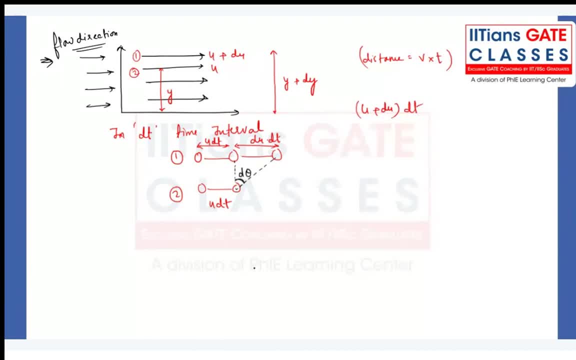 If I talk about this is a d theta, if I say this will be d theta, then what we can say, Then what we can say, my dear friend, Tell me guys, If I right tan theta, then what we say tan d theta will be what du dt divide by dy right. 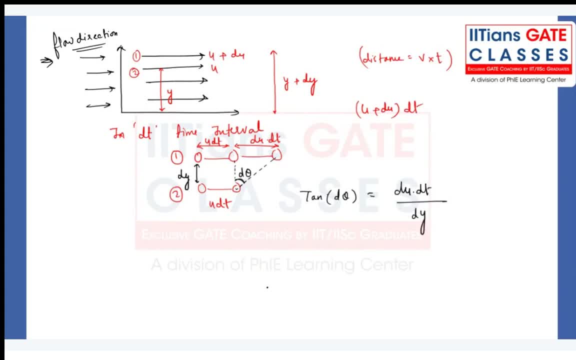 Can we write like that? Good, Now, if d theta is very, very small, d theta is being very, very small, d theta is being a very, very small. so what we can write, tan d theta will be approximated as d theta. 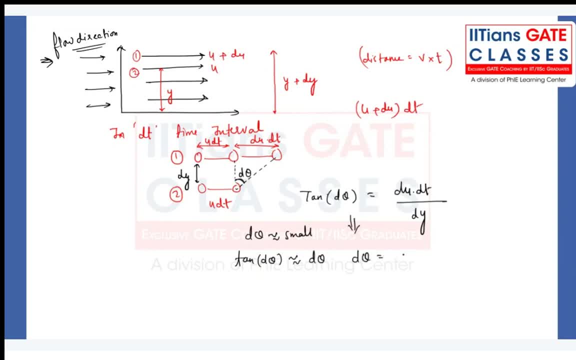 This can be written as d theta, that is equal to du, into dt divided by dy. So d theta by dt, that will be du by dy. Make a note of it. So what you are observing, rate of angular deformation, what we call rate of angular. 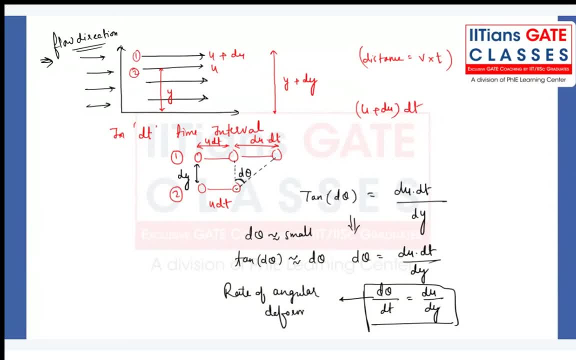 deformation will be equal to velocity gradient in a transverse direction. velocity gradient in a transverse direction, in y direction. Make a note of it Sometime, my dear friends, sometime, right in a solid mechanics, when you just apply this, 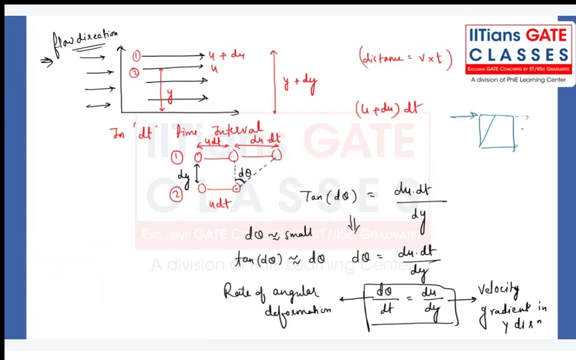 air force it will be basically getting deformed and that deformed will say shear strain In a fluid. we will say that, not shear strain, we will say shear strain rate. So sometime we used to write d gamma by dt, that is equal to d. theta by dt, that is equal 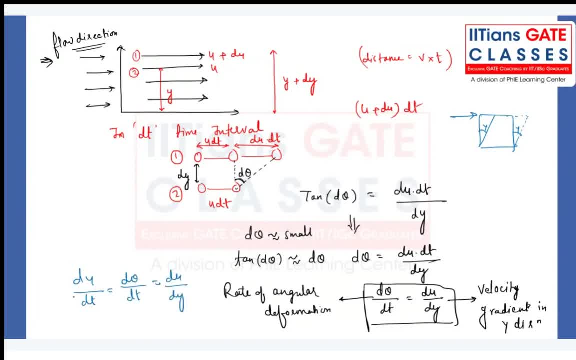 to du by dy. All are same term. Make a note of it. It is just like I told you in a first class you just consider a fluid element. You just apply this air force. The moment you apply this air force, it will continuously deforming. 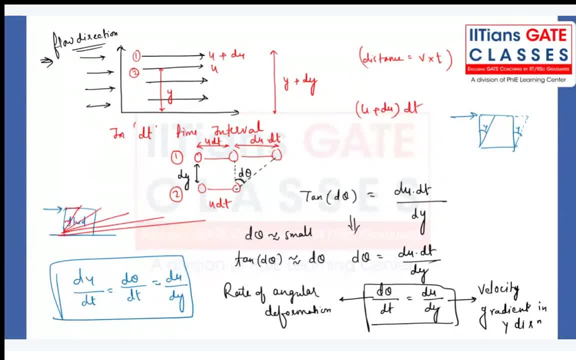 Continuously, it will deform That deformation. you know that deformation depends on the, how large the air force you have applied That deformations, that deformations. Make a note of it, Thank you, Bye, Bye, Bye, Because you will always have the velocity profile. 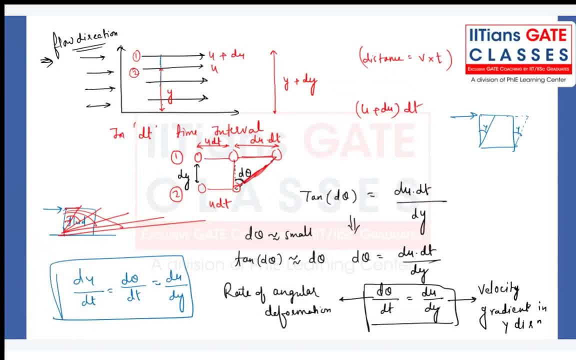 Maybe something like this, Right, So maybe you can think of. you may have considered this two-layer- and I have just taken the zoom of that- like this, Okay, Where this one is being a fixed one and may be above fluid layers, Okay. 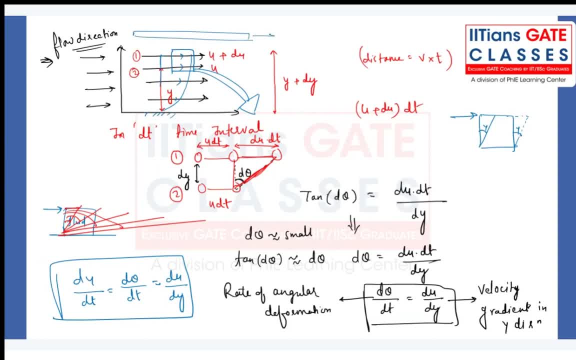 having the certain velocity. v See in my classes, my different- you have to bear with the some kind of derivations, because without derivation you may not be feeling about the subject right. Only solving the numerical. we can finish the numerical in one class. 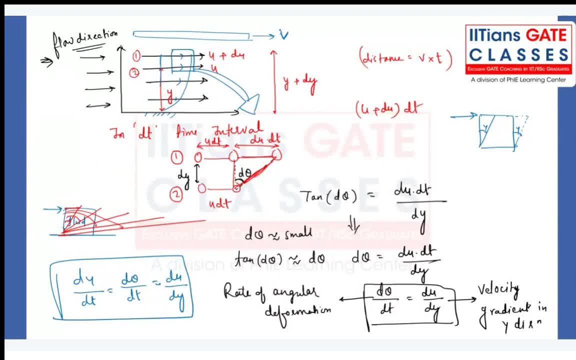 But the main thing is that we have to understand very carefully each and every topic Because, gate examination, we cannot expect that a very easy thing will be coming, that we already learnt right Now: du by dt. what is that? Now? that is the acceleration, you know. 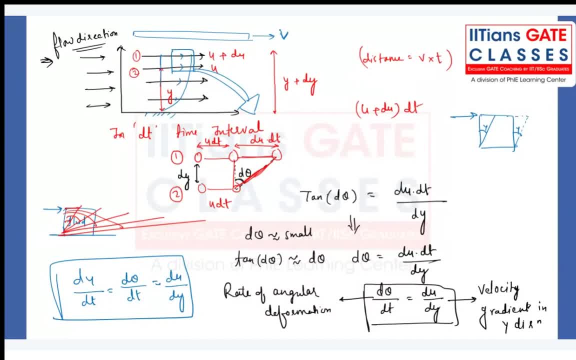 That will be the acceleration. That will be the acceleration. That is the velocity gradient du by dy with respect to Y-axis- Remember with respect to y-axis, not with respect to x-axis. Remember that Share strain, Share strain. We also represent gamma dot. 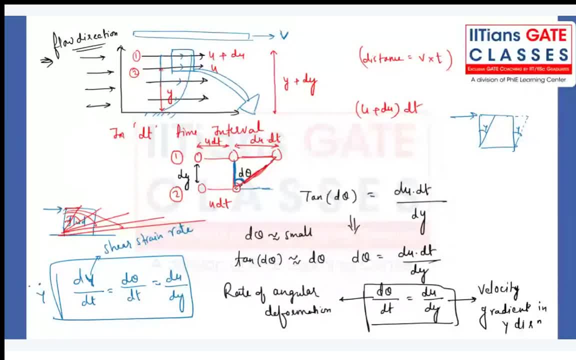 We also represent gamma dot. Now let us discuss about gamma dot. Okay, Okay, Okay, Okay, So sorry, So, ah, the concept of Newton's law of viscosity. Anyone know about that? One dimensional flow: Yes, 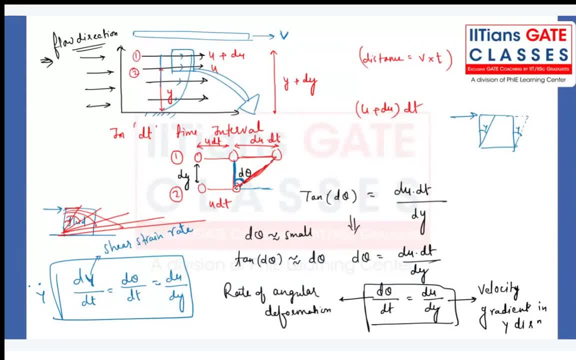 We are talking about the one dimensional flow, because two dimensional flow, when you think of basically, we cannot think of that situation right? Because see, the fluid particle is flowing like this right And fluid particle cannot penetrate right in this direction. Velocity has to be zero. 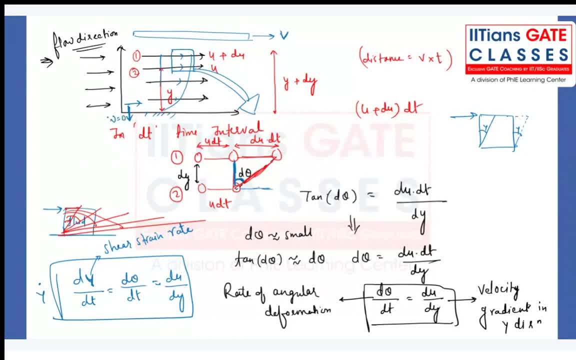 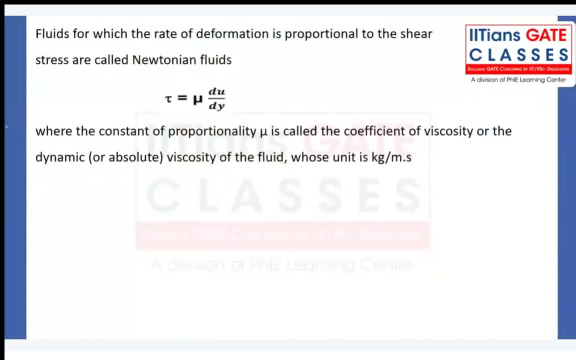 viscosity has to be zero And fluid particle cannot flow perpendicular to the plane of the laptop board, right? So once again, that is zero. So in a one directional flow we are considering right Now, think about the Newton's law of viscosity, The fluids for 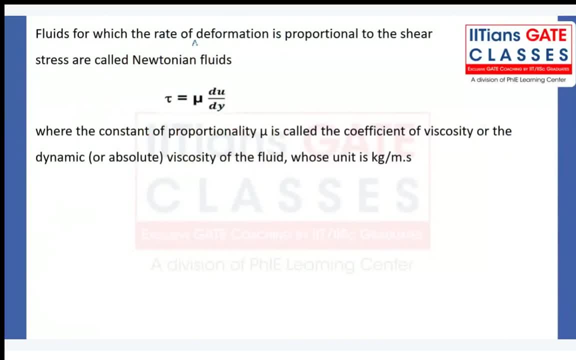 which the rate of deformation, which kind of deformation, angular deformations- is proportional to the shear stress, are called Newtonian fluids. The fluids for which the rate of angular deformations are directly proportional to shear stress are called Newtonian fluids. right Here only. 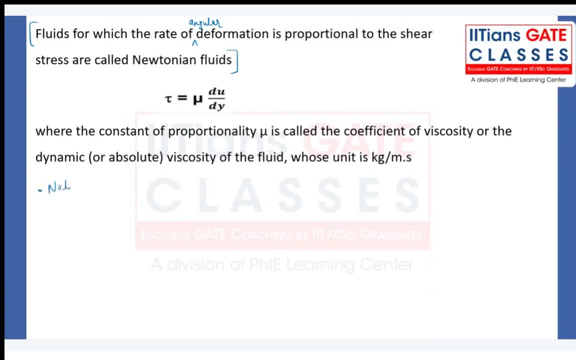 you just make a note of it, Newton's law of viscosity. It is a very, very important law. According to this- first let me read out that statement- According to this, particularly Newton's law of viscosity, my friend, the shear stress- remember, shear stress at a distance y from a fixed wall is 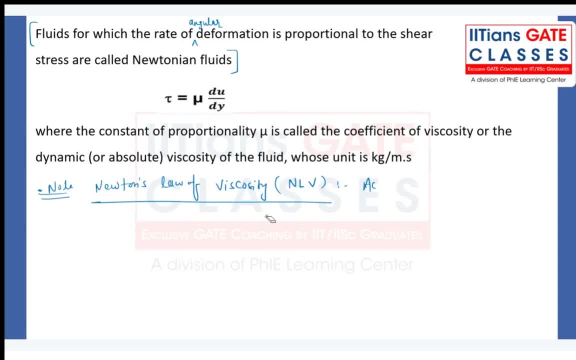 directly proportional to is directly proportional to the shear stress at a distance y from a, directly proportional to the rate of angular deformations or rate of shear deformations, or the shear stress will be directly proportional to velocity gradient in the transverse directions. So make a note of it. 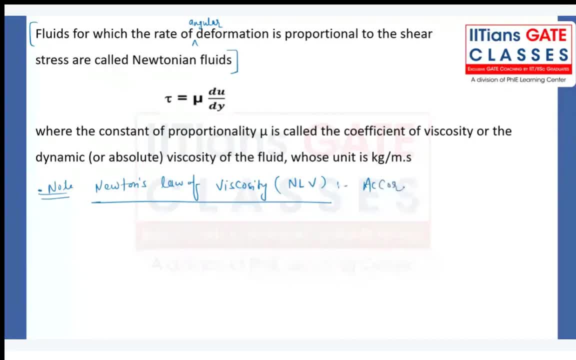 According to this, shear stress at a distance y from a fixed wall is directly proportional to is directly proportional to rate of angular deformations. The rate of angular deformation might be different. Make a note of it. It is a very, very, very, very, very important. 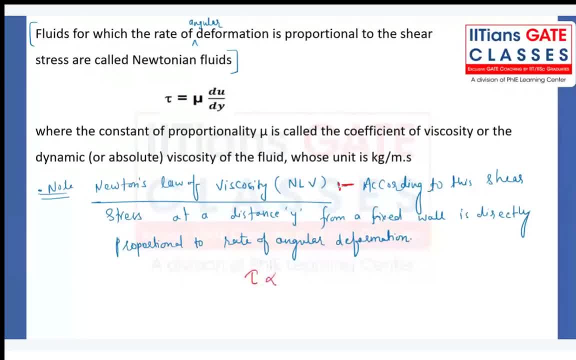 That means shear stress will be directly proportional to du by dy, Directly proportional to the angle of deformation, Directly proportional to the angle of deformation Directly proportional to d theta by dt. Directly proportional to d gamma by dt. Here important term is what? 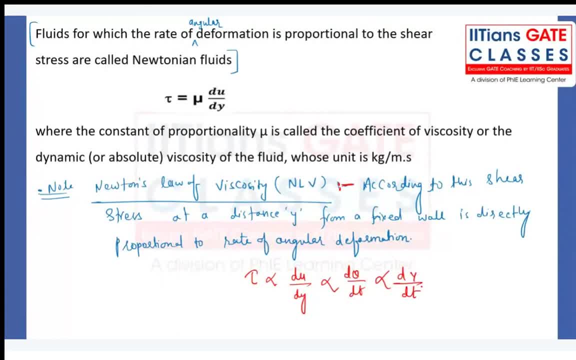 Dt Per unit time. Fluid is always represented per unit time In solid. there is no rate of that because there is no continuous deformations. There is a fixed deformation, So we will not take per unit time in case of solid. 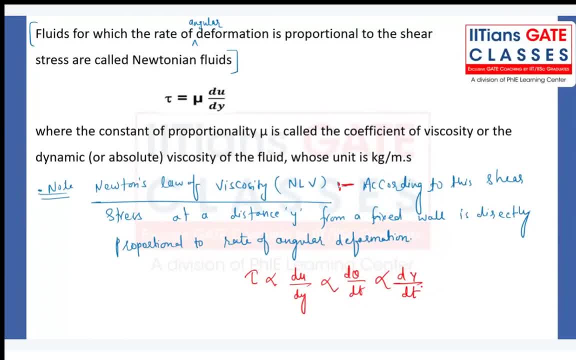 This is a very, very important. Now, if I remove the proportionality, I will be getting one proportionality constant. That proportionality constant will be called as viscosity. We also call dynamic viscosity. Now, make a note of it. Now, make a note of it. 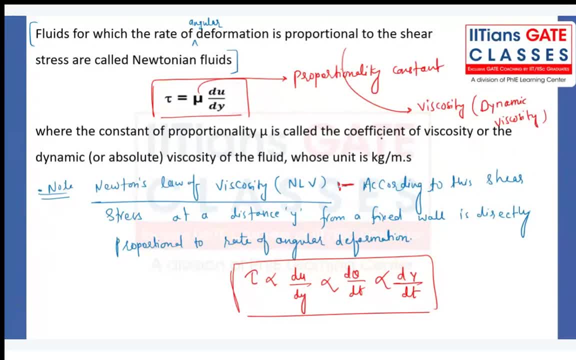 We also call coefficient of viscosity, Absolute viscosity Or simply the viscosity. Whenever see we have the two viscosities. Whenever see, we have the two viscosities. One is a kinematic viscosity, Other is dynamic viscosity. But whenever in the question they have given only viscosity. 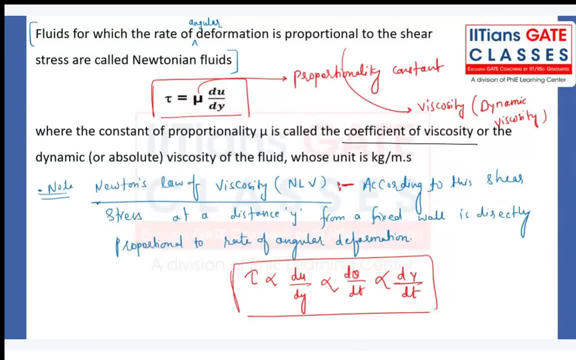 Remember that they are talking about dynamic viscosity directly. They are talking about the dynamic viscosity directly. Now let us see the unit of dynamic viscosity All of you have noted down- And the fluids. Remember the fluids, The fluids which follow the Newton's law of viscosity will be called as Newtonian fluids. 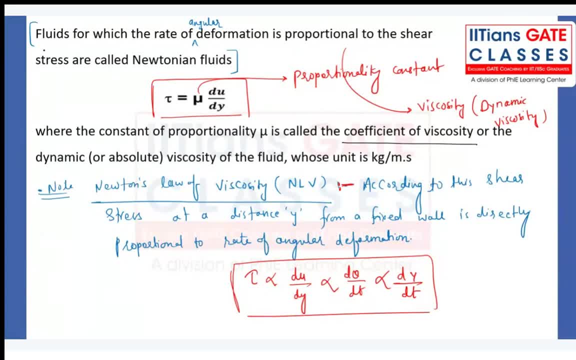 Because the definition is quite similar. You know, The fluids for which the rate of angular deformation is proportional to shear stress will be called as Newtonian fluids. What about the fluids which do not follow, or which does not follow the Newton's law of viscosity? will be called as non-Newtonian fluids. 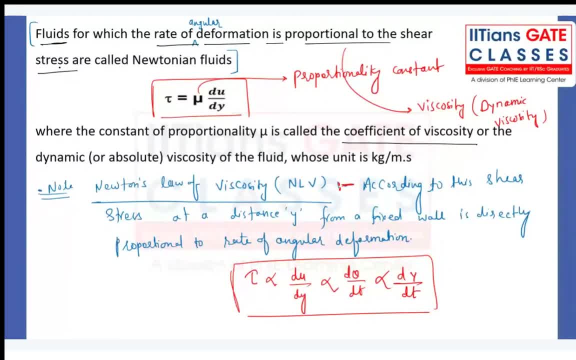 Right Will be called as non-Newtonian fluids Right, So we will write Newtonian fluids. Good, Make a note of it. I have done that over and over again. 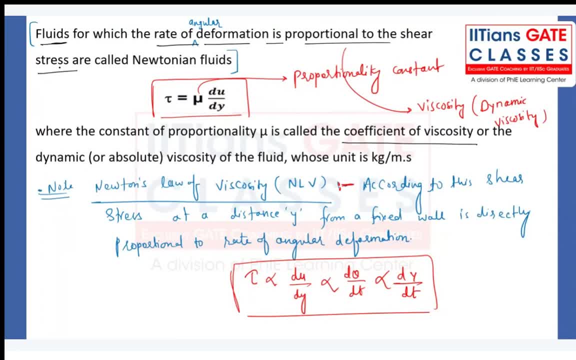 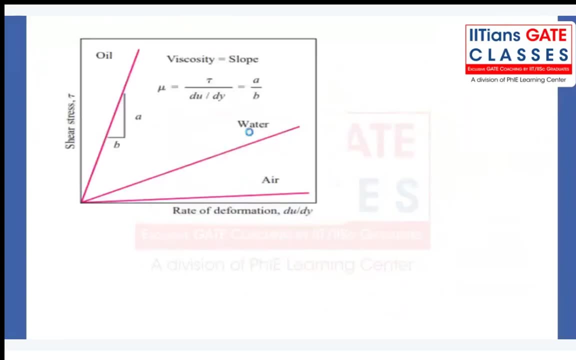 all of you have noted down. is it done for all? can i go to the next segment now, my different? if you just talk about the unit of viscosity, yeah, this is only the reason that they do not follow the newton's law of viscosity. 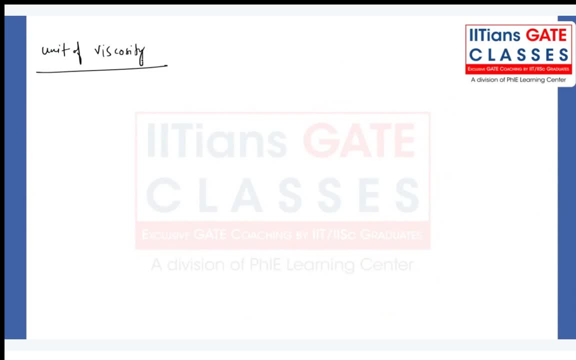 because the branch of science in which we deals with the types of fluid, we say rheology. in that rheology we deal with the newtonian fluids and we also deal with the non-newtonian fluids. now, unit of viscosity, when you just think of tau, is what mu uh du by dy, right, mu du by dy. now, when 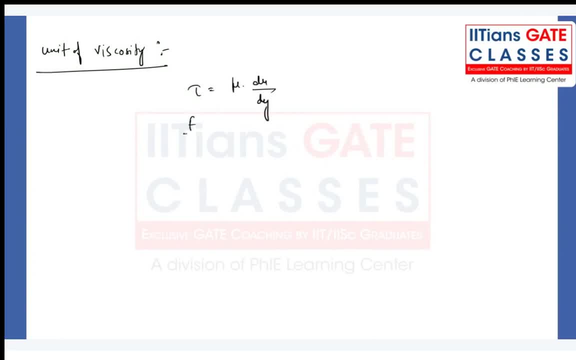 you think of cell stress, that is, a share force divided by area, the air force divided by share area, right area, on which that will be acting. you know, the shear distress will be acting. so that is a mu into du by dy, for example. for the time being i'm assuming linear velocity profile. 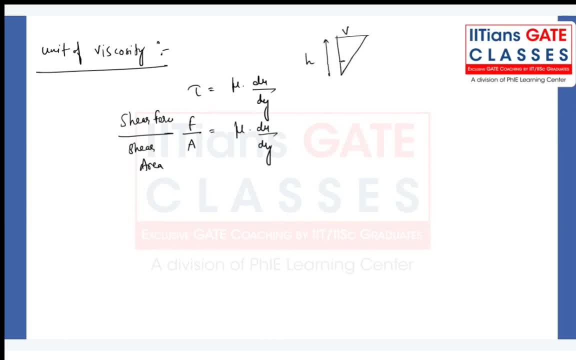 linear velocity profile. then what about d, theta by dt, my different, this slope? this slope will be what du by dy, that will be v minus 0 divided by h minus 0, because this will be y and this is being 0, the reference one. right then what we can write, v by h. so force by area. 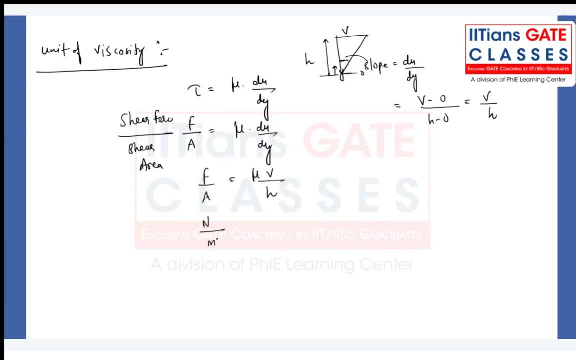 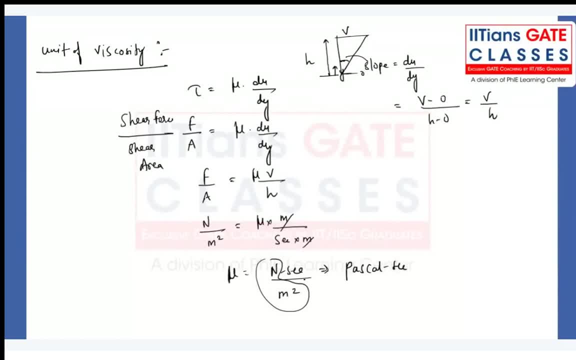 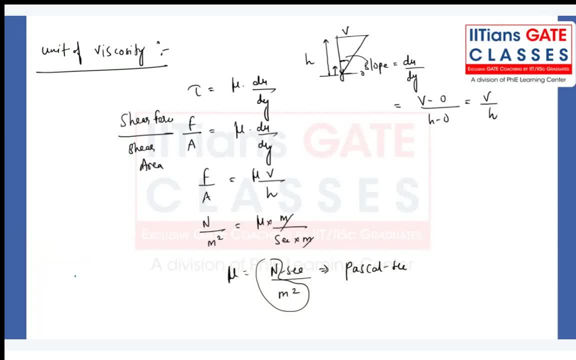 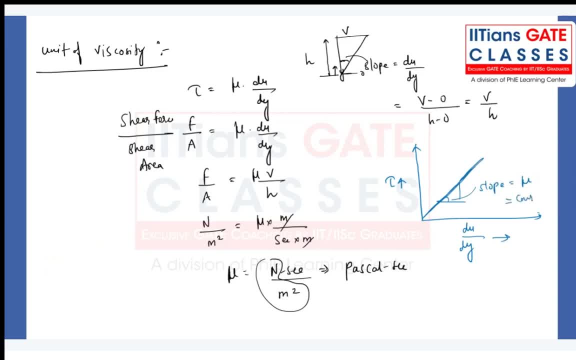 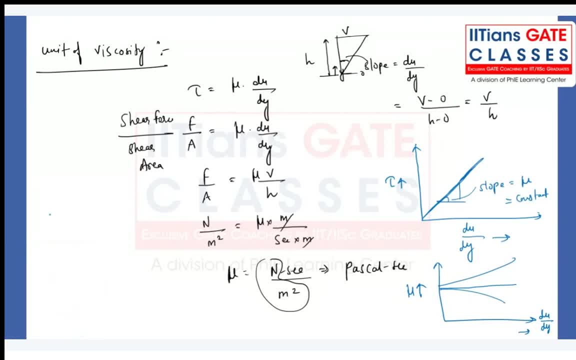 The viscoelastic fluid will be what see? it will follow like this. then what will happen? Tell me guys, I will discuss. I will come to that viscoelastic. Let me discuss first of all the unit of this. let me remove this part. 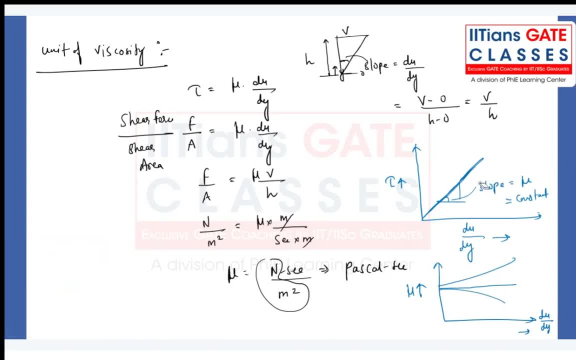 We have the types of fluid flow there. I will discuss ideal fluid, plastic fluid or maybe ideal fluid. what about the ideal solid? what about the viscoelastic fluid? all those things will be coming there. Now see, when you just apply this shock load, you know certainly what will happen. 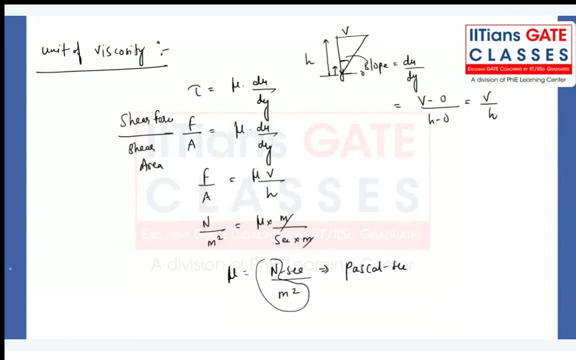 Environment changes will be happening, you know, because shock will happen. why the shock will happen? Tell me guys, there is a certainly uncertain conditions will be there where the pressure might have changes, or maybe it is being passed through a very, very, you know, sharp cross-sectional. 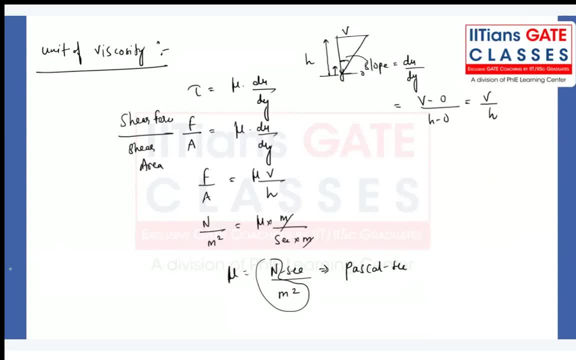 areas. you know in that particular case what will happen. or maybe it is flowing in a divergent section where the large divergent angle is there right, where the flow suppression is quite high. there the shock will be happening, right. 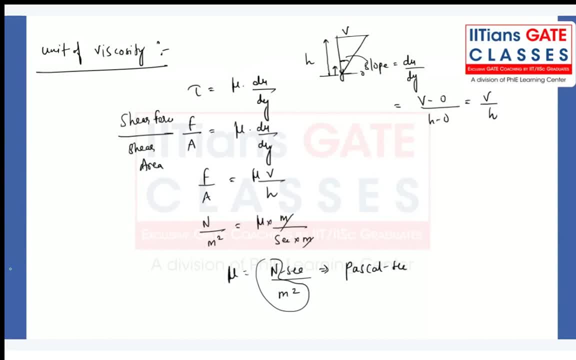 Okay, And in that case, whenever the shock will be happening, shock loads will also be acting. In that case, it is a hypothetical thinking that the Newtonian fluids might be think like a solid one, but it is absolutely true? I don't think so. 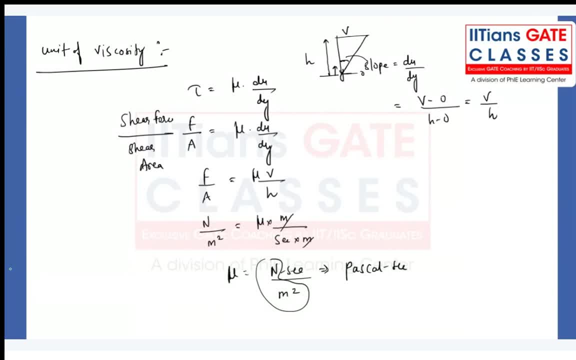 Getting my point Now here, when you just think of a unit of viscosity in a dimension format. so what will happen? What will happen Here? mu can be written as tau divided by mu, du, by dy, for example, And we can also think of: sorry, we have already taken mu left side. that is a force per unit. 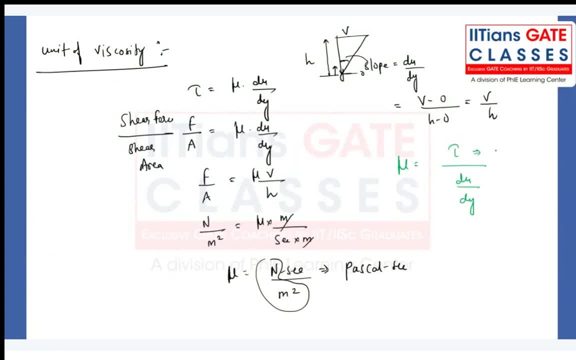 area. right force per unit area. Now that will be being discussed by aerodynamic faculty right. that I am not discussing right now, right Now here, because that is a… Don't think that… What we are discussing… 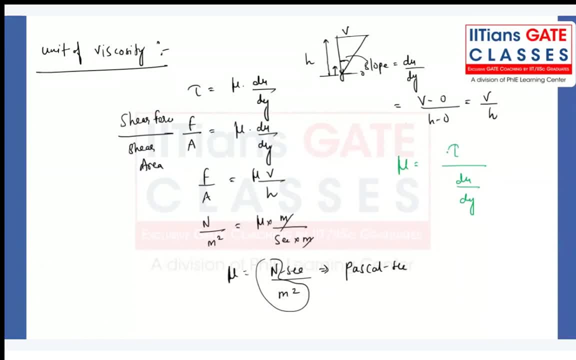 It is completely related to that because to have a clear background, if you want to discuss shock load and all, I need to give you a brief history of that. you know background of that directly. I cannot discuss getting my point. 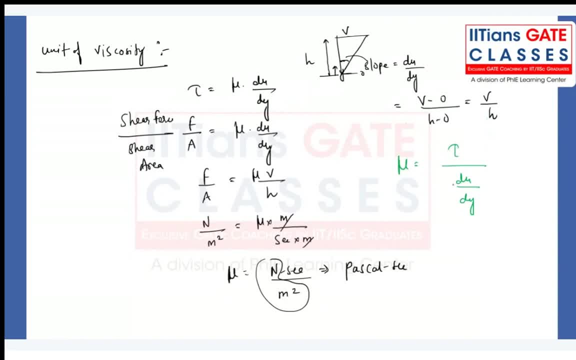 Now here, what is that force? what are the force dimensions? MLT minus 2, right, And what about you say the area meter square? so what you can have. MLT minus 2, right, And what about you say the area meter square? 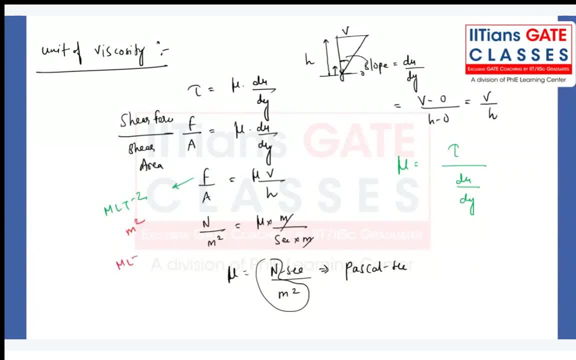 So what you can have: MLT minus 2.. MLT minus 2 divided by L square, so this will be ML minus 1, T minus 2.. This will be the dimension of, say, the stress: ML minus 1, T minus 2, velocity: this will: 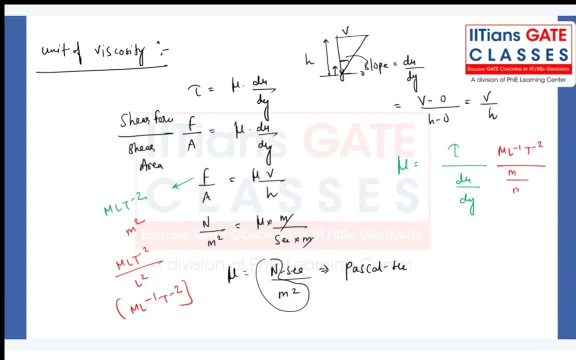 be what meter, meter you know, per second. this will cancel out. so automatically this will be second. so T will be multiplied once again. right, T will be multiplied once again. So finally, what is the dimensions of mu? 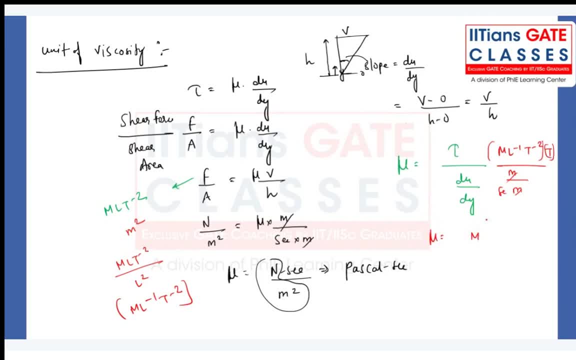 ML minus 1.. Right, Right, T minus 1.. T minus 1.. Make a note of it. Is that clear, all of you? Tell me, guys, Is that clear? Now, what is the other unit of that? 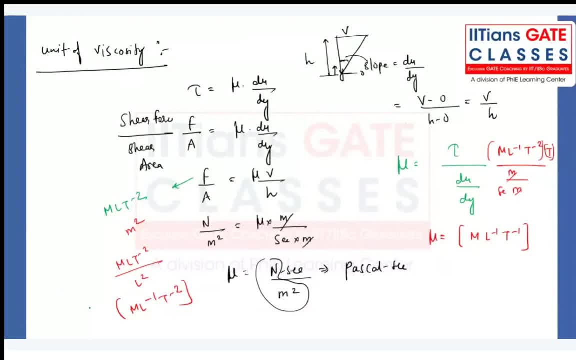 What is the other unit of that, apart from the Pascal second, Apart from the Pascal second? Remember this will be SI unit. Remember this will be SI unit. But if I talk about the other unit, maybe CGS unit, or maybe if we just talk about the 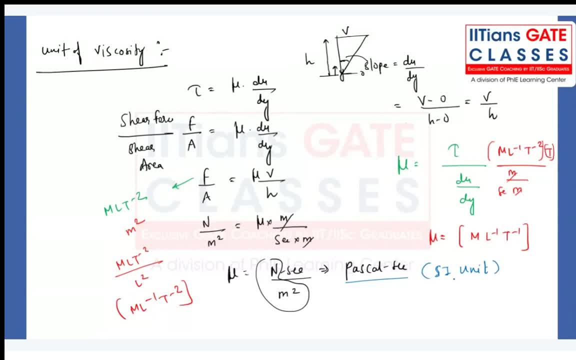 other SI unit. then what we can write. Then what we can write: See, that can be think of what we say, mu right, mu can be think of kilogram, because that is force per unit area. Force is what. 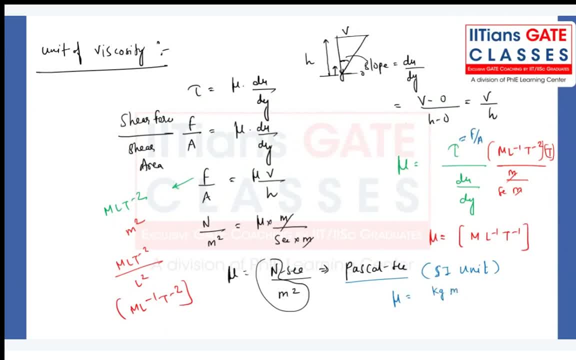 MG Or mass into acceleration. Kg meter per second. square kg per meter second, square right by meter, square 1 upon second right. So you will be getting what Kg per meter second? That is another SI unit. Make a note of it. 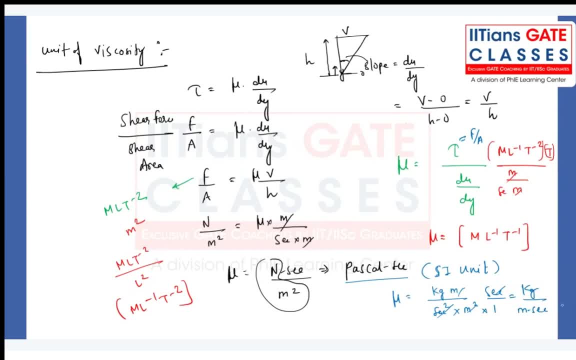 Now we have to discuss about the CGS unit of viscosity. What could be the CGS unit of viscosity? Let's discuss about that. Poise And 1 poise is what? 0.1 Pascal second, How? Let's discuss about that. 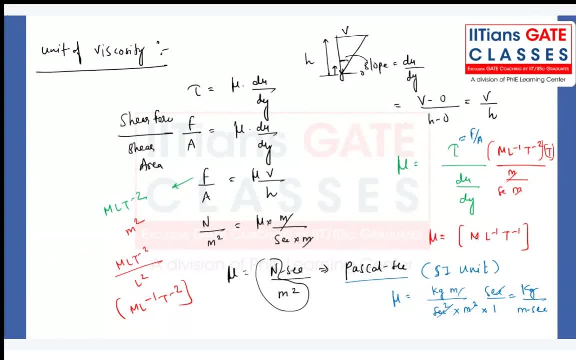 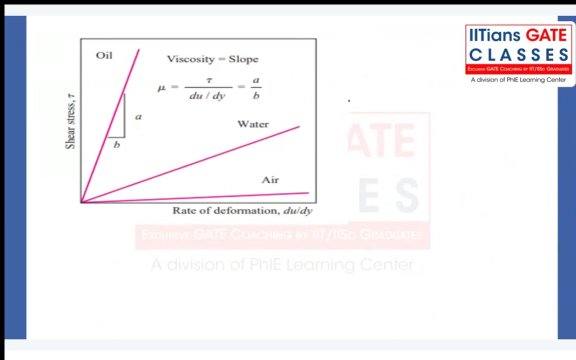 Is it done for all? All of you have noted down. Now don't draw that one. Let me discuss the CGS unit of make a note of it. The CGS unit of viscosity. Let's discuss about that. How, How. 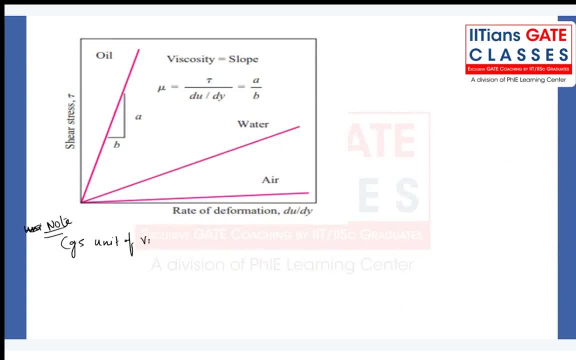 How, How, How, How, How much viscosity? Viscosity will be 1 gram. basically, if I just say gram per centimeter second, Gram per centimeter second Right, This is a unit of CGS unit. 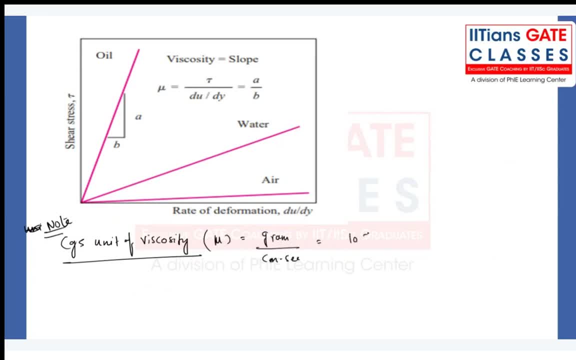 1 gram is what 10 power minus 3 kg. 1 centimeter is what 10 power minus 2 meter. So gram per centimeter, second meter and second. so when you just calculate you will be getting 0.1 kilogram meter second, or 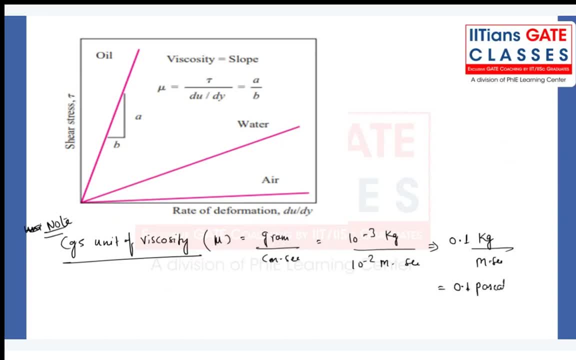 1.1 pascal second right. this will be called as one poise. this one you can write completely like this: one poise will be 0.1 pascal second. now guys, so we have discussed about the newtonian fluids, right? what are all the examples of? 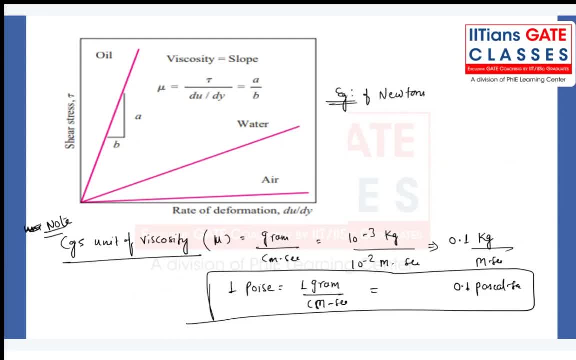 newtonian fluids. anyone know that? what are all the examples of newtonian fluids, my dear friend? the fluids which follow newton's law of viscosity, the fluids which follow which follows newton's law of viscosity, l, l, v, n, l v. newton's law of viscosity will be called as: 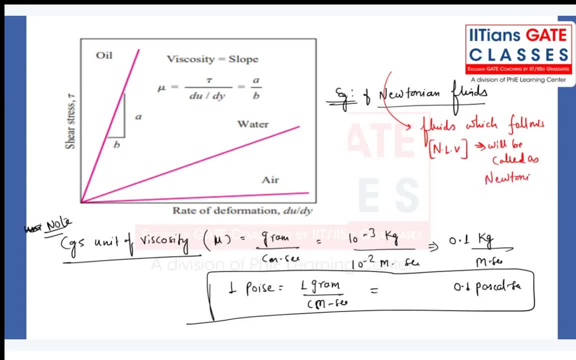 newtonian fluid will be called as newtonian fluids. what are all the examples we have here? the fluids which are considered as newton's law and the fluids which are considered as kind, and first, lungs will be actually cold. oraz this, this fluid has the unique characteristic l. if that, if it simmet bank. 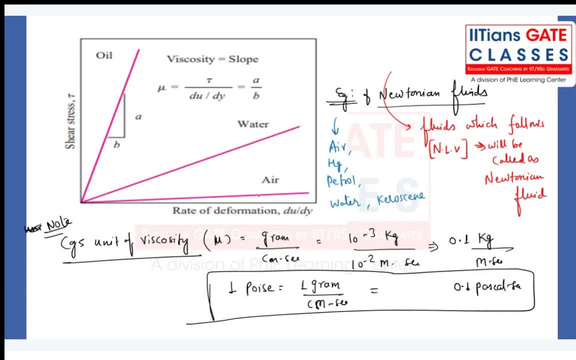 in in the y, e, d, n, v, f, c, z, l, n, i, f, a, y, v, you, you now, now, as you mentioned the honey one, you know, whatever the honey you mentioned, it tends to behave like a newtonian fluids, but there are certain conditions, right? uh, if, whatever the what we say, the honey, what it makes more, uh, what we say. 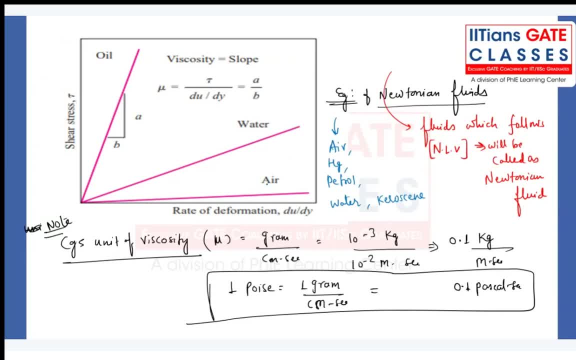 what about the ingredients of the honey? if you, if i ask you, what are all the ingredients or maybe content of honey that makes the honey more you know, sweetness, yeah, uh, sugar or what we say, uh, whatever the sucrose content, is there that that, if you want to have that, you know that should be at a very 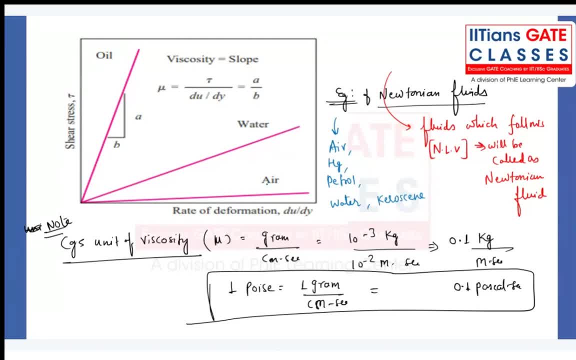 very high level in that honey right, because some honeys are there where we don't have that. uh, sucrose levels are low. right types of honey is there? so where the suppose quantities are more, or maybe sugar quantities are more, that will tends to behave like a newtonian fluids. but my suggestion will be: don't go. 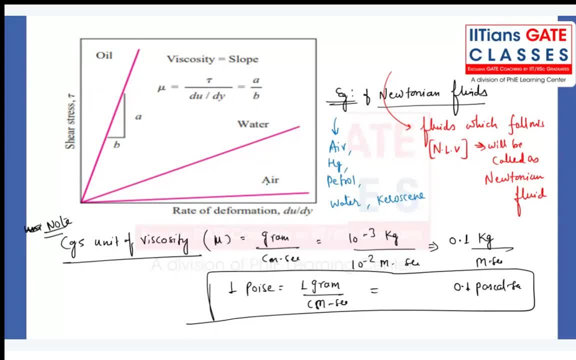 into the deep of that. that is absolutely not required for aerospace guys. it is important for the mechanical and chemical, but it is absolutely no. none of the uh basically use will be there for further right. so regarding particularly fluid, you just maybe, if you want curiosity, you search it right from the authentic sources. if you are getting the answer, it is okay. 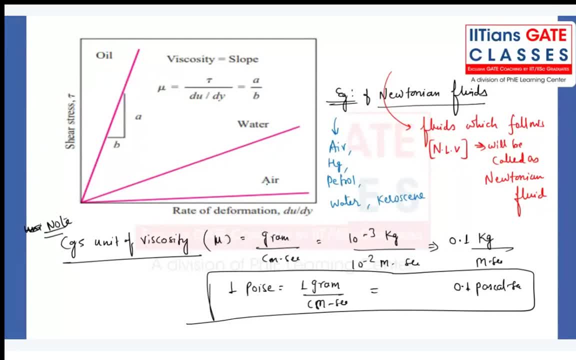 if it is not, then you can leave it, because whatever the exact newtonian fluids are there- i have given the example right air. we always, always see that surrounding airs, atmospheric air, that is the neutral fluids. right, that will not change its viscosity at any other circumstances. 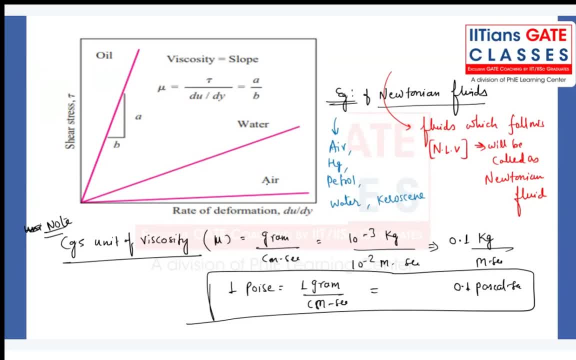 right Now. So when you think of shareless cloud, then which of this locations will you install? etcê are located intoать the사used became ideas from which Newton fluids, но nowulaing to put costs for cooling ion discharge to, how are you going to find? so we have that example, right: air. we always see that surrounding airs atmosphere, that is a neutral zone, right, that will not change its viscosity at any other circumstances right now. so 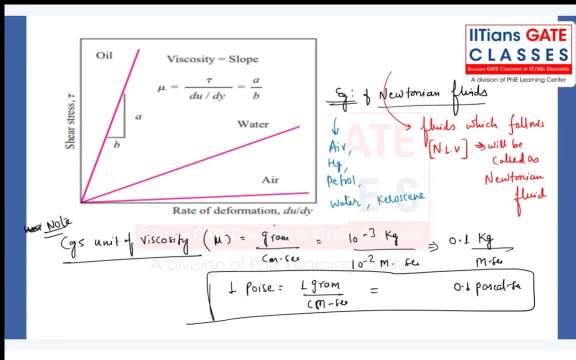 shear stress and the rate of deformations. we already seen that. What is that? The shear stress is directly proportional to du by dy, y is directly proportional to x And if I remove the proportionality I will be getting what y is equal to mx, the straight line. 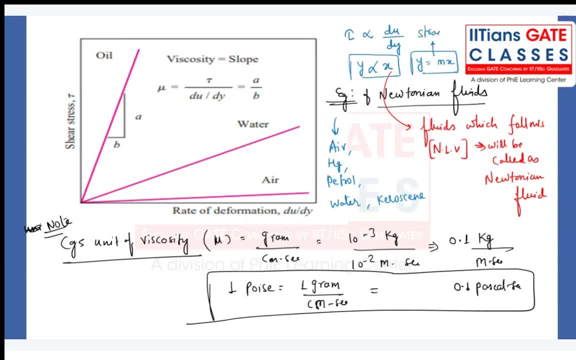 equation And that is what the straight line we have drawn And the slope of that straight line will be. the slope of that straight line will be viscosity. More the slope of that straight line, more will be the viscosity. So here for this example, what about the viscosity? 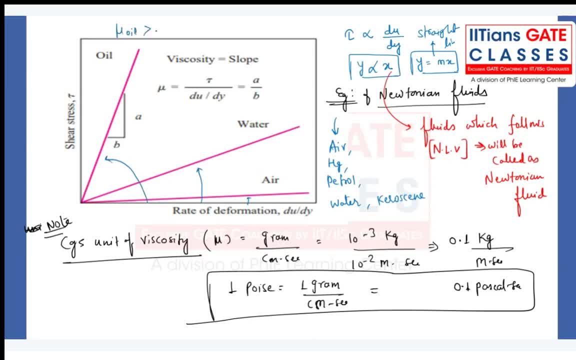 of the oil, Very large Viscosity of the water, then viscosity of the air. Make a note of it, Because whatever the viscosity is there, that theta slope is there. the slope is representing directly the viscosity If slope is constant. everyone know that if straight line slope, 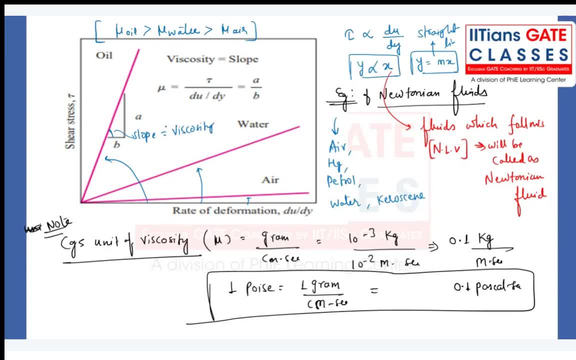 is constant, the viscosity will also be constant. So this is the straight line equation And if I remove the proportionality, I will be getting what That is, the quality of Newtonian fluids, Even though how large shear force or shear stress is being acting, even though continuously deformation is happening. but 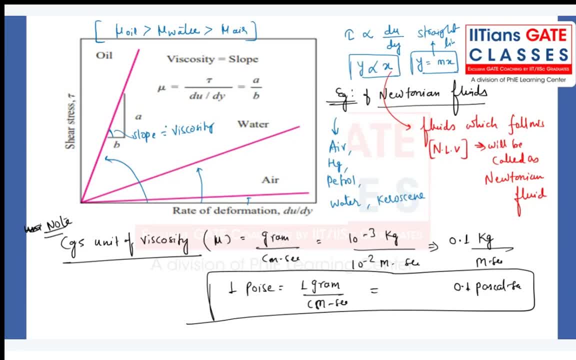 viscosity will not change, Tau will change, velocity gradient will change, but mu will remain same. If it is also start changing, if it is also start changing the viscosity of that fluid, that will be no longer Newtonian fluids, That will be called as non-Newtonian fluids. That will be called as non-Newtonian fluids. 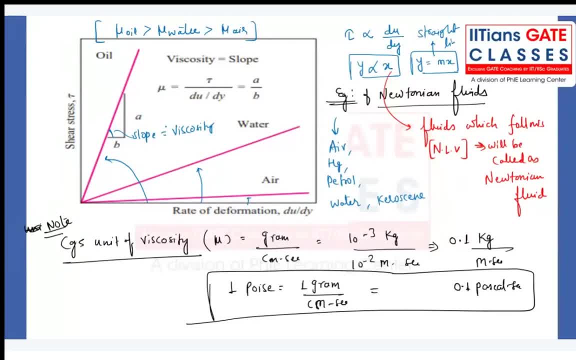 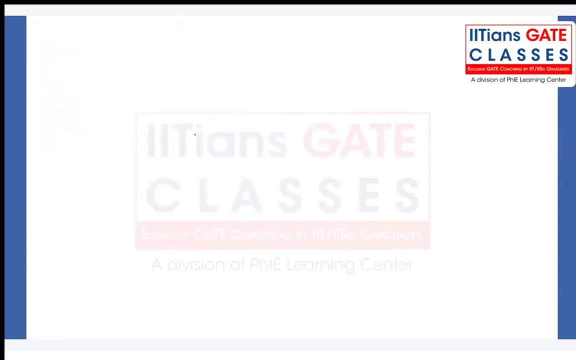 Now is it done for all? All of you have noted down Now, guys. so here I will be discussing types of different types of fluid, But before that, make a note of it: Newtonian fluids. What is happening with the Newtonian fluids? That, whatever the graph, 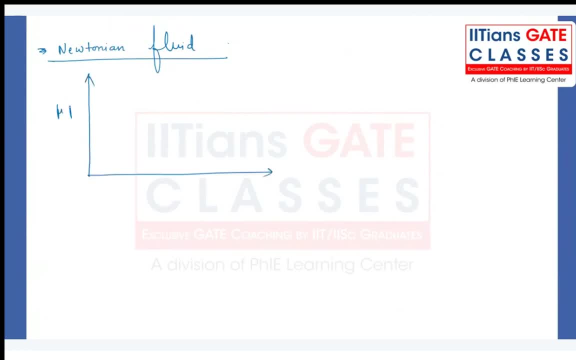 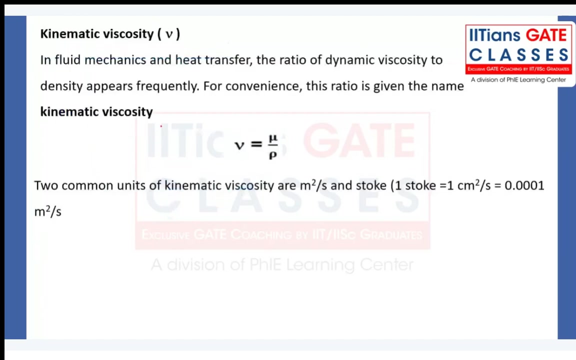 is there, you just make a graph of that. It will be having certain values that will be constant. Viscosity will remain same. It will be having certain values that will be constant. Now, guys, note down one more important concept that we will be discussing. make a note of. 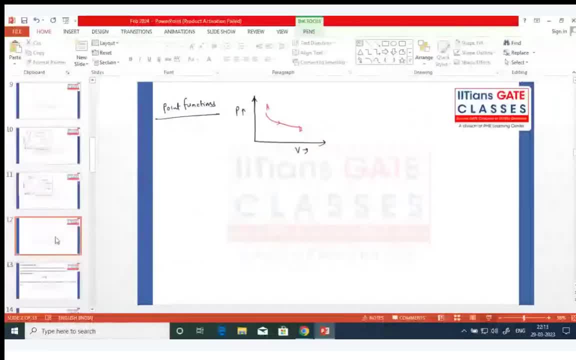 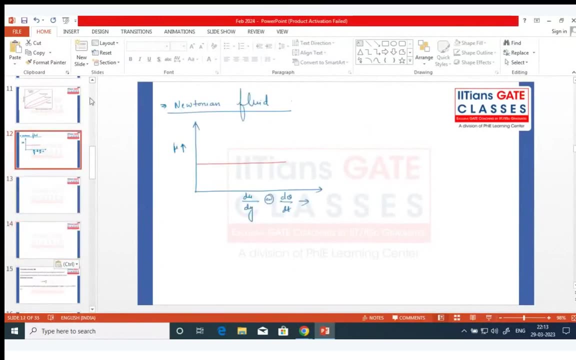 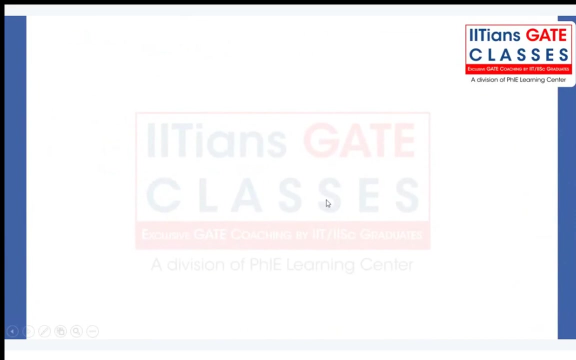 it all of you have noted down just a moment. is it done for all Over? Now, guys, try to think of certain situation which I am telling you. so, till now, what you have discussed, what is the physical significance of viscosity? 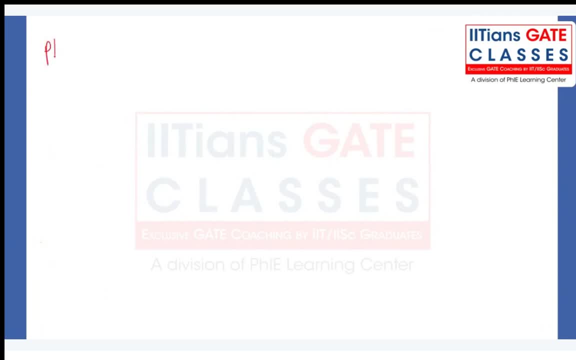 What is the physical significance of viscosity? Some of you might be feeling, sir, still I am not getting the feeling of viscosity, but viscosity before coming to your class, before coming to my class and, sir, after basically attending your classes and not before and after. there is no basically improvement in. 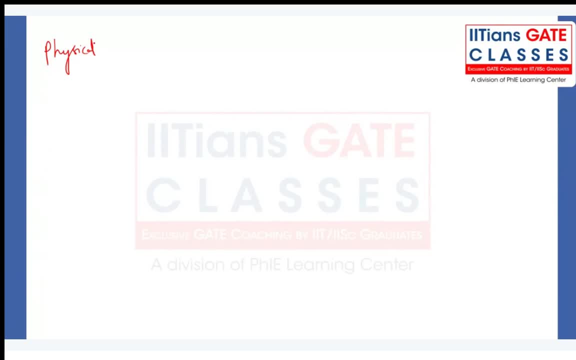 that my level of understanding. then there is no use of that. So let me give you physical significance of viscosity. So if I say viscosity is very, very high for a fluid, What will happen? We have the two fluid layers. suppose the plate is there, in which the plate is moving. 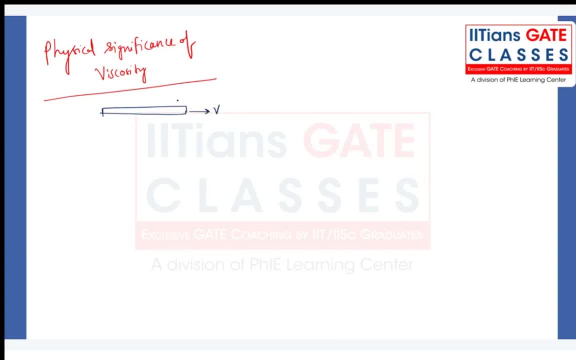 with the velocity v and that plate is moving by some force. right, definitely, there has to be some force and the bottom plate is fixed one. In between that, we have the fluid which is being flowing, not flowing, it is a basically what? static fluid. 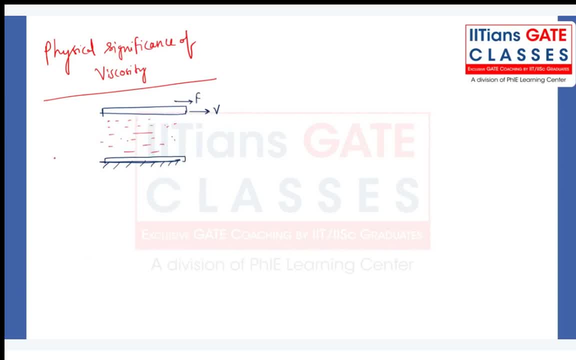 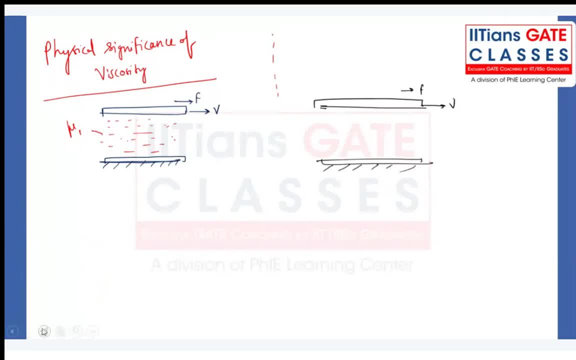 plate is fixed one, But now we have the fluid which is having the viscosity mu two. Mu 1 is greater than mu 2.. My defense tell me in which case the velocity will flow with more fluency. That means velocity gradient will be more indirectly. 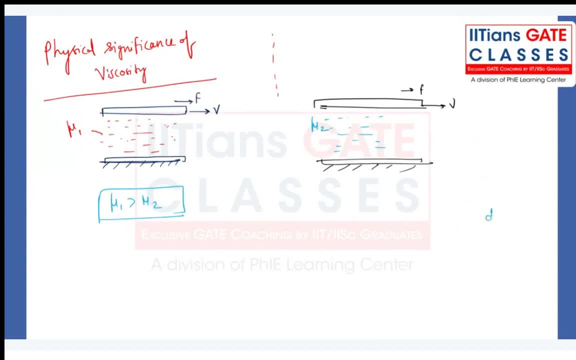 Remember, velocity gradient means flow only Right. So you think of in that scenario, So when the viscosity will be more in the first case, for the same shear stress, for the same shear force for the same plate of area A. 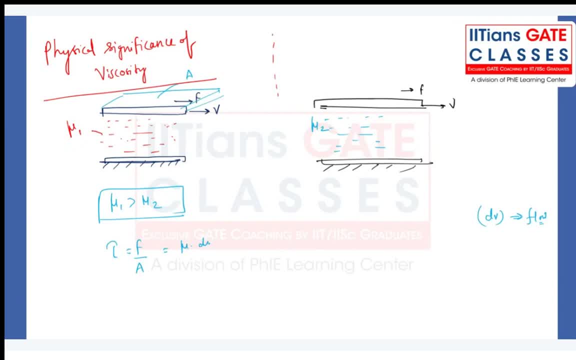 mu into du by dy Right, Then, for this being constant, let's constant will be k. Mu will be what k divided by du by dy Right. And, my dear friend, if mu will be more and more and more, then what about du by dy? 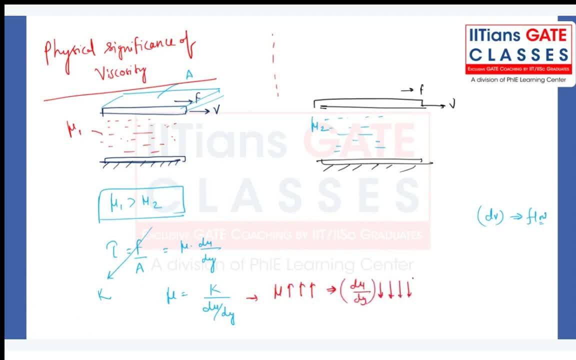 Will be less will be less, will be very, very less. Flow will not be that easy. Flow will not be That easy. That means we might have the cases where we can see the velocity profile, something like this: Maybe any velocity profile. 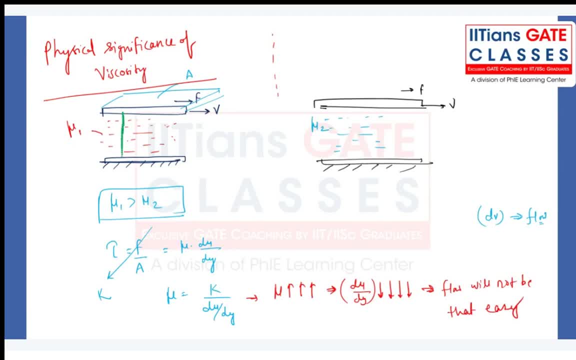 I am not talking about the linear velocity profile For the time being. for understanding, let's say, the velocity profile is linear one, Here also the linear one, for example. But you will observe that it will have something like this, But here you will find that this velocity gradient will be high. 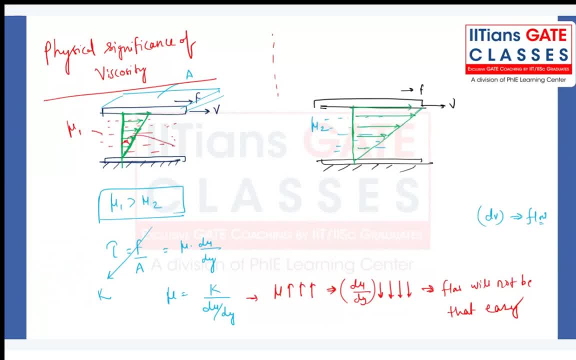 This theta will be high: Theta 1, theta 2. So theta 2 will be higher than theta 1.. If viscosity of one of the first fluid will be more than viscosity of the second fluid, then flow will not be easy. 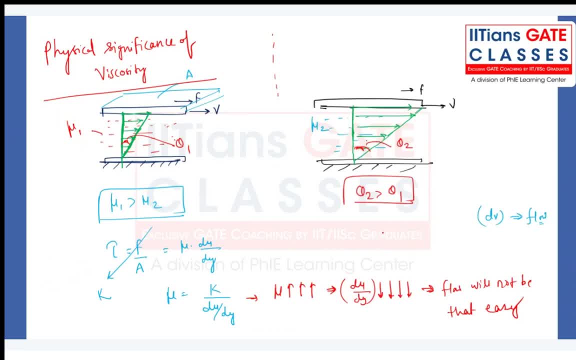 You only think practically. you know a lot of bondings are there in between the liquid particles, Right? So suppose you are talking about This fluid particle, first one and second one, What the communication will happen If you are moving with certain velocity. I will also move with somewhat same velocity as you. 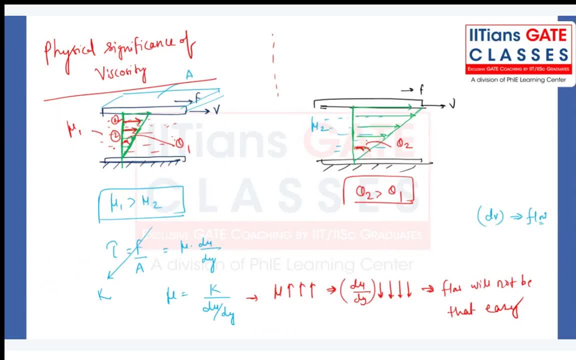 Because we have a lot of bondings, We have a lot of viscosity between us. But what about here? A lot of viscosity is not there, A lot of resistance is not there among the fluid layer. That's why there is a large relative velocity as compared to the earlier fluid. 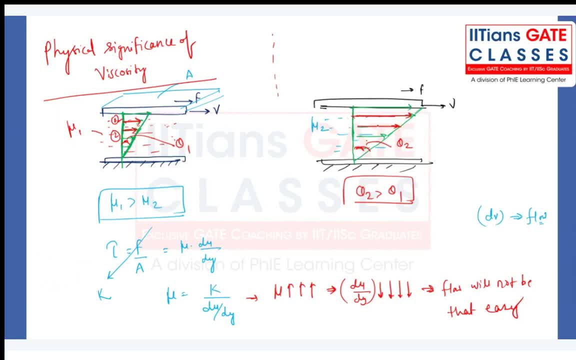 That is a form of fluids. So that's the physical significance. Make a note of it. Correct, That is what the reason of viscosity: in case of liquid, High cohesive force. But if, If you might think of, sir, if it is not the liquid, if it is the gases, then there is hardly any cohesive force between the gases. 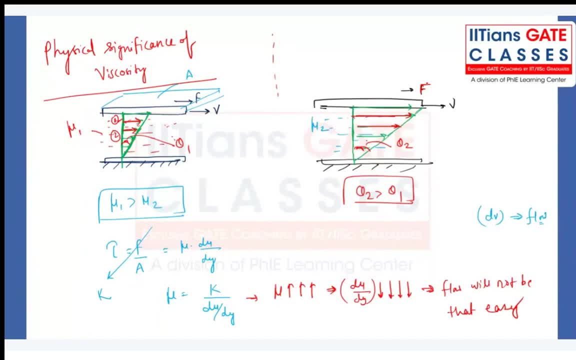 Then, sir, how Their momentum exchange is very, very high. There, the momentum exchange is very, very high. They will always colliding with each other molecules, Right, You know, for a given control volume. So what will happen? 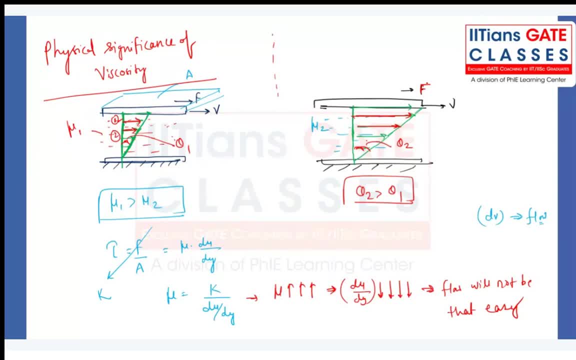 What will happen in that case? If the viscosity of the gases is low, a lot of momentum will not be exchanged, A lot of collision will not be there. If a lot of momentum exchange will not be there, how the fast-moving gas molecule will come to know that will be colliding with the low gas molecules, low velocity gas molecules. and if there will not be any collision between low velocity gas molecule and high velocity gas molecules, then how momentum will be transferred from the low to high 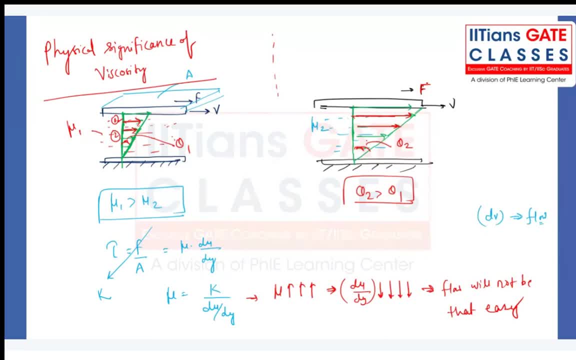 Right. So that's all about the physical significance of viscosity, Because you guys have not basically discussing that much about this. First, fluid statics and fluid properties. That's why I'm basically what Forcing too much onto this one, Because particularly fluid kinematics and fluid dynamics- onwards, you may be familiar with the topics. 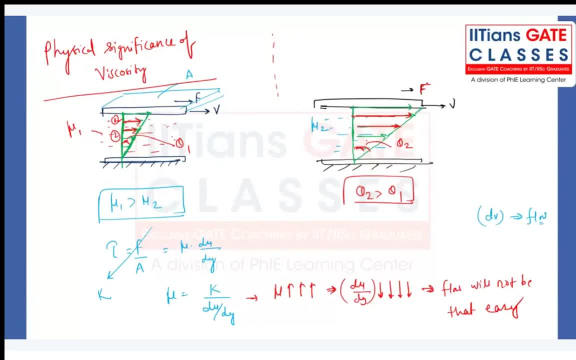 Right. Once it is done, let me know. So always remember the way I'm explaining you. You have to study In this manner for all the subjects, Even though it is taking time, until- unless you are not on See, remember whether it is a gas dynamics, whether it is any rocket science subject. 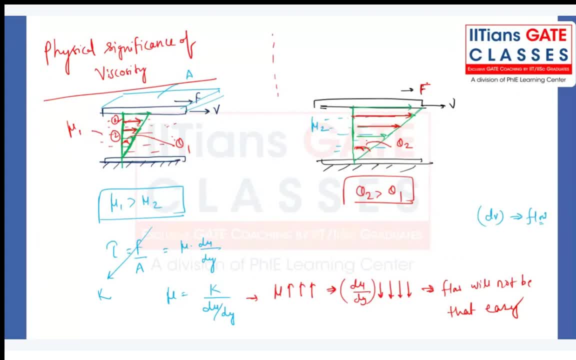 Always remember when you are not understanding each and every fundamental concept of that topic, Even though you try to solve the numerical of that topic. you may be very, very expert in that- solving the numerical- But the moment gate question will be coming and they will be testing a little bit of. 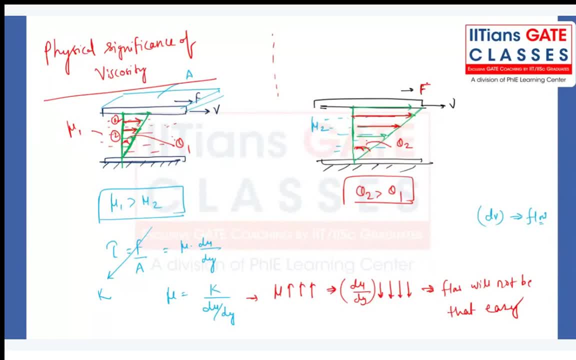 Theoretical understanding of that Numerical question will numerical You cannot solve Right. So we will try to see certain cases where theoretical understanding is important in solving numerical. also, It doesn't mean that you keep on doing the PhD in each and every topic and forget to solve the numerical. 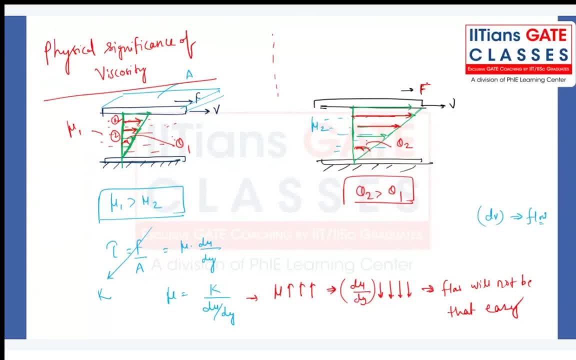 No, Following the numerical is our first priority, But with that first priority The precaution will be. we have to study very carefully each and every topic Right, And that is what the human being is given 24 hours of the time Right. 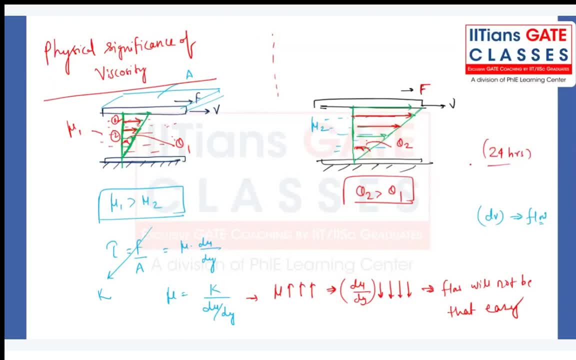 Initial days, when you start preparing for the gate, when you're not understanding any topic. you put some effort right, You just put some effort from here and OK, I'm not able to understand this topic. I will be putting at least 10 to 12 hours per day. 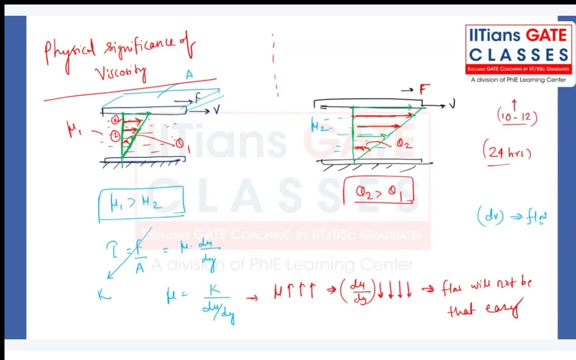 Believe me, after three months of time, even though you are putting six hours of time, or maybe Five to six hours of the time, daily basis, you will be achieving definitely a very decent rank, And you will not believe yourself that I got this particular rank irrespective of your score in BTEC. what you have scored, what you're scoring right now, it doesn't matter. 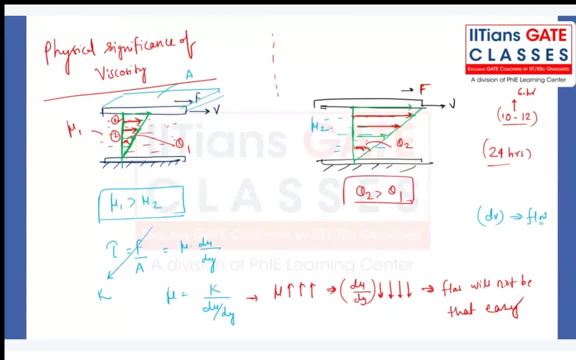 Gate examination is completely about the, what aptitude. you may be top of the, your university or maybe anything, but you may fail in gate exam. But a very, very poor candidate in the BTEC, He may top the gate exam. so that's that can happen. 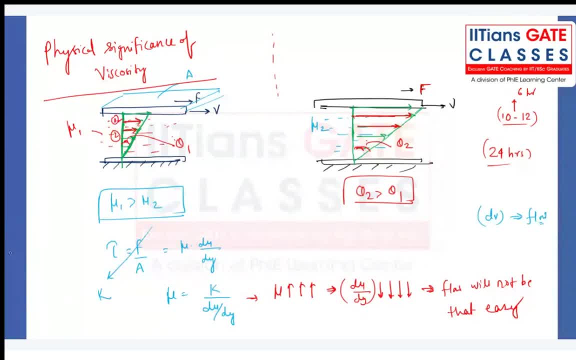 And remember one more mantra of gate examination: success right. Whatever the hard work you're putting, That will be proportional to results. If you're not getting results, don't blame your luck. So on the exam day, something, something happened. I couldn't apply the logic, I couldn't apply the things. 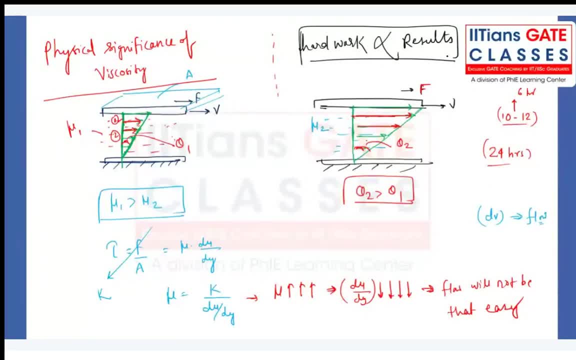 Maybe before one month. I was totally busy in studying only but couldn't practice much. All those excuses you should not give to yourself. Remember that whatever the hard work on the first day you are putting, remember it will be directly proportional to results. 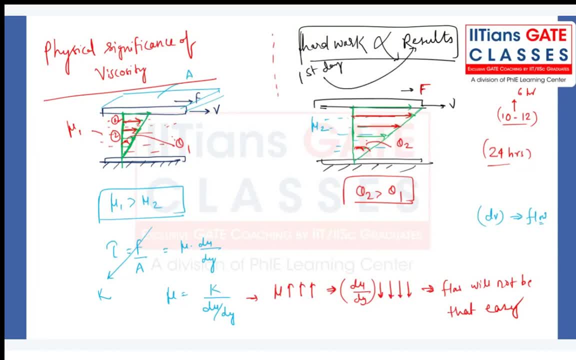 Each and every part will be contributing to getting a decent rank in actual gate examinations. Right now, is it done? all of you, All of you have noted down Why I'm motivating this thing, because at this particular age, maybe you might be having an age of 22 or 23.. 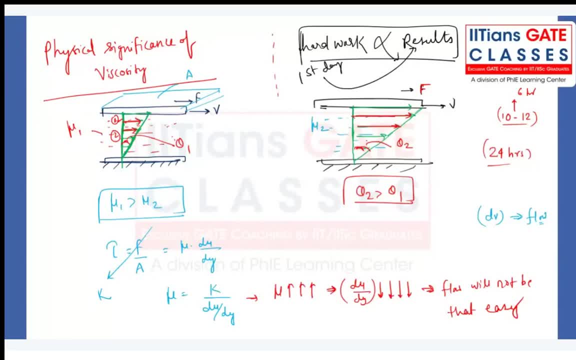 Your parents cannot motivate you right, They cannot tell you always, they cannot scold you all the time that you please study that, because now you have to understand yourself that it's your responsibility, that you have to work hard and get the. whatever the success and whatever the admission or maybe the placement after that. 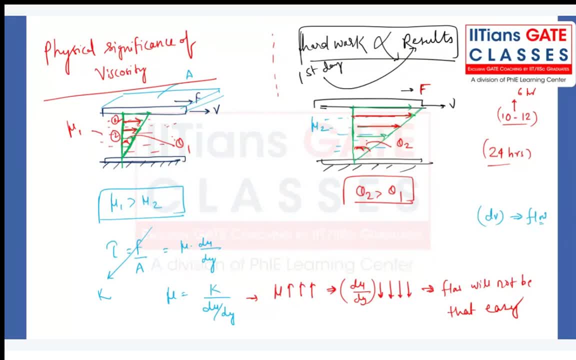 Right, Nobody at this age will say that you please continue, or basically what you study hard. or you just say that, whatever the, if you compare your ages, maybe you when you are in the 10th or 12th standard or maybe 8th standard. 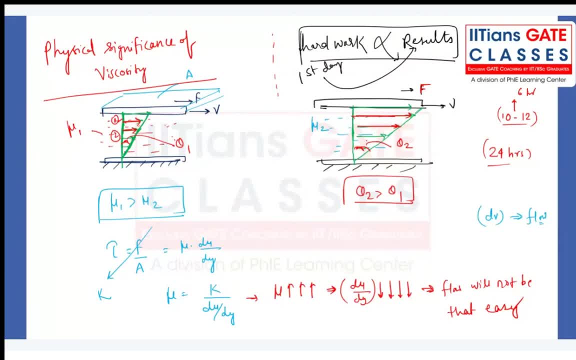 Right, There is someone who is there behind you who always guides you, But at this age, after passing basically what we take, nobody will be there to guide you, or nobody will be there to tell you that you please study. Self-motivation has to be there. 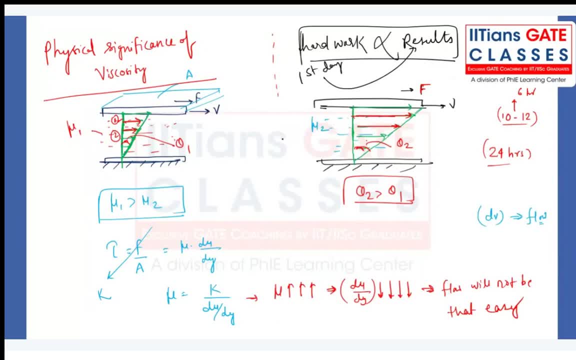 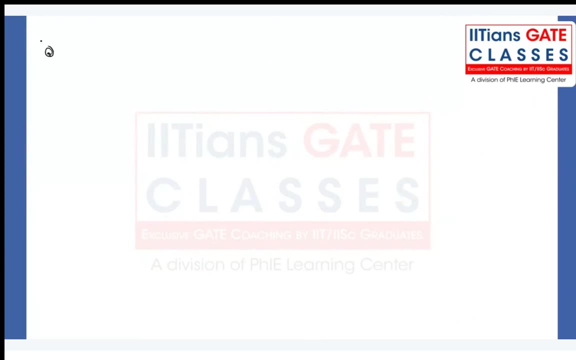 Now, regarding the other free body diagrams of the share, whatever the share stresses will be there that we have to discuss right Now. suppose, my dear friend, we have the plate note number one and we have the plate two, which is being fixed. 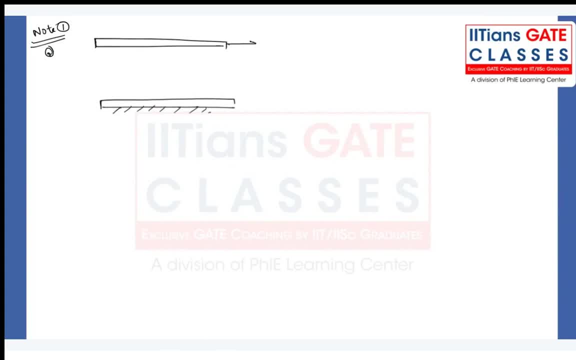 Now, in this case, my dear friend, we have the fluid which is being a static fluid. Remember, the fluid is not flowing. the fluid is what? Static fluid? The fluid is only flowing because plate is flowing. the top plate is what? 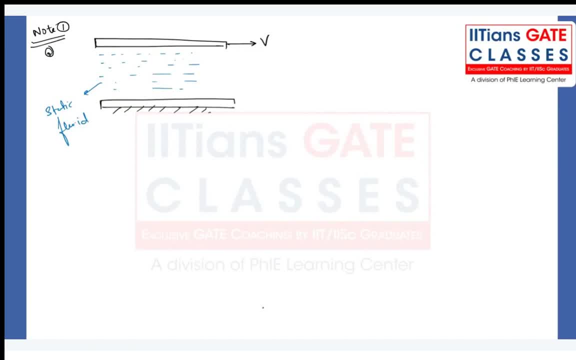 Flowing. That condition we call simple cuvette flow. Right, When the fluid is not flowing on its own Right, Where the pressure gradient is zero. that's what we call simple cuvette flow. But we have certain conditions or certain cases where not only the plate is providing a driving force for the fluid to flow, but we do have the flowing fluid also. 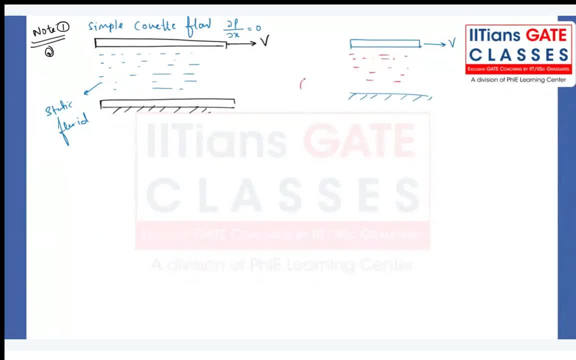 Maybe we have just provided some kind of pump where the fluid is continuously pumping and dou p by dou x is not equal to zero. So there's two things are there. which is driving? First is the pressure force: The pressure force, which is a driving force, and the plate force, or whatever the plate velocity, that is also a driving force. 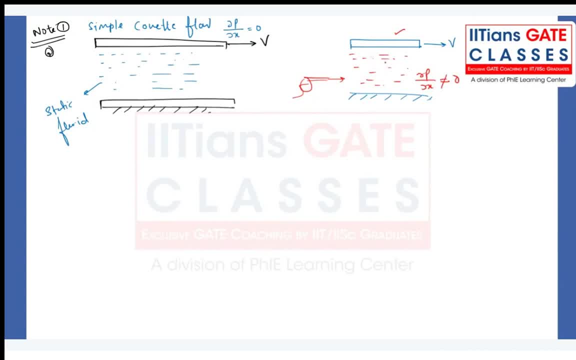 So definitely here the fluid velocity will be higher than this case. Again, we will discuss in Leibniz flow in different cases now. So here I want to talk about certain conditions. Let's say the fluid velocity will be having a velocity profile. 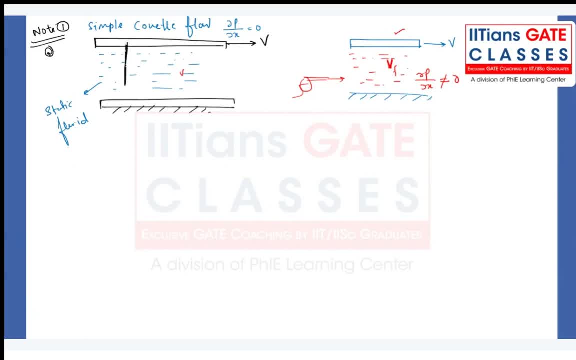 We have something like this: We have the velocity profile like a parabola, And what you will observe here that in case of velocity profile, which is being parabola, at a narrow distance from the wall narrow region, when you focus your attention within the very, very small distance from the wall, 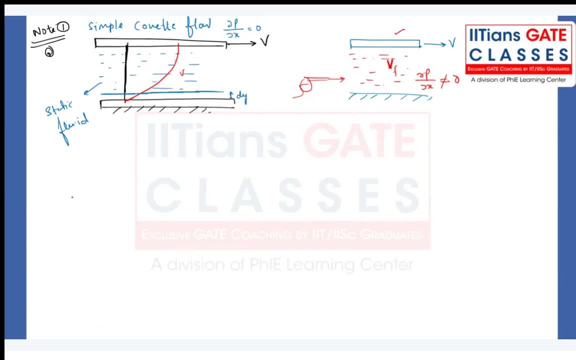 in a dy distance, what you are observing, any variation. you will say: so, this is a parabola or something like that. you will feel that it is a linear variations. You will feel that this will be A linear variation. You cannot see any variations, right. 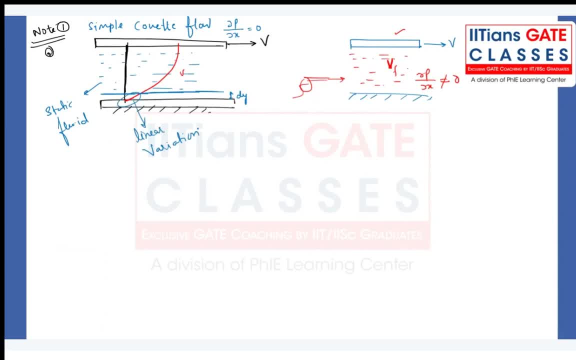 That is a linear variations. So put a note, note number one: For a very, very small gap, For a very, very small Gap, The velocity profile can be assumed as A linear one. Or maybe, in case of velocity profile is not given, you can assume it as a linear velocity profile. 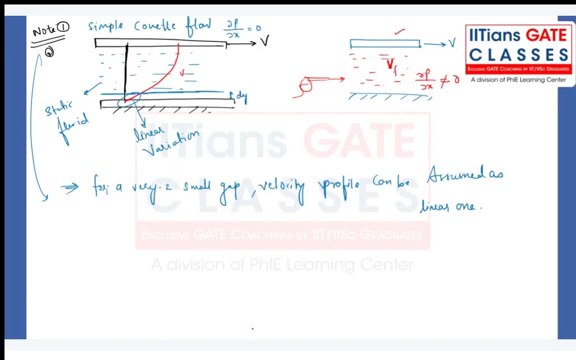 Make a note of it. Once it is done, let me know Where is that Simple cuvette flow? What is the meaning of cuvette flow? The fluid which is being flowing in between the two plates in which one plate is fixed and other plate is moving. 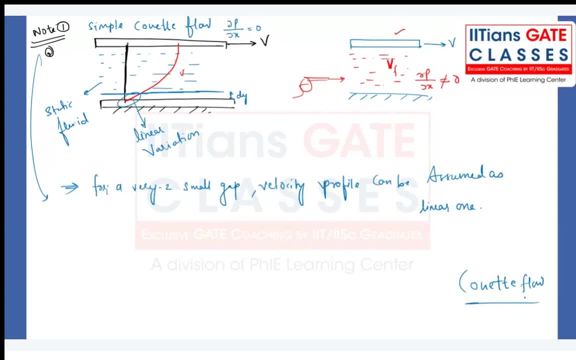 with some constant velocity. that flow condition will be called as cuvette flow. Right Now, can I move to the next one? Note number two. All of you have noted down. Can I move to the next one? All of you have noted down. 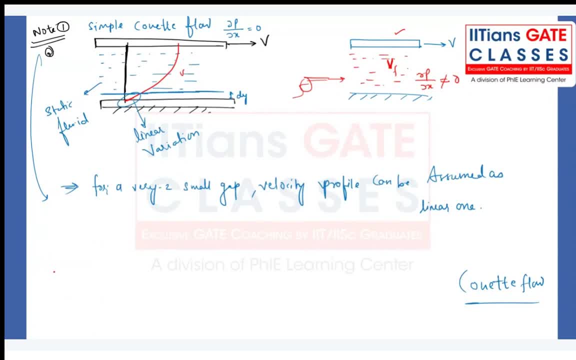 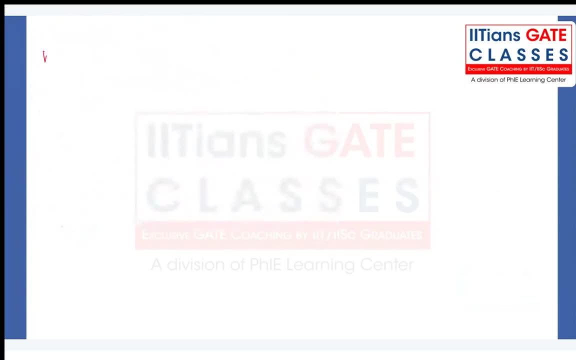 Done. Is it done Now? so here we will try to make a note number two. Note number two: it has Something like this: We have the plate. We have the plate, my dear friend, And we have the fixed plate, like this, where the fluid is flowing. 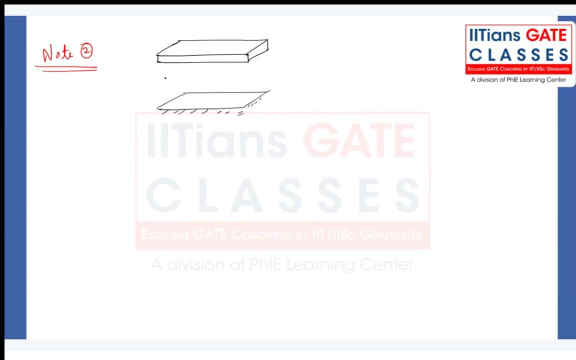 Yeah, we can say the fluid element is placed like this. I'm assuming the fluid element, There is a two plate. There is a fluid element right Now I'm asking you that it is being applied with the force F and it is being zero velocity, zero fixed plate. 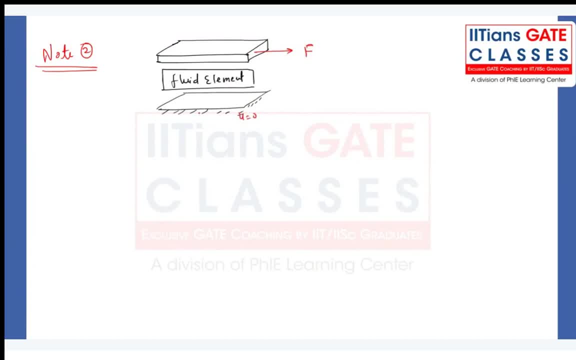 So here you will have to draw the direction of the plate, Draw the direction of, Draw the direction of the share pose On top plate, Bottom plate And What you say. So here I'm giving you the option. let me give you the option, option A: 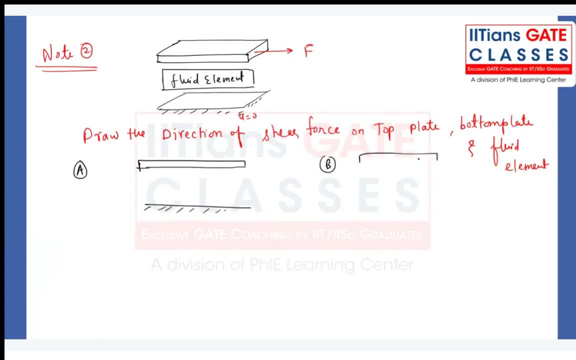 Let me first draw the option. None of the above, so let me first draw it. The variation of the basically what? the shear force, that is, the resistive force offered by the fluid element, which is having the viscosity Fluid element here, once again, fluid element. once again, we do have fluid element and we 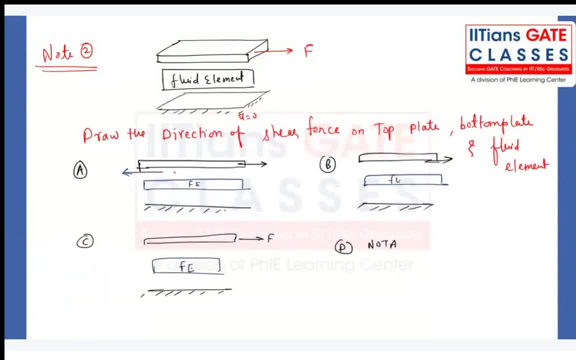 can show here by shear force, shear force F. We do have the force F here. Let me just write it by F1, F1, F1.. I'm assuming the linear velocity profile, linear velocity profile, right, Because see in the linear velocity profile my different. 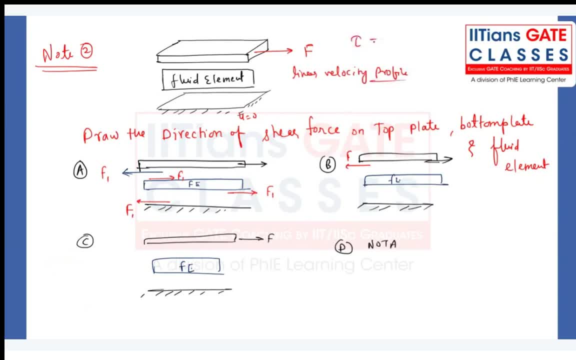 What about the shear stress? Mu du by dy. This is a slope right. Du by dy will be what? What about du by dy? That is the velocity gradient. Velocity gradient for all the fluid layer will be same. This will be same. 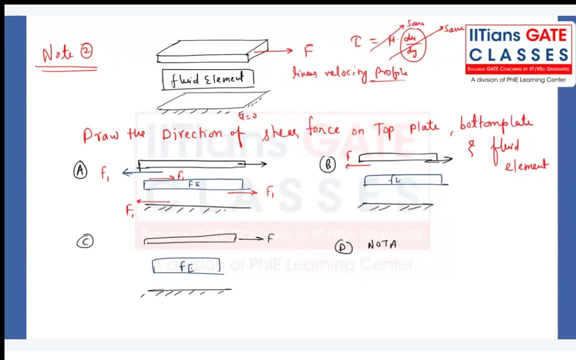 This will be same For all the layers. shear stress will be same area is same, shear force will also be same. So in that respect, I have assumed this one, This one will be F1.. And then we do have- yes, we have this- F1, F1. 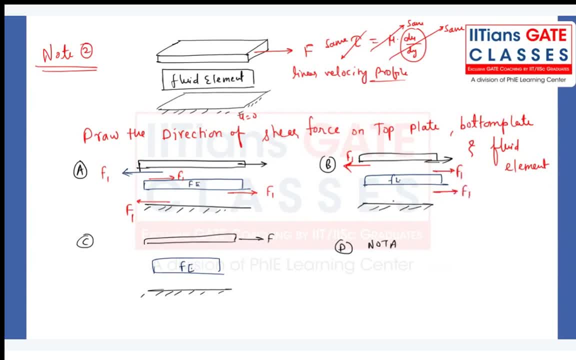 Now just check it out. Okay, let me just do here, Because in this matter, for each other it is F1, F1, F1.. Yes, So, yes, it will be F1 or F2.. No, It's that same. 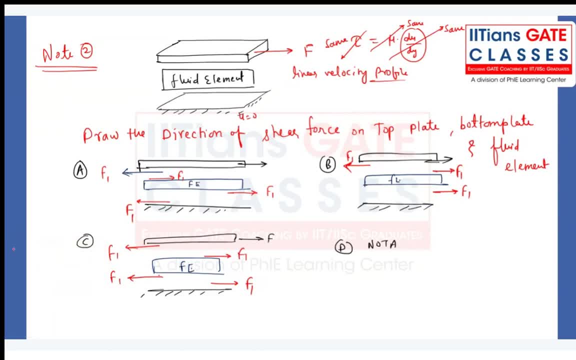 Let me just go back here. Make sure I do on the chart, make sure that F1, F1 and F2 will go down. That's it. I think F1 will go down Here. it is here, That's it. 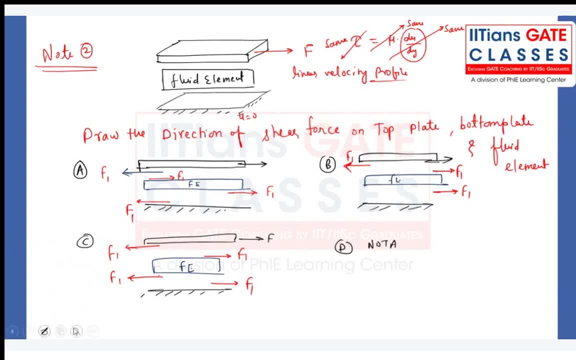 See, it will go down. Yes, Yes, Yes, indeed, That's it. So, yes, Two pi, Thats it, That's it Good, Good. So let me do this, Let me do that Well. 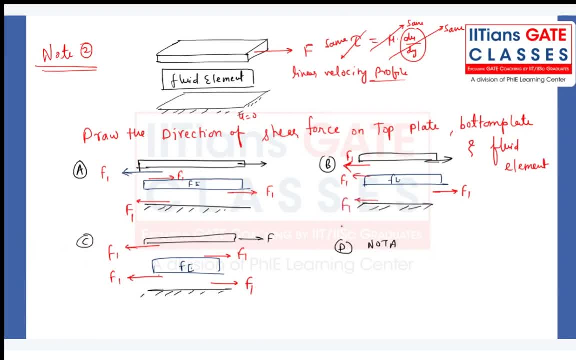 So next, let me just do it for us. So correct option is C right. So it always try to resist the what, The relative motions, How it will try to resist, See, because the top plate is moving in which direction In. 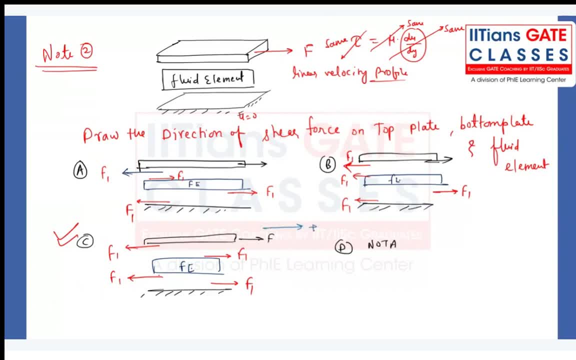 the positive x direction, right. So the fluid layer, fluid element: what the communication will happen. What the communication will happen. The fluid layer which is trying to stick with the top plate and the fluid layer which is there. what the communication will happen. 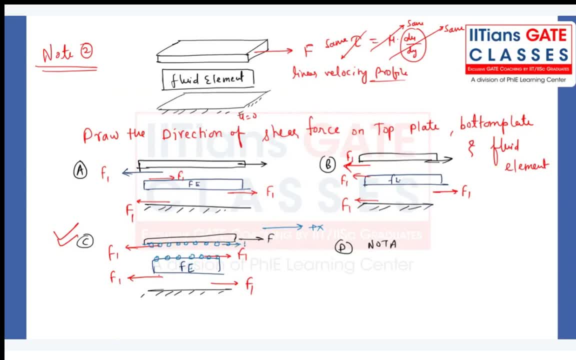 They are trying to move in with some higher velocity, the fluid element will say: you come back and they will offer some kind of resistive force. They will try to oppose the motion and they will apply the safe force in the direction of, in the opposite direction of. 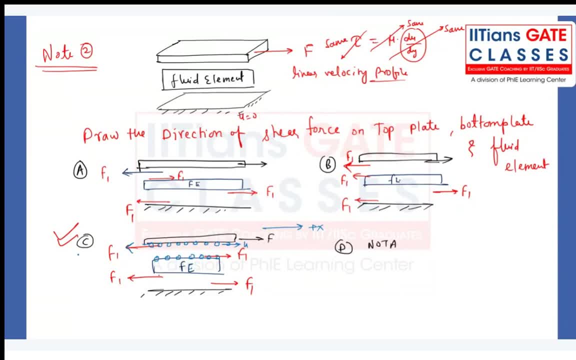 motion. So what the Newton's third law will say? It will apply some same amount of safe force in the opposite directions. Now what the fluid element will say After application of the F1 pose, this one, the fluid will say: you come back and they will try to move in. 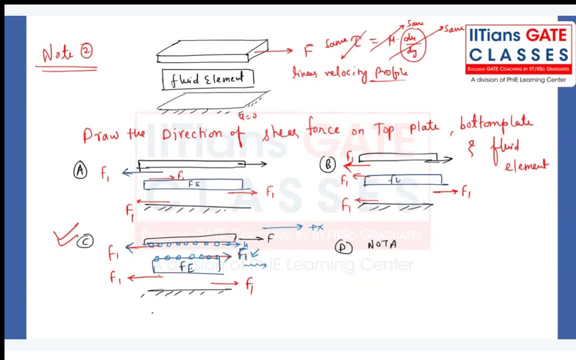 this direction- positive x direction- What the plate will say: Hello, come back. And by the Newton's third law, the fluid element will offer some kind of force, viscous force or safe force in this direction onto the fixed plate. Make a note of it. 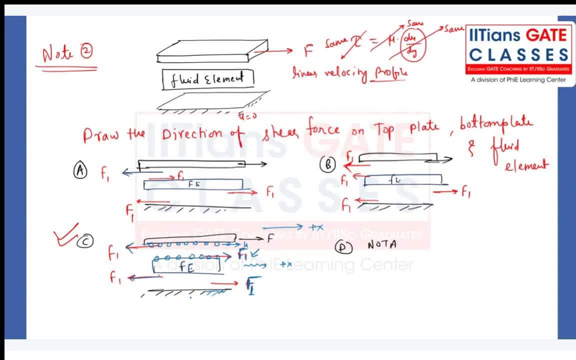 So remember, viscosity will always resist the relative motion, not absolute motion. Fluid element means there was a fluid right, But I have assumed it as a complete fluid element. Maybe the fluid particles which is being attached with this one. they will be. 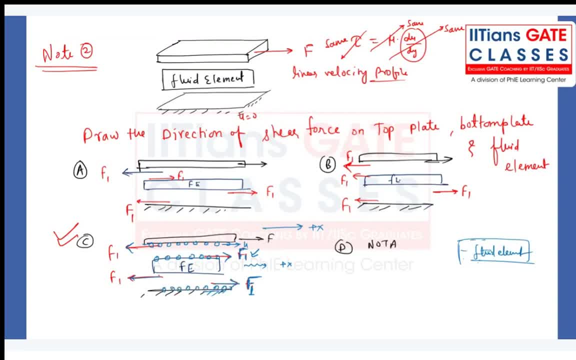 applied F1, pose onto them. Now all of you have noted down. Can I move to the next one? Now all of you have noted down Some question we will do. Now, my dear friend, when you try to see, we have lot many questions We will discuss. 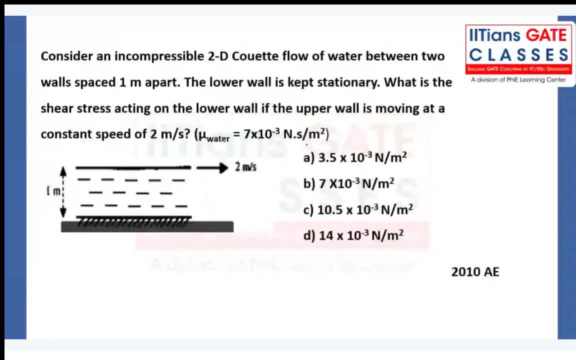 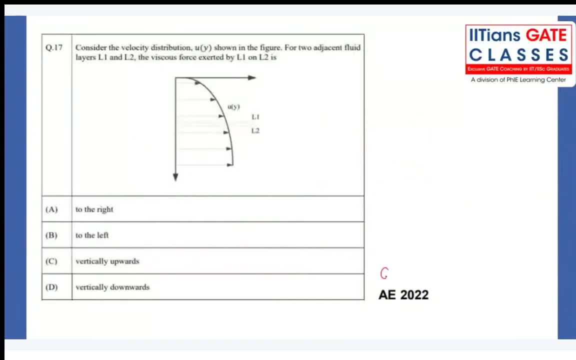 one by one. Yeah, So when you see the gate 22, aerospace paper, we have this question of one mark. Consider the velocity profile. Maybe the velocity profile. they have reversed it. That means the top plate is being fixed one and the bottom plate is start moving in these directions. 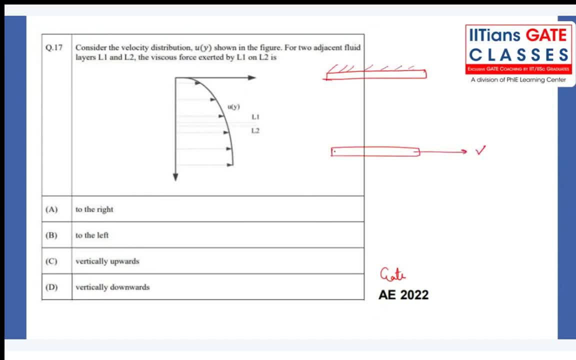 right, We will discuss the two fluid combinations you know. Now, here my dear friend, tell me what could be the answer. Whatever the particle velocity is there, they will try to move right And they are basically forming like this: 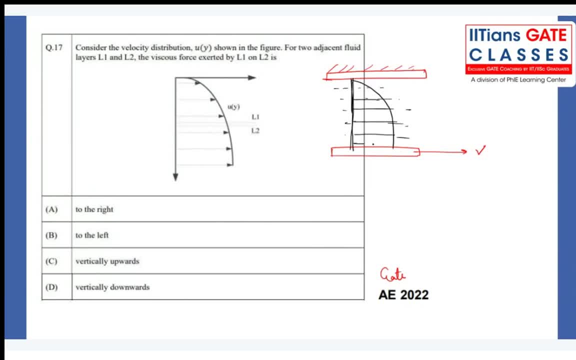 What you are understanding from this segment. you are completely understanding one thing. that one thing is sure, sure, guarantee, is there that, my dear friend, whatever the fluid particle, is there, this L2 layer having the more velocity than L1 layer, right, Right. 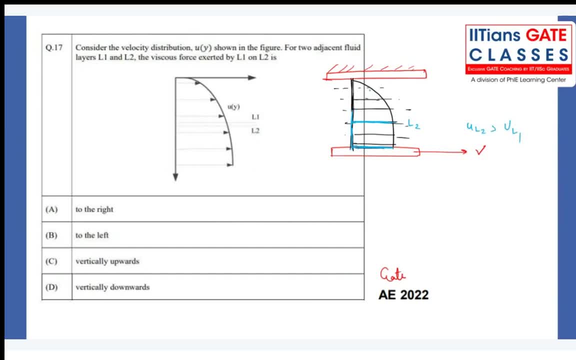 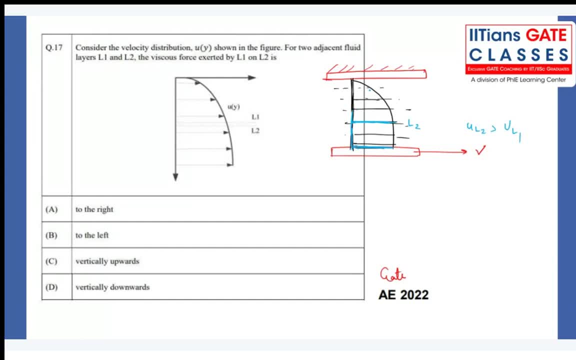 Of layer 0?? Right, Right, and that cannot be the question, right, Right, But this is: if you could apply it from any dimension Of layer 2? Of layer 0? Ok, but if there is something like that over here that your. 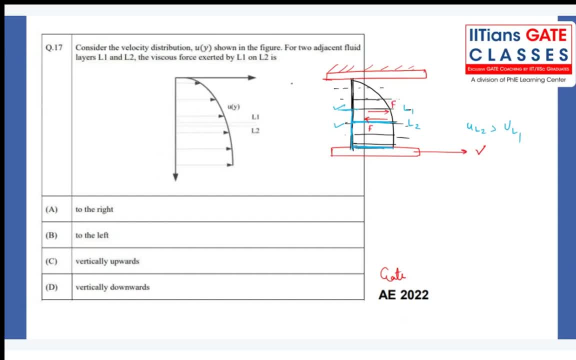 body is moving in the grid by L1 onto the L2 to the left. getting my point? So this is small, small discussion by different those who are not very strong in BTech. they have done the fluid mechanics or aerodynamics in a very light manner and if you are not, 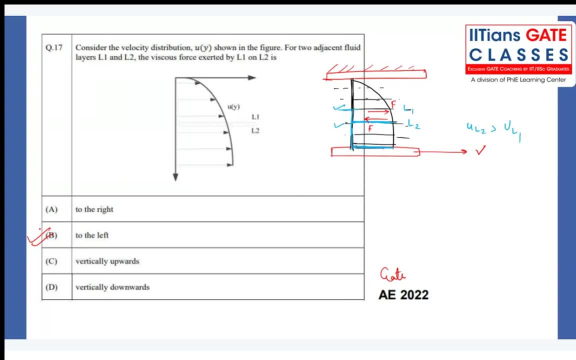 be getting the support from external, from the coaching institute, then how can you attack this question, right? So try understanding If this question can be easily attacked by the normal candidates. also, if you know the fundamental concept of engineering mechanics, like what the behavior of the coefficient, 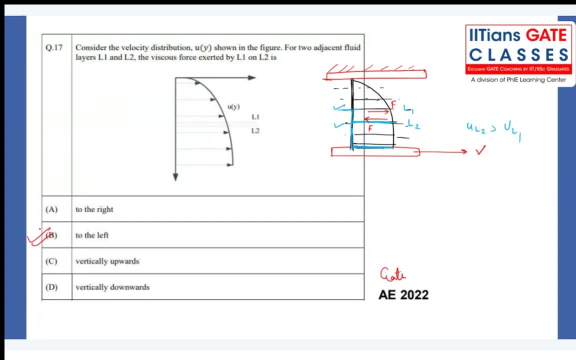 of friction there, force of friction. same phenomena is happening over here also in case of viscosity. They have just reversed the what the condition we are discussing right now, you know. We have just reversed the what the condition we are discussing right now, you know. 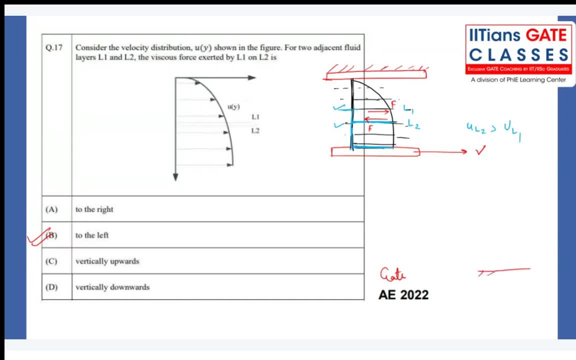 We are discussing the bottom one is fixed one and the top plate is moving. They have changed it And that is what they want: to test it in a particular three minutes of duration for particular question that has been allotted. Is it done? all of you? 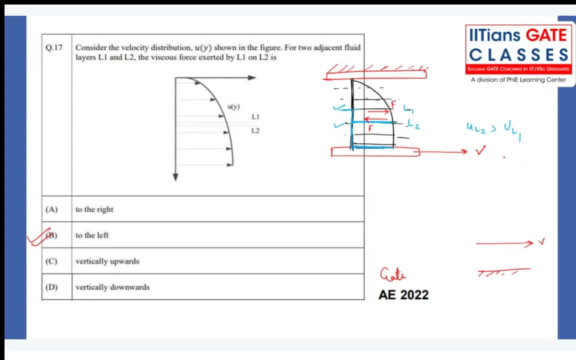 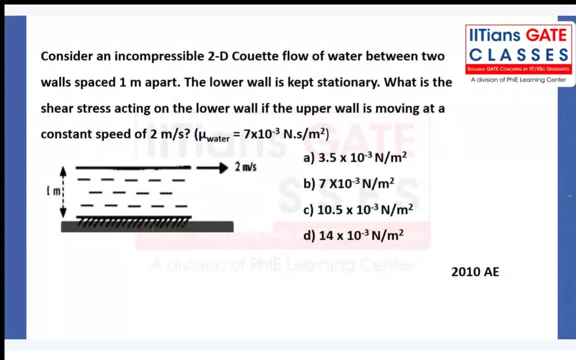 Can I move to the next segment? Next question: Perfect. So here, when you see a very simple question This question has been asking A to the 10, A Consider an incompressible 2D cuvette flow right, So which is one plate is fixed, one and other plate is moving with some velocity, my dear. 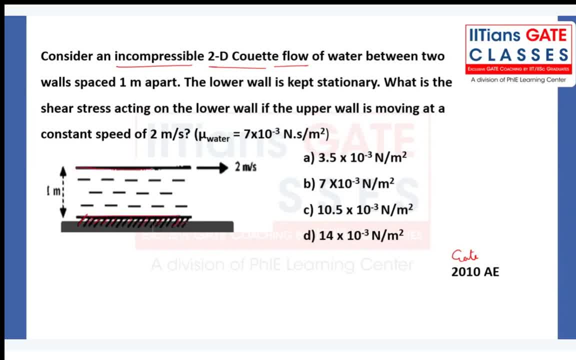 friend And you are observing that the plate is also moving with some velocity: 2 meter per second, And the space between the plate is 1 meter apart. The lower plate is kept stationary. What about the stress? Okay, So what is the stress on the lower plate? if the upper plate is upper wall is moving with. 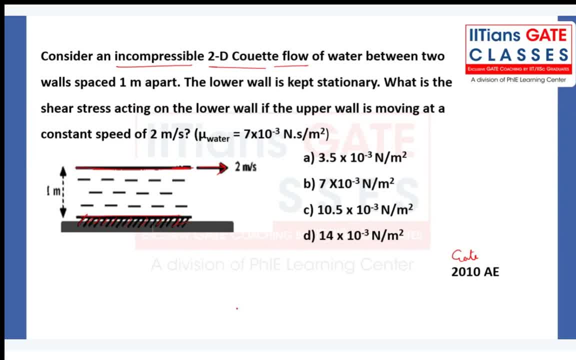 some constant velocity. So, my dear friend, what you are understanding from here? that we have to apply the Newton's law of viscosity, because water is a Newtonian fluid And Newtonian fluid will follow Newton's law of viscosity And there is no velocity profile. 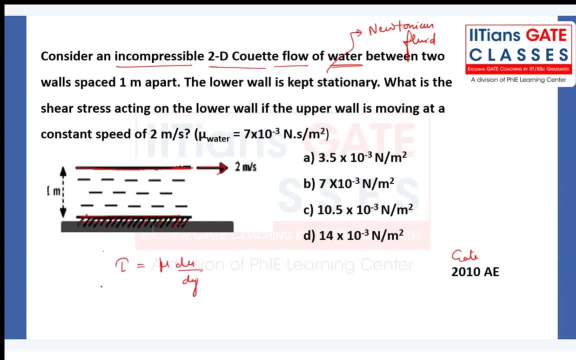 When there is no velocity profile, we can assume it as we can assume it as what? Linear one. But there is a proper reason why we are assuming that to be a linear one, right? I will give you that reason, so that you will be surprised to see that that is not the assumptions. 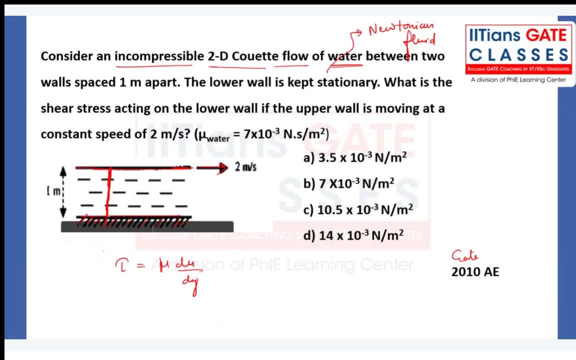 that is being indirectly we are getting from the equation Navier-Stokes equation. This is what we have, the linear velocity profile, And when it is a linear velocity profile, we will assume that it is a linear velocity profile, And when it is a linear velocity profile, we will assume that it is a linear velocity. 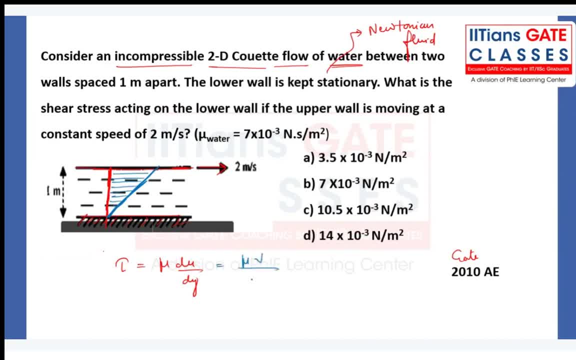 profile. So the velocity profile will be getting like this: Share stress will be: and for linear velocity profile, what is the share stress distribution, my dear friend? The share stress distribution will be something like this: That will be uniform. Again, you do not draw the backward arrow, you simply draw it. the distribution that 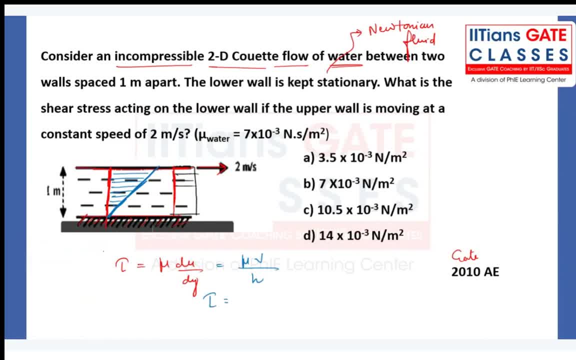 simply showing the at all the fluid layer, the share stress will be same. Right now, 7 into 10 power minus 3. velocity is what 2, h is what 1. so 14 into 10 power minus 3. newton per meter square. if the same question, if i would be asking: 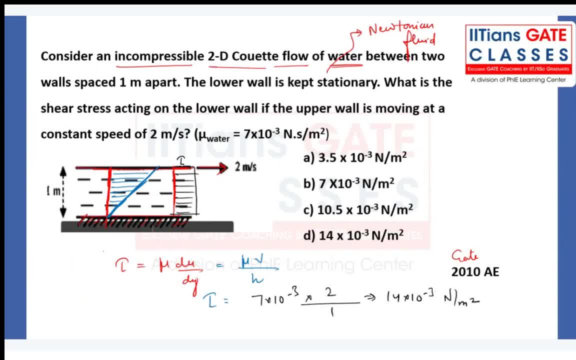 what about the shear stress onto the upper wall? what your answer? they have asked the shear stress on the lower wall right. what is the shear stress? the next question: what is the shear stress onto the upper plate, upper wall? same answer will be there. same answer will be there because v is constant, h is constant, mu is constant, nothing is varying. 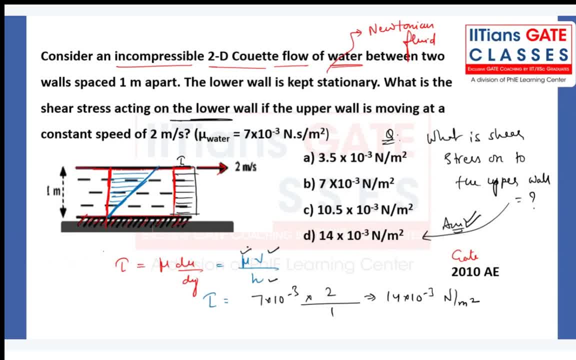 right now coming to over here, sir, i am not understanding why you have assumed linear velocity profile, even though gap is reduced reasonably. not a very small gap, one meter gap. is there linear velocity profile? now for that let me discuss. uh navier stokes equation, in fact, uh, very hard to say right now. 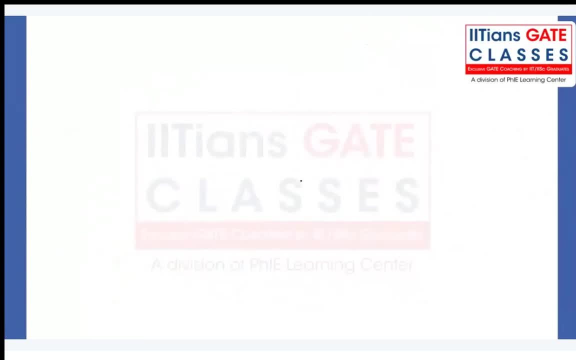 if i discuss- that is a very injustice to all of you- that, sir, you have not covered the navier stokes equations. we have not covered till now the momentum equation. but you are talking about that, but, believe me, without that there is a, there will not be any feeling about that. 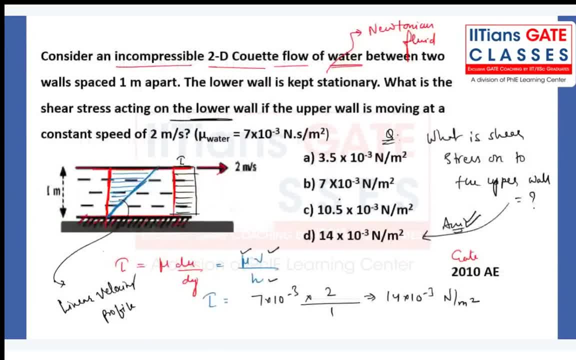 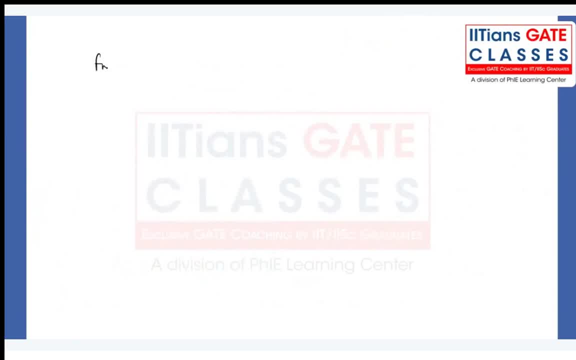 simple you. I have a straight forward, two mark question. right, a lot of understanding is there now. so when we write net force that is equal to mass into acceleration, so when i will derive that navier stokes equation, obviously i will be considering the viscous force and the body. 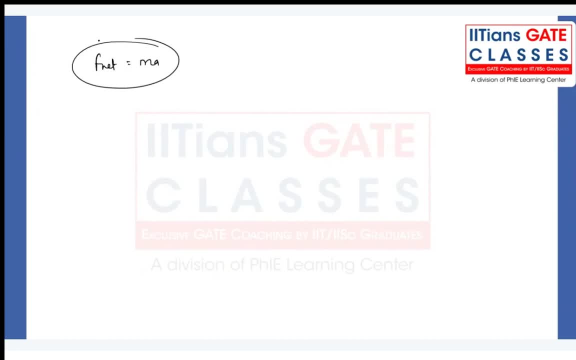 force right now here, and the pressure force. so in all, if i write the x momentum equation in all together, if i write x momentum equation, my dear friend, what i will be getting? the x momentum equation, uh, acceleration, will be u into dou u by dou x, v into dou u by dou y. don't worry at all. 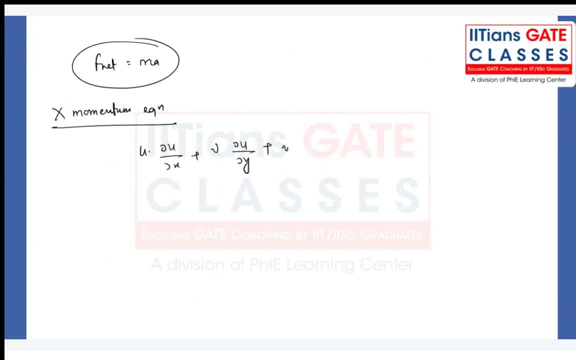 those who are not getting, it's absolutely fine minus one upon rho dou p by dou x plus mu by rho dou square u by dou x square plus dou square u by dou y square. now you try understanding my different in this segment. velocity u is there right and velocity u is a function of y. for example, velocity u is a function of y in this. 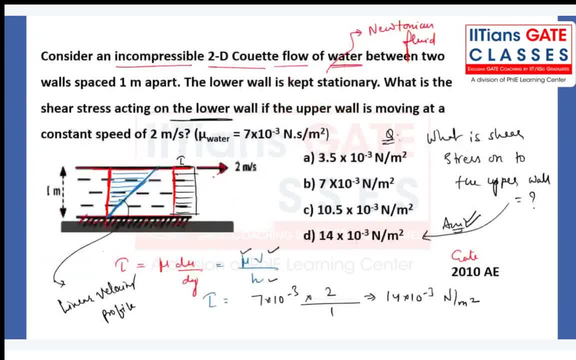 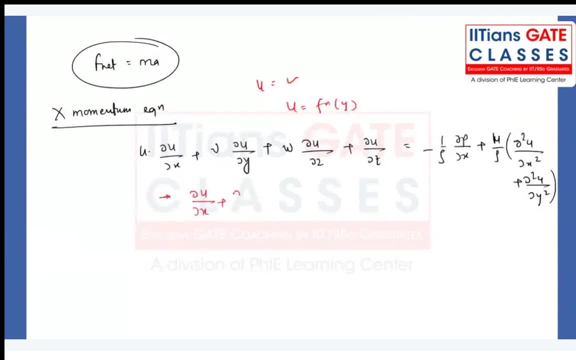 particular equation right now, even though they have mentioned 2d, flow right from the continuity equation. dou u by dou x plus dou u by dou y, that is equal to 0, being the velocity is only the function of y. dou u by dou x will be 0 velocity. dou u by dou y: see, this is a? u component v. 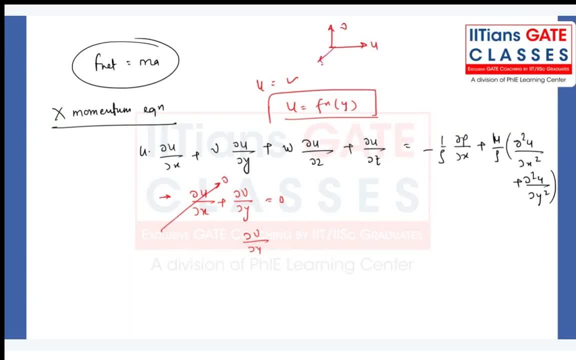 component omega component right. this will be 0. that means v is a function of x and z, but we know that the fluid cannot penetrate. there is no hole in that plate right. so this will be 0. dou u by dou x will be 0. third component of velocity will also be 0. we are assuming steady flow. 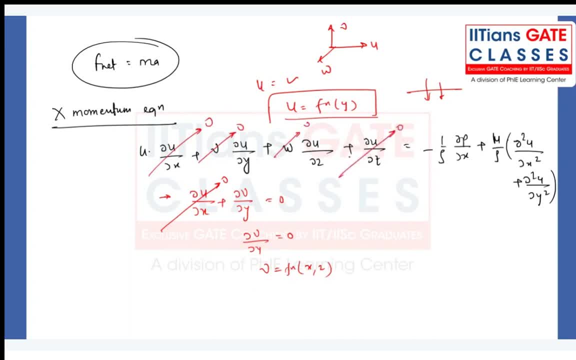 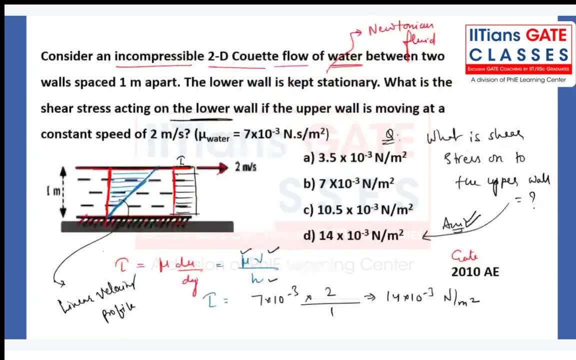 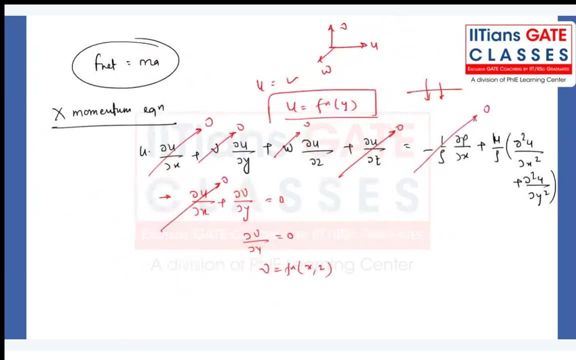 steady, incompressible flow, right, density is being constant, right, uh. and in that case we are assuming simple cuvette flow, right, simple cuvette flow. we are being uh talking about. so what will be there? dou p by dou x will also be 0. now, what about this? dou square u by. 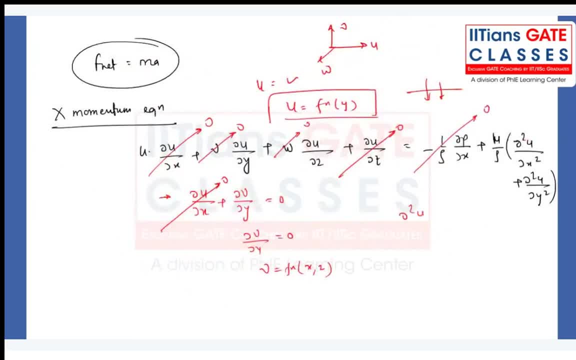 dou x, square, right. this term you can approximate as u. infinity x is nothing but length of the plate. length of the plate right, x you can when you do the dimensional analysis and similarity. one term, one topic i will discuss right, uh, order of magnitude analysis. there i will be treating x. 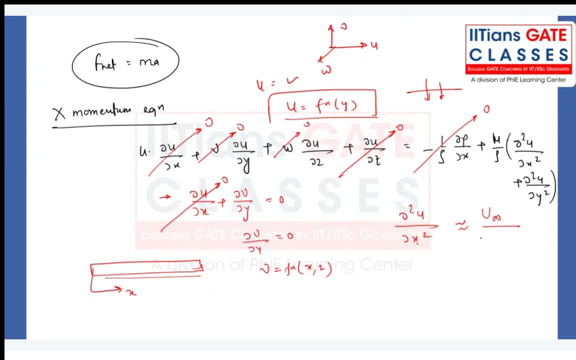 what is the maximum order of magnitude for x, l square right, as compared to boundary layer formation delta? this l length of the plate delta l, delta by l, is very, very low, very, very less than 1. so if l is very, very high, this term will be negligible once again. that term will also be 0. 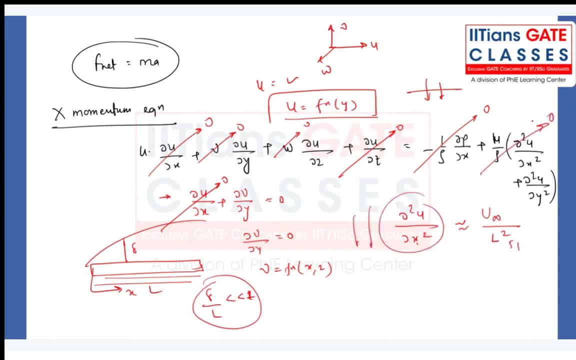 So only you will be left with this one dou square: u by dou y square that is equal to 0.. When you integrate it and when you further integrate it and you only tell me whether velocity is a function of linear variation of y or not, 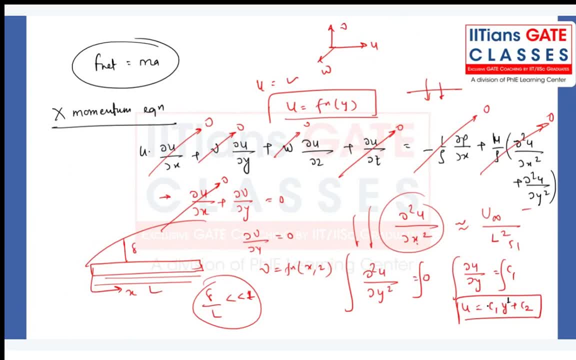 Once we will discuss the Navier-Stokes equation, you will not be having a penny of doubt. But for the time being, for proving that I am just doing this thing: Correct: Upper fluid and upper plate. they will be having fluid which is being contracted right. 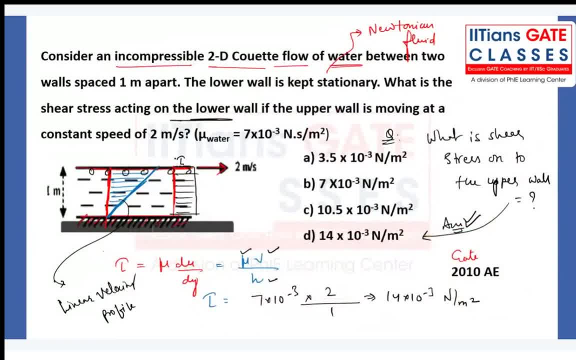 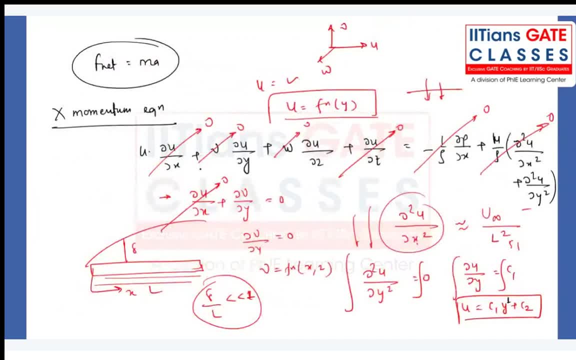 They will be having no slip condition. being satisfied. Getting my point Is still my different. Some of you might be thinking, sir, why the hell we are calling that to be a 2D flow? I will be discussing in the fluid kinematics types of fluid flow, my different. 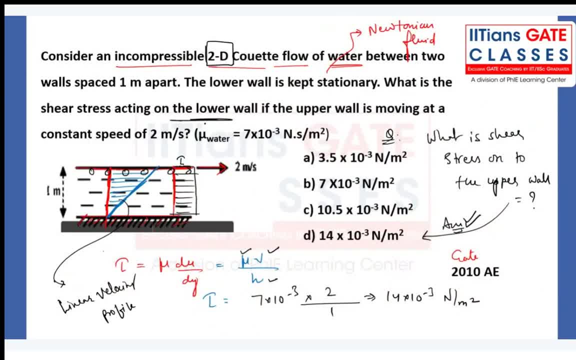 There you will come to know the importance of that. No, So in the upper plate the relative velocity is 0. Then with respect to the upper fluid, then the relative velocity is 0. No See on that fluid whatever. 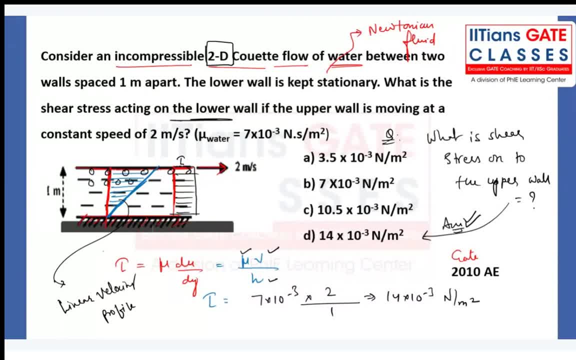 The below fluid is there, they will offer some kind of resistance force. right Adjacent fluid layers, they will offer same kind of force. F, Whatever the force I will be getting tau into area right, That will be having the same force in each and every layer. 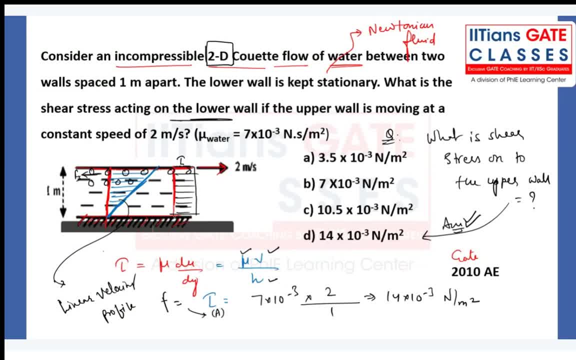 Getting my point. This force of friction will be force of resistive force, will be same in each and every layer. Getting my point? Is it done? all of you? Can I move to the next one Or we can close it. Next particular thing we will discuss right. 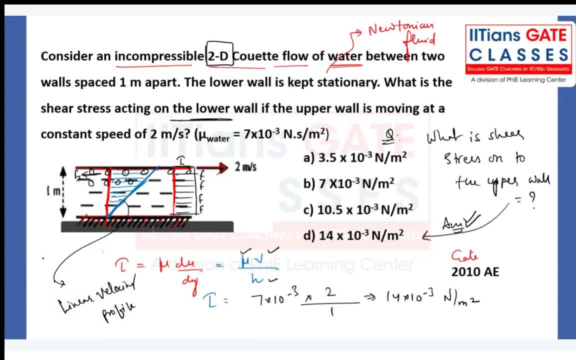 In further classes. Thank you all. right, So we will try to finish more questions, right? In fact, you will see in one gate paper, right? You try to solve this question as a homework, right, All of you? 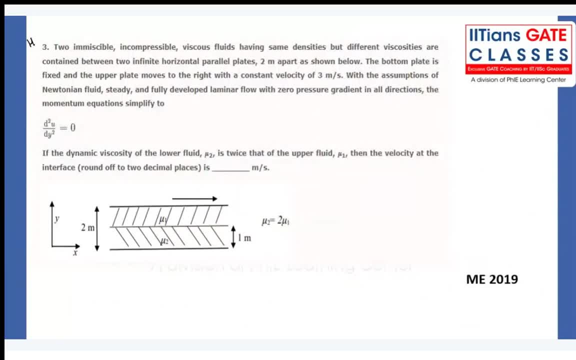 You please try to solve this question as a homework. This is mechanical 2019.. Where two fluids are there in that right? One plate is fixed, one Upper plate is moving. They have given the relationship between the velocity viscosity right. 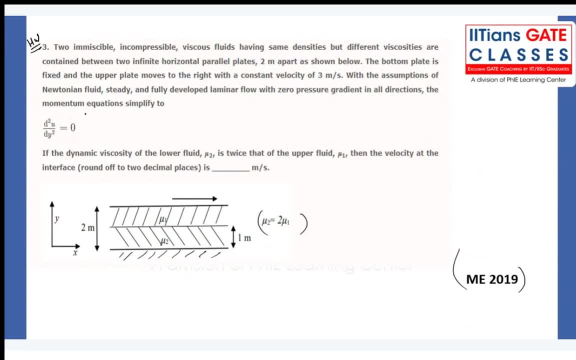 And they have given the equation also. See that That means linear velocity profile And how it is coming. I have shown you the proof of that from the Navier-Stokes equations And still I am agree with the fact that right. 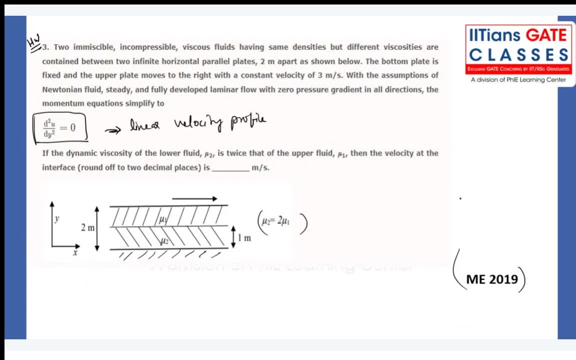 So we will try to solve this question as a homework. I have shown you the fact that right. I have shown you the fact that right. Some of you will be thinking, sir, 1D flow is there, But in the question they have mentioned 2D flow. 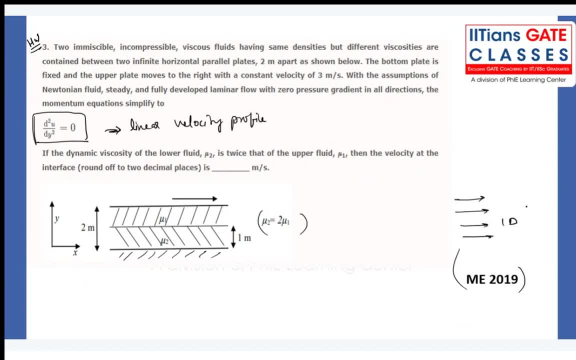 In a fluid mechanics, the flu 2D flow. 1D flow is not defined by the coordinates, Whether fluid is flowing in X coordinate, Y coordinate, Z coordinate. Even though it is flowing in a one direction, still it can be 2D flow. 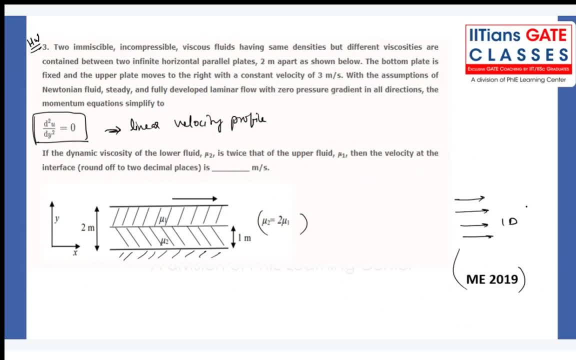 I will be discussing in the types of fluid flow in a fluid kinematics right. Thank you, Sir. Excuse me, sir, hello, so right now, what you are understanding. language of the question is also very important. you try to understand each and every line of that incompressible viscous fluid. 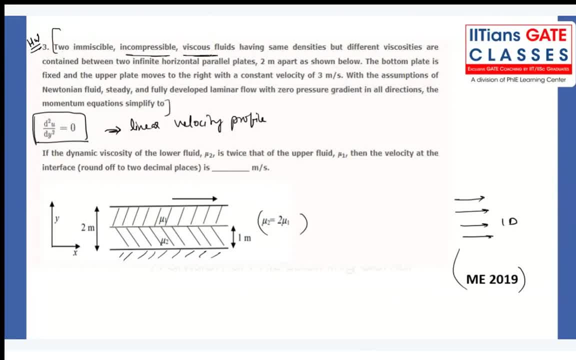 viscosity is there, incompressible density is constant, because who knows that with density they will give some function of time. then what you will do? right, we have to be careful with each and every terms, right, sir? now all of you, hello, hello sir. if it is done, we can leave for the day. 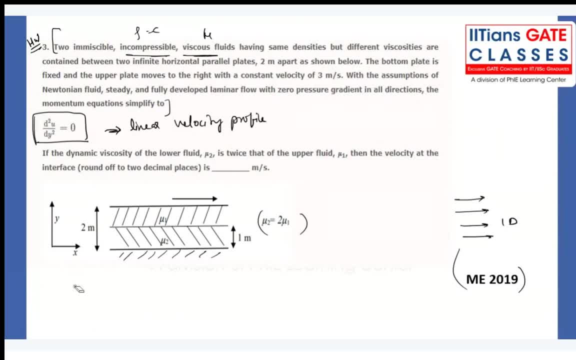 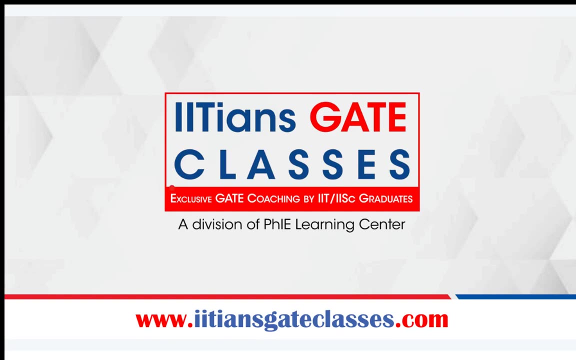 done. yes, yeah, please, quickly, like you, infinity. yes, that is strike with the plate. uh, we are assuming a good flow. if the force is same, then how the velocity will be different for different, different layers. yeah, obviously, card is there, so sell me for the day. okay, sir, okay.